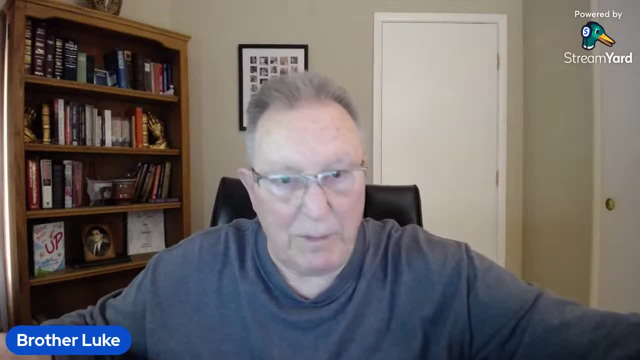 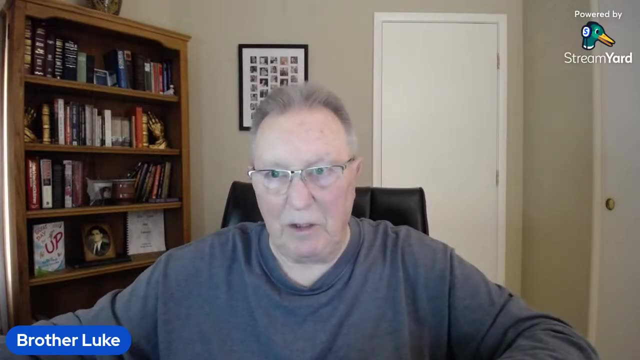 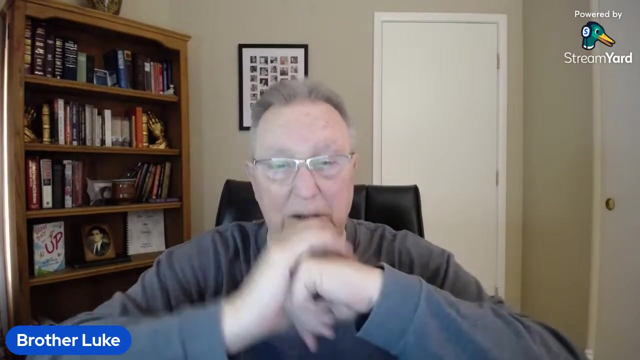 got my cough medicine, got my antibiotics. I've been taking a lot of medication, but it's persisting. It may be what Brother Tom is talking about in the chat room. Maybe we have the same thing, I don't know. Mine's not related to acid reflux, though, but mine's irritated throat congestion in the chest. 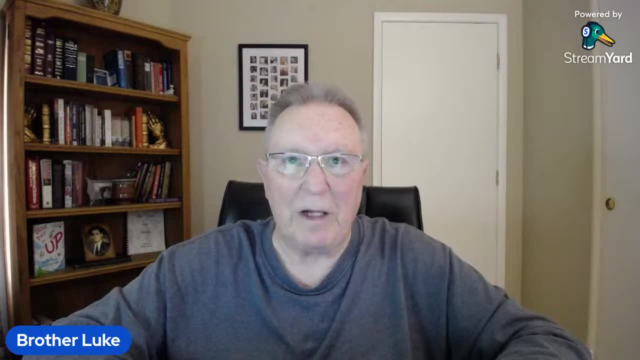 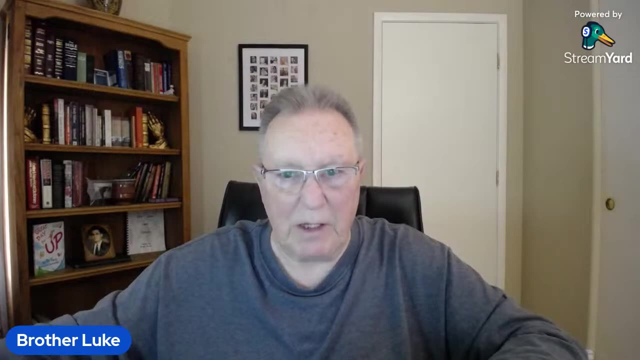 It's not severe, but it just doesn't want to go away. It will, So I guess let's start off the prayer. Prayer requests: praying for Brother Tom for his healing, and also for me too, And anybody else who has any prayer requests, put them in the chat room. 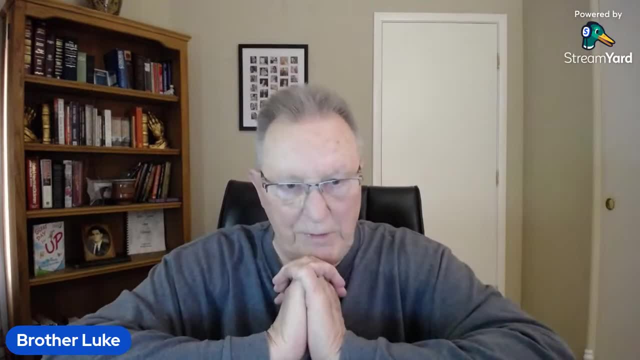 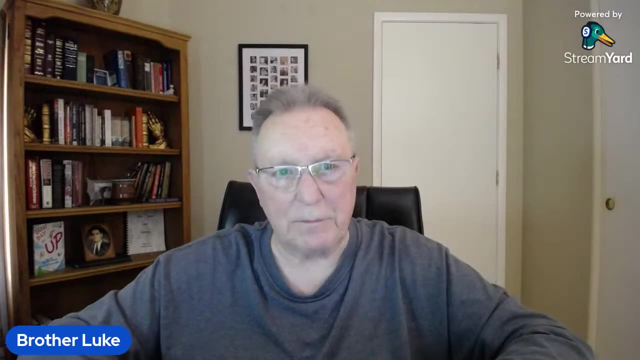 and I'll put them on the screen so that we can all pray for each other. All right, Normally our program goes for about two hours, but that's when Renee's here and we're talking about, you know, 50-50.. 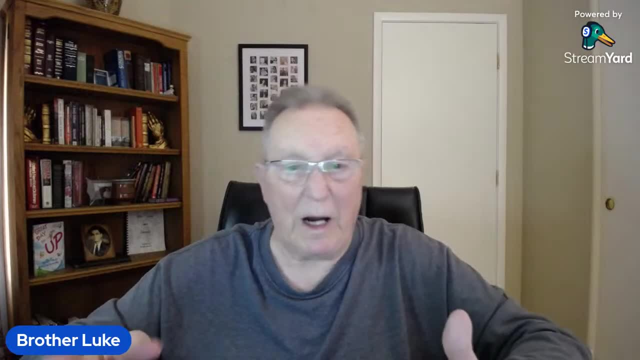 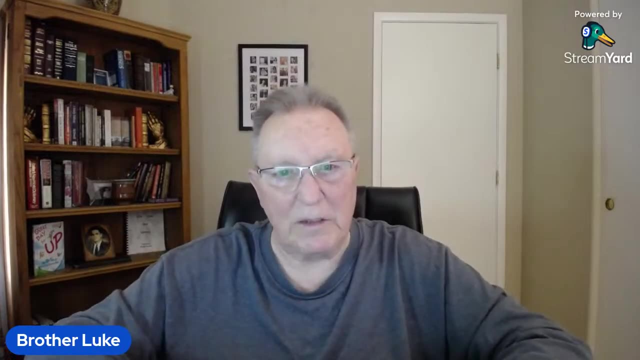 So I'm not talking for two hours, I'm talking for one hour or less, And even when I'm healthy, talking too long weakens my throat. I'm not sure how long I'll make it, but I'll go as long as I can and see how long I last here. 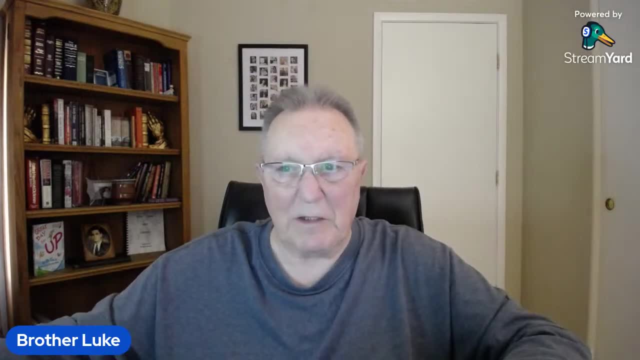 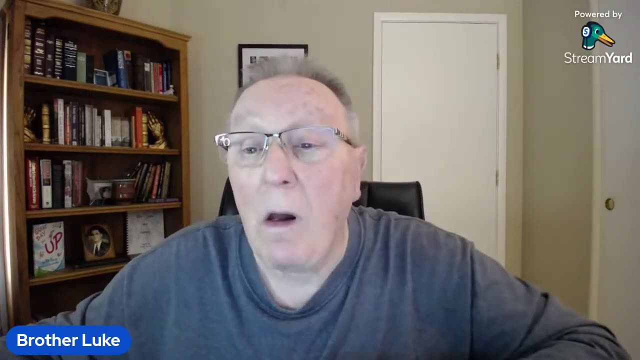 But let me start off by just saying hello to everybody. Oh, by the way, also, I've been reading all the comments- or not all of them, but Tom's putting comments in all caps, so I'm assuming that's for my attention. 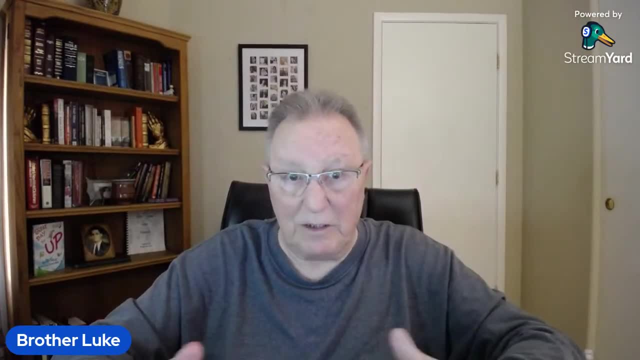 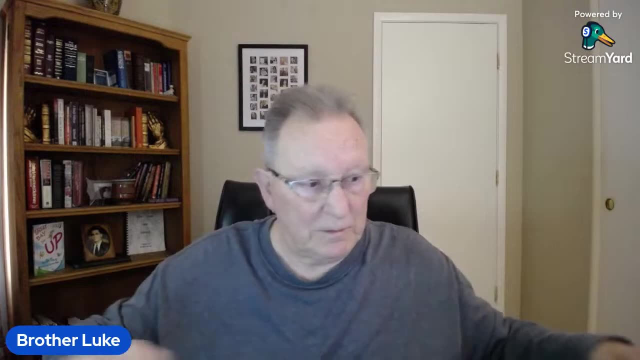 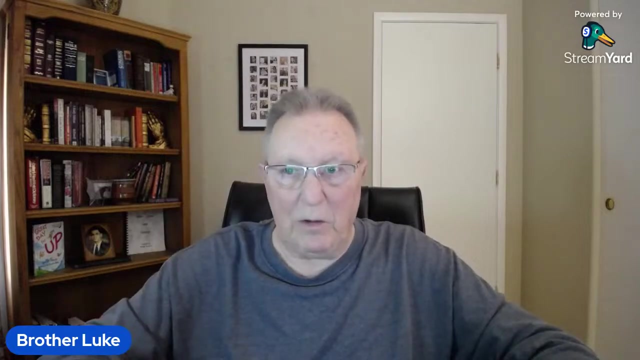 If you put a comment or question in all caps, I assume it's for me. But, Tom and anybody else I want to ask you- and Glenn, you've also made some comments about this today. You're probably all aware that my original YouTube channel was Sin City Preacher. 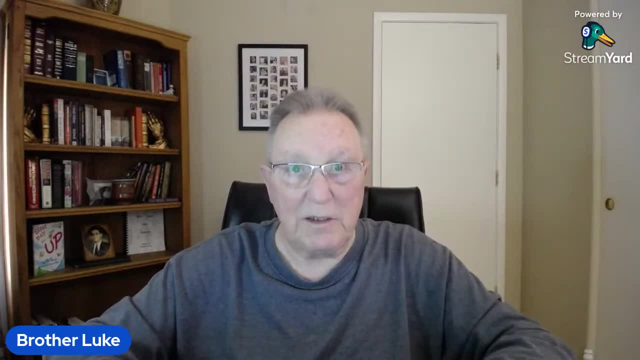 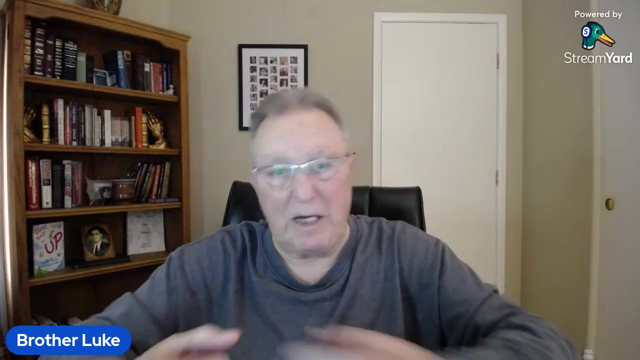 And we first started doing our church programs on my Sin City Preacher channel. but we got in trouble with YouTube over a photograph that we showed that was without permission And they closed my channel down. I mean, I had seven days to scramble to save everything and move it to a new place. 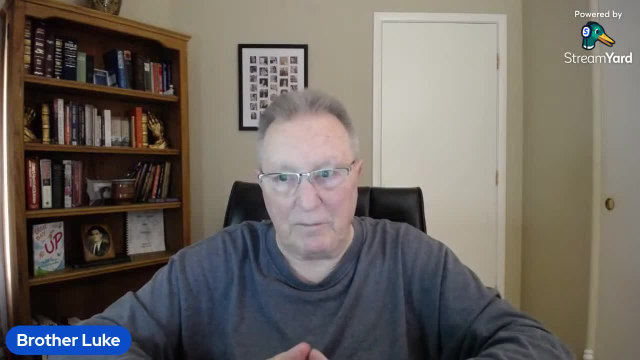 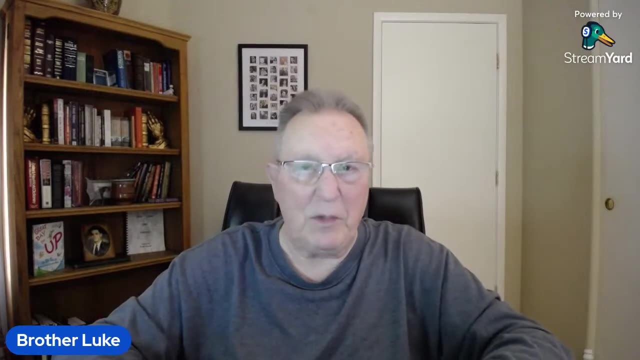 And It was very unjust the way it was done, but we are at the mercy of YouTube, So there are several things I ask everybody to avoid discussing in the chat room, because there are potential problems with YouTube And we don't want CES to suffer consequences because we're making mistakes, talking about things that they don't want us to talk about. 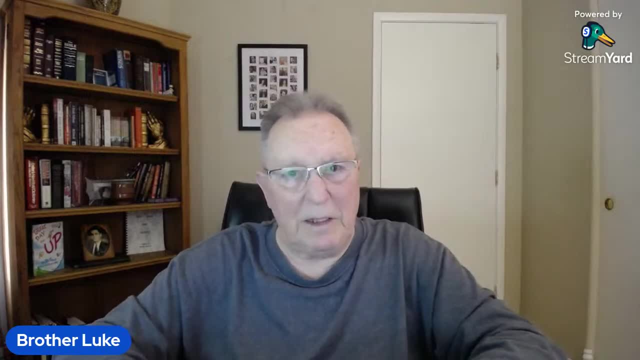 I know I don't like it either, But where they have the power, So we have to operate under their guidelines. So anything, any comments you're making regarding medications, medical procedures, that could be construed as you possibly giving out medical advice. 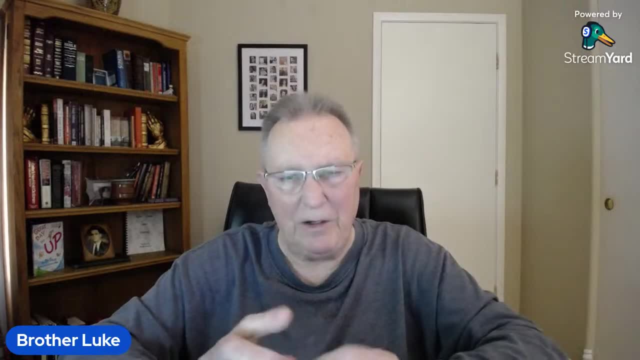 I'm going to ask you to remove any of those comments And let's not make any comments like that, Because we're risking the CES channel getting punished for it. I'm sorry, but that's the way it is And that's the world we have to operate in. 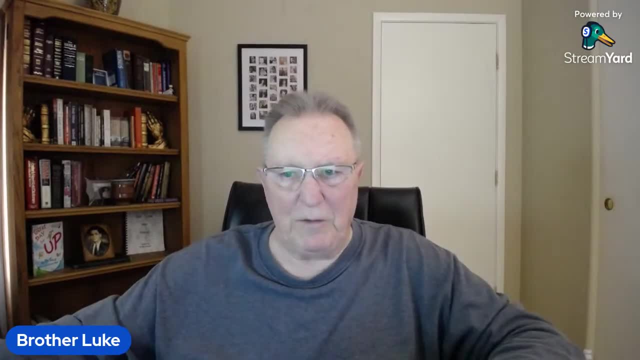 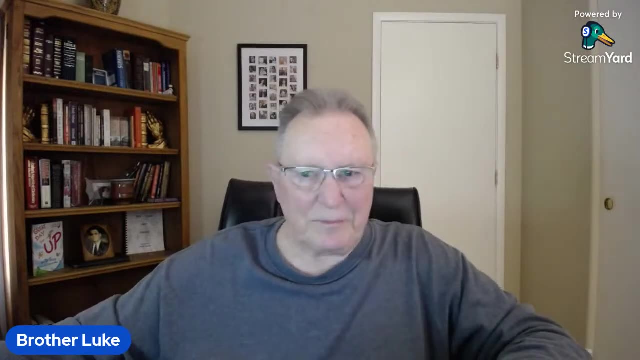 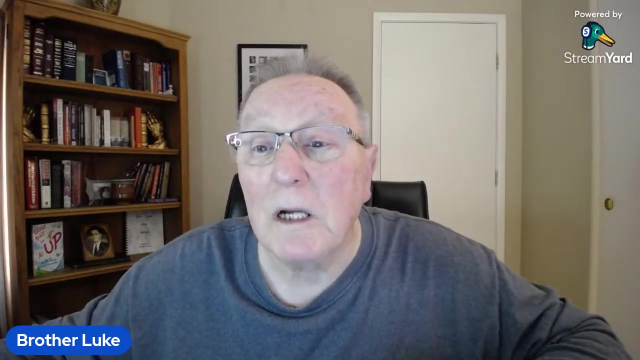 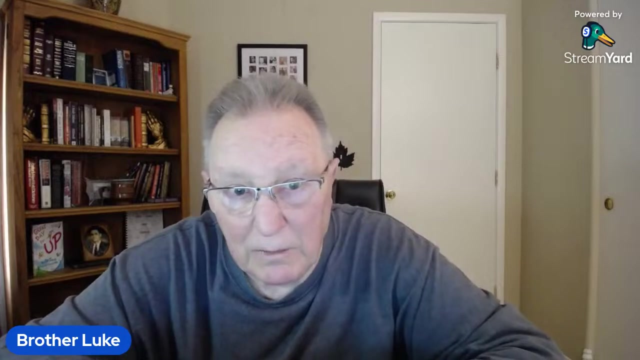 So please remove the comments if you've said something that would violate that. Let me start here at the top saying hi to everybody First. hello, Brother Tom, and blessings to you, And I hope you can get either medical help for your problem or the Lord. 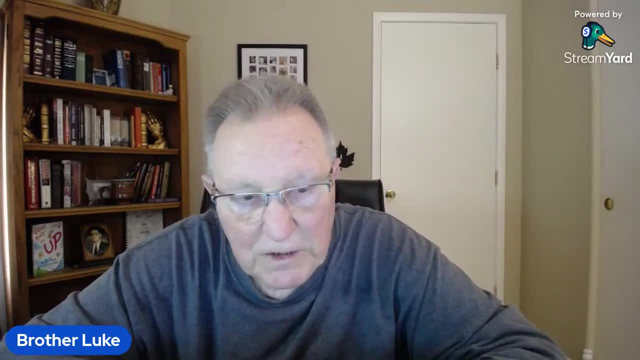 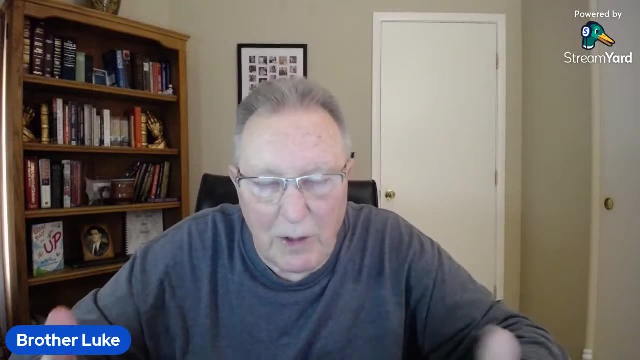 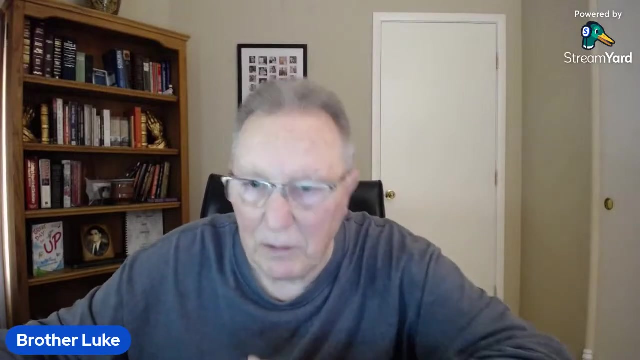 Pray, the Lord will just give him a miraculous healing. Isn't that always the best thing? And when we get healed and we know that there was no other explanation but the Lord came to our rescue, It gives us a chance to boast in the Lord and give all the glory to God. 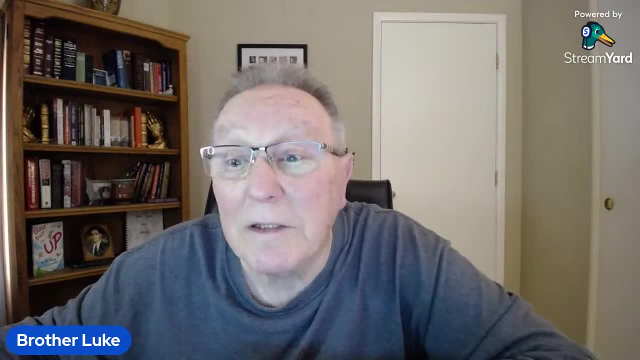 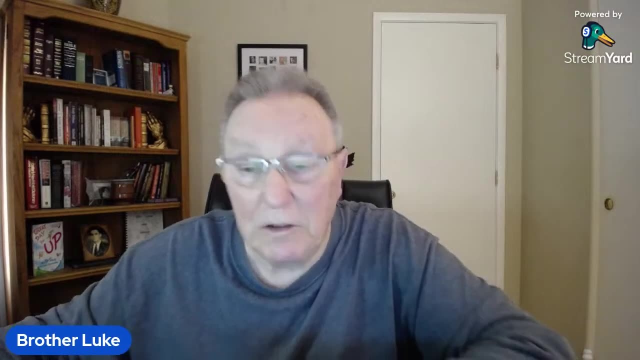 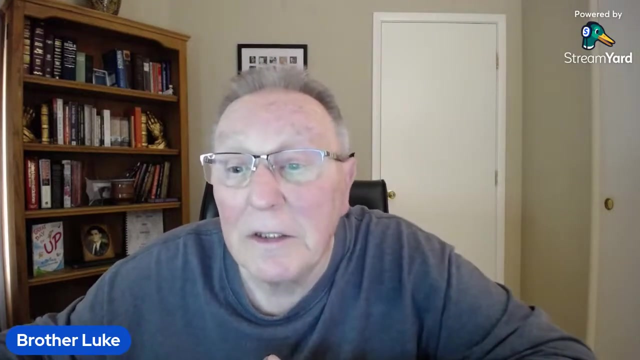 Brother Glenn's here too. He says hi to everybody And let me see. You know, since Sister Shelly hasn't been able to be the moderator, We're depending on the other moderators more now than ever. Tell me if we do have anything to greetings or help that's needed in the chat room. 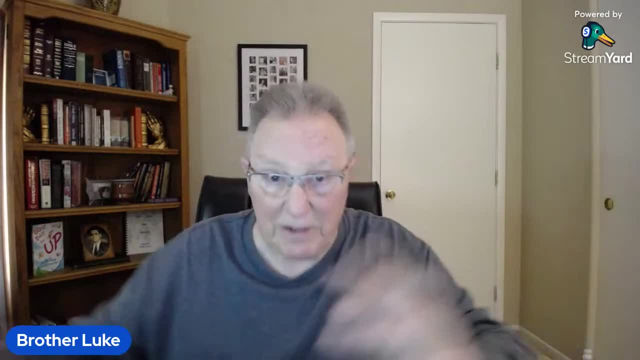 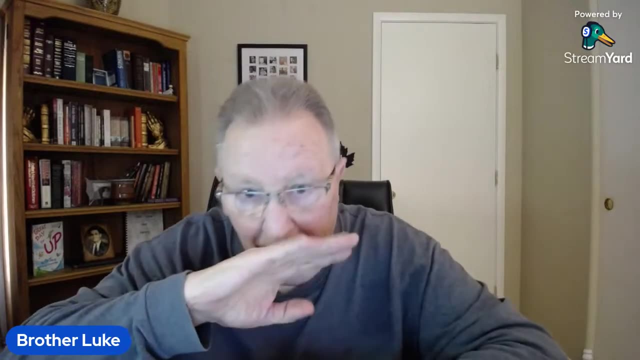 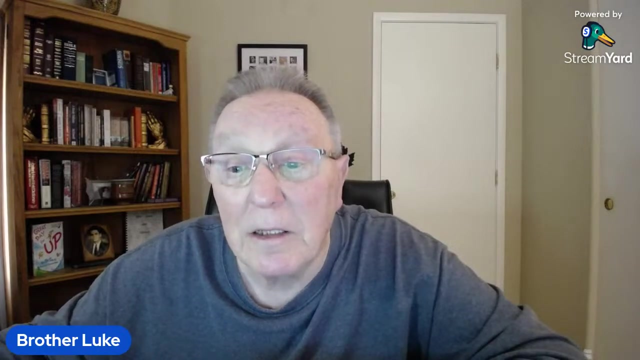 If you're a moderator, please come to help out, especially now, because Renee is not here. It's just me. I have to juggle so many things I need. I need your help. Sugar Swan is here. Sugar Swan, Hello. 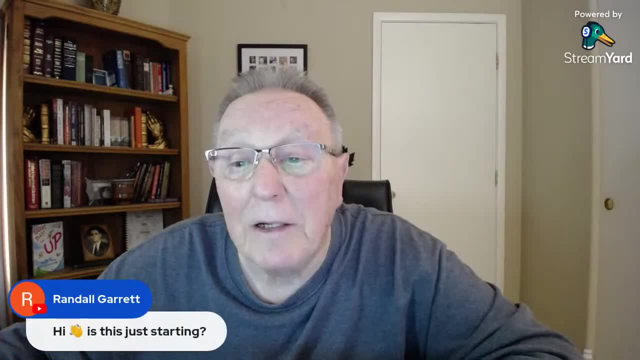 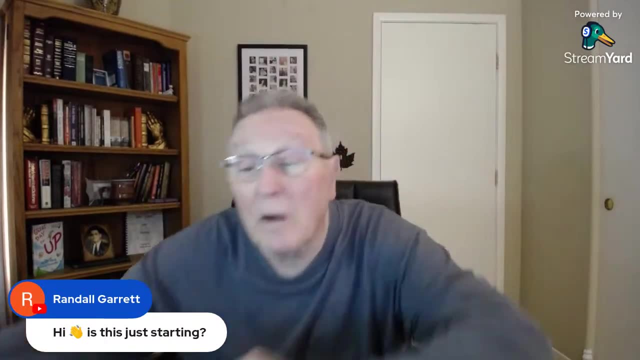 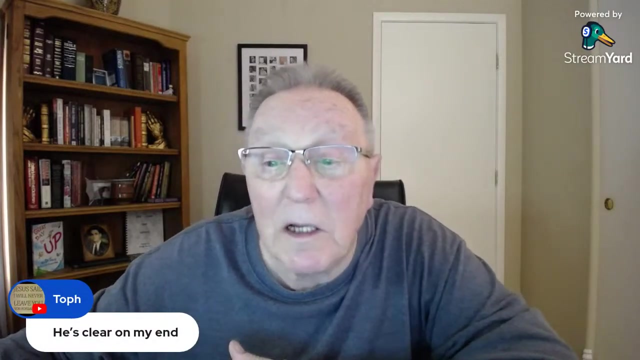 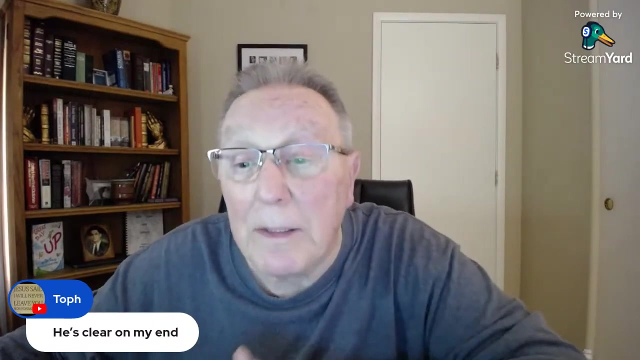 And Randall Garrett. Hi, is this just starting? Yeah, just started seven minutes ago. Brother Tov, Hi Hi, He's clear on my end. Is Brother Luke cutting out a lot for anyone? Yeah, Let me know, Am I? 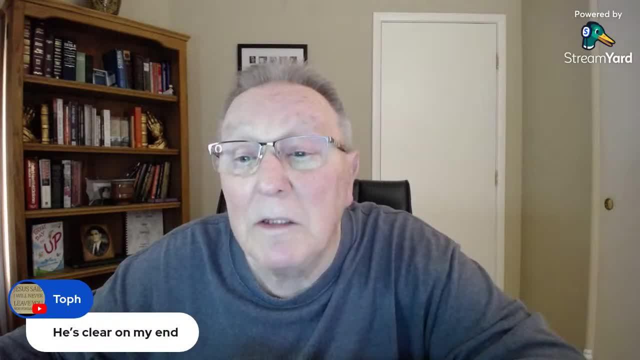 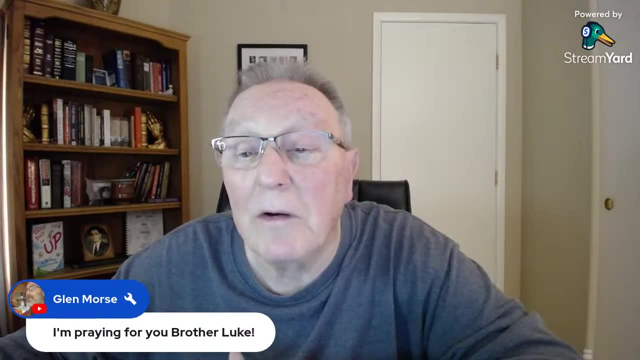 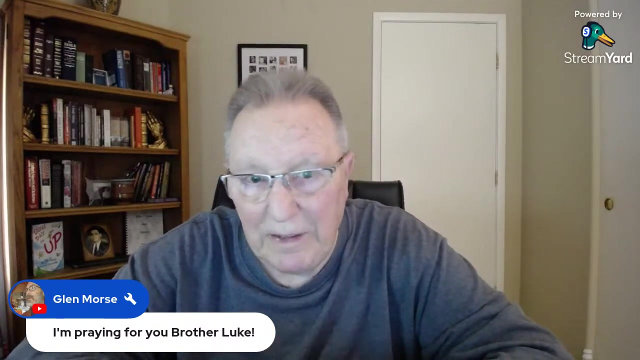 Is there a problem? Let me see- Tov says he's clear on my end, Glenn praying for me. Thank you, brother. Everybody, Please pray that. I think it's going to go away. It's been 12 days and I have a sister. 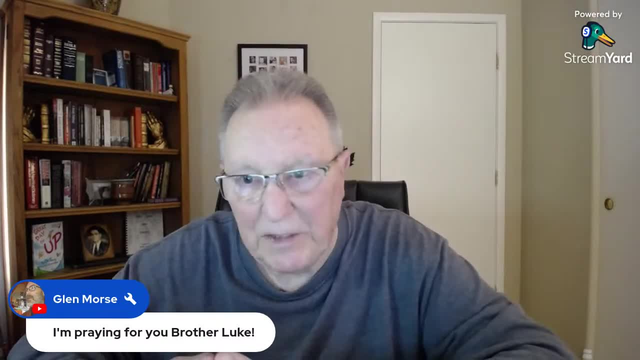 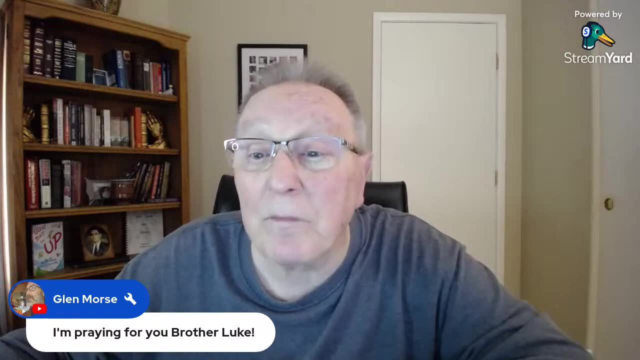 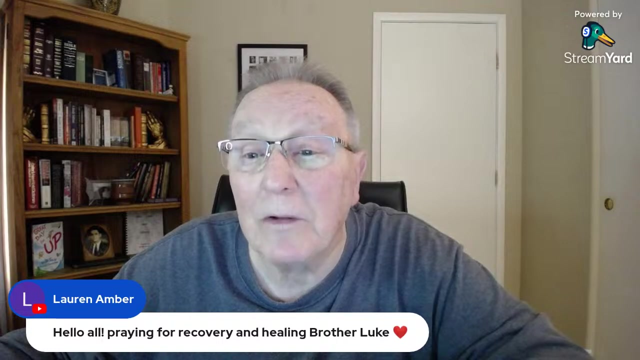 And then There's other people I've known that seem to have the same kind of a thing, And it just seems to go on for at least two weeks or more. So, and Lauren Amber says hello, All praying for recovery and healing by the look. 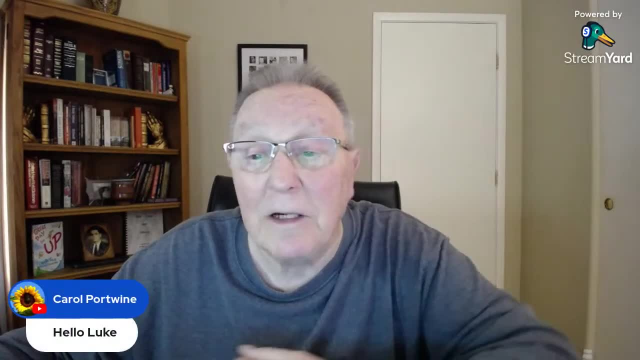 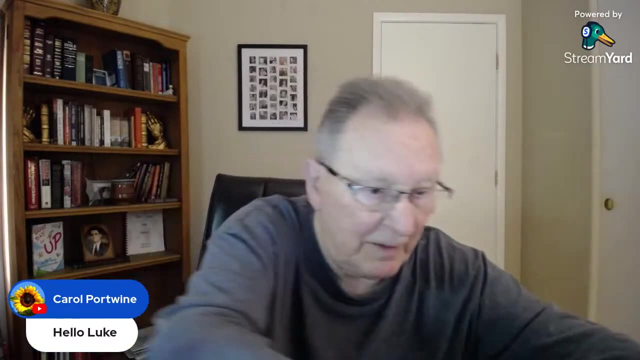 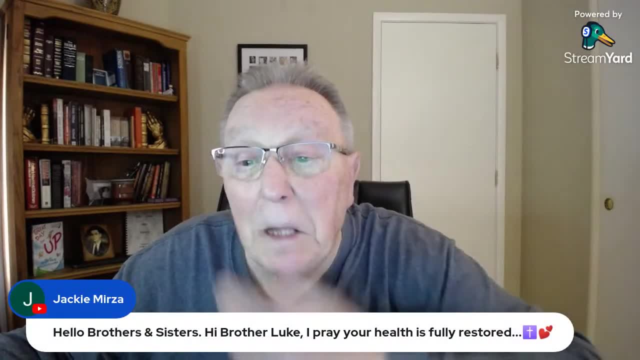 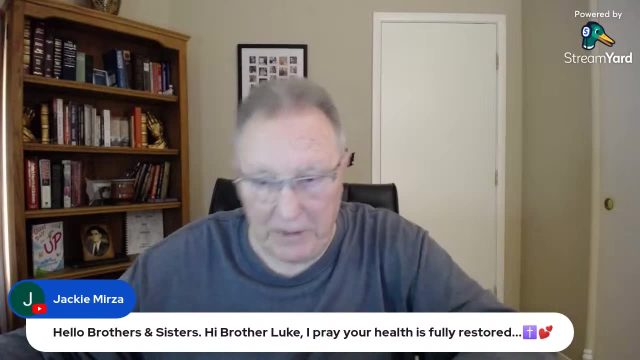 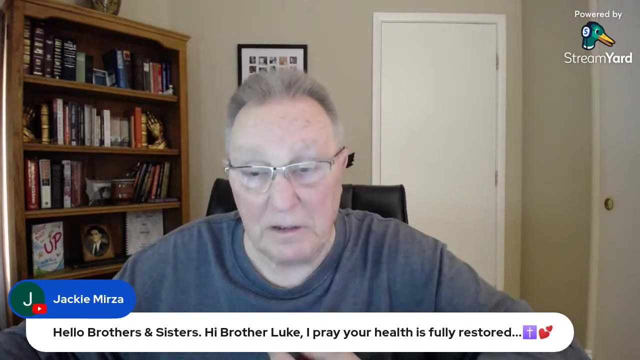 Bye, Bye, Bye, Bye, Bye, Jackie Marza. Hello brothers and sisters. Hi reserve Luke, I pray your health is fully restored. Thank you, All these aids here, just throw lozenges, Actually helping quite a bit. 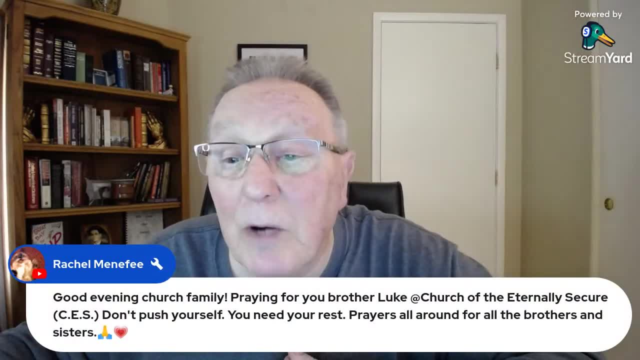 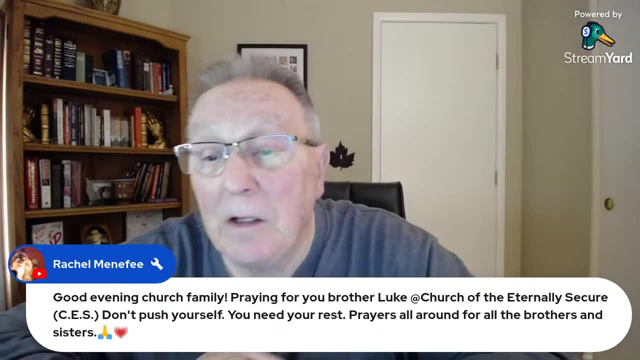 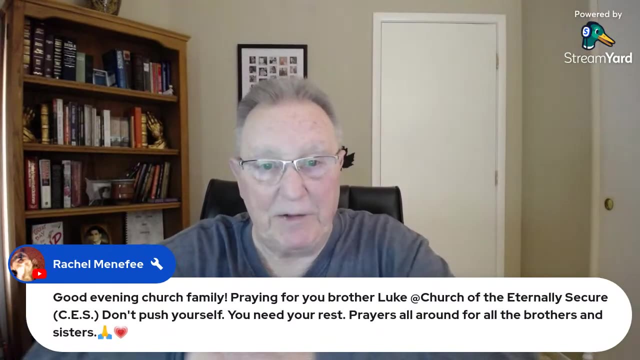 In Ergeb Good evening Church. Family praying For you by the look, Don't push yourself, You need your rest. praying all around for all the brothers and sisters. that's good. you know i keep saying this. i guess it can't be repeated too much. uh, while we're on a live program, we're asking for prayers. 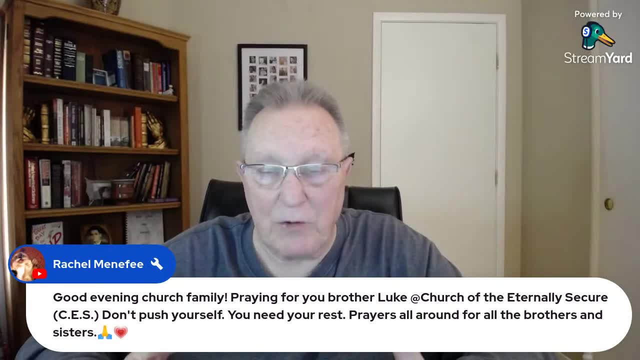 for each other. but when the program's over, are you still praying? i hope that you'll pray every day for each other and, uh, you know, we don't even have to remember the details. the lord knows. you can just simply say: ask the lord to to help all those at ces who have asked for prayers. 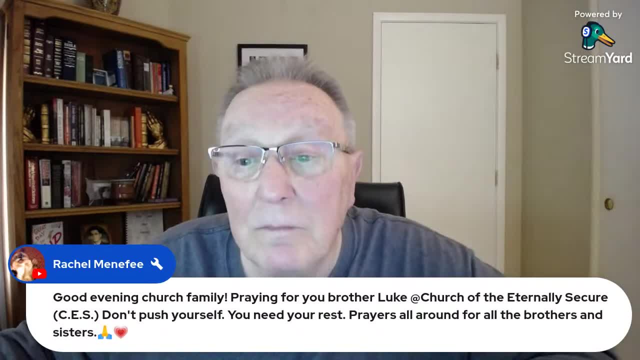 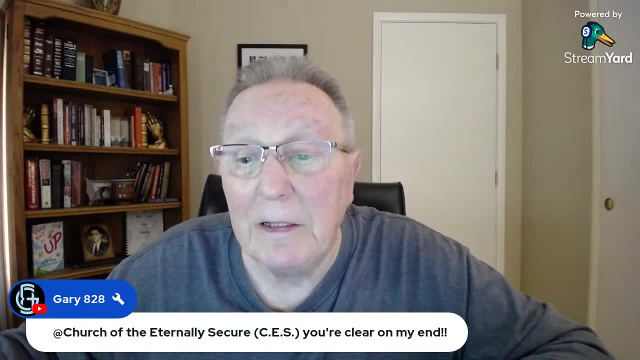 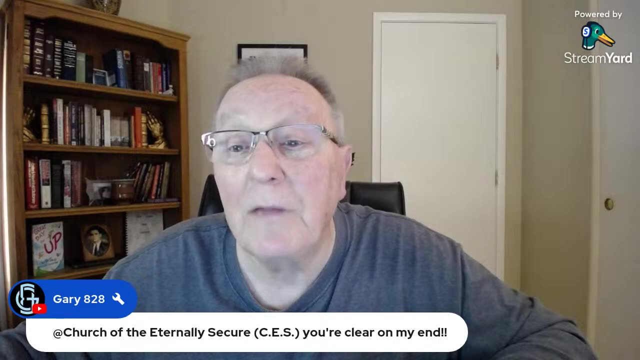 that's that simple. diane says prayer for you, brother luke. thank you, diane, gary. uh, you're clear on my end. yeah, if any anybody is having a problem other than i think it was sugar swan, said she and it wasn't hearing me clearly. if anybody else is having a problem, uh, let me know, but apparently it's probably just. 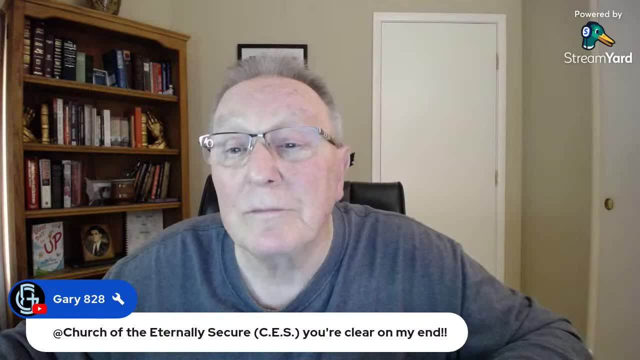 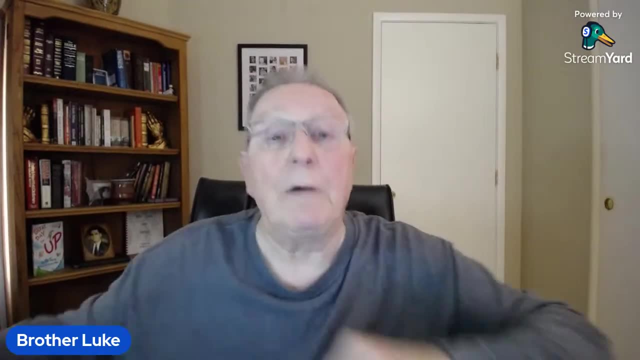 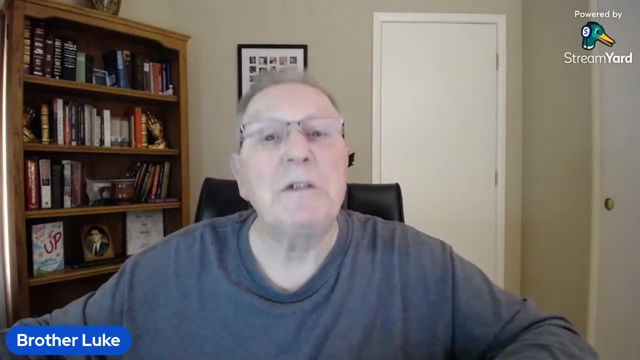 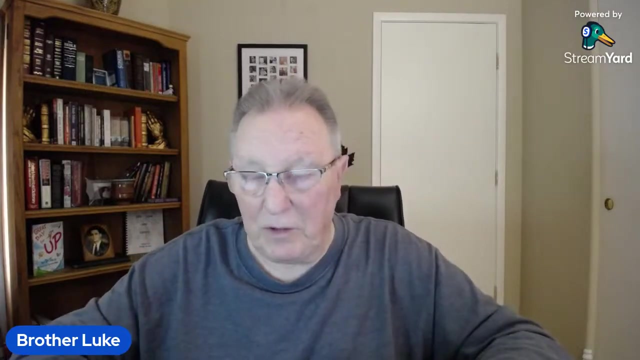 on on your end, sugars one. okay, all right, so at least i've been able to say hello to everybody. oh, now we do have some questions that have been sent in and uh, let me see there's also one prayer request, and so, uh, in the chat room during the program, any prayer needs or 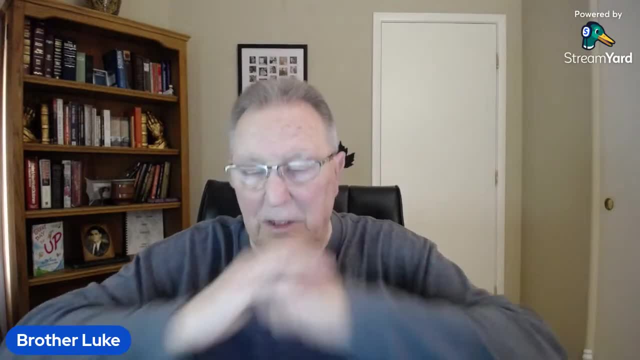 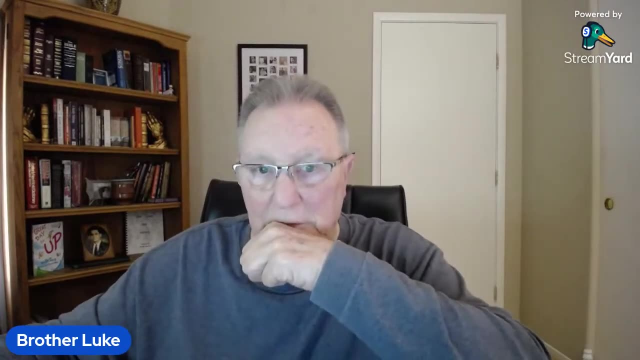 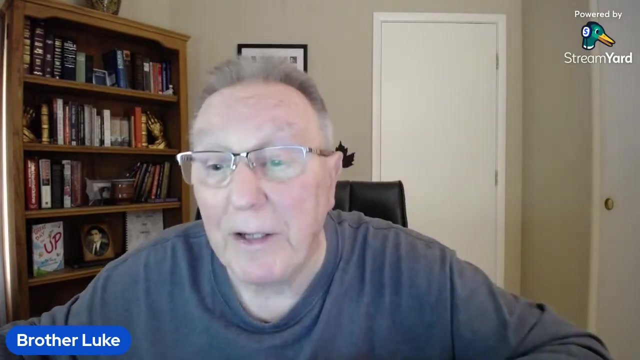 any questions today, put them in all caps. uh, especially today, it's got to be in all caps, because that's the only way you're going to be able to get my attention, and i've got a few other old subjects in mind that i would like to talk about anyway, so there's plenty of things to talk. 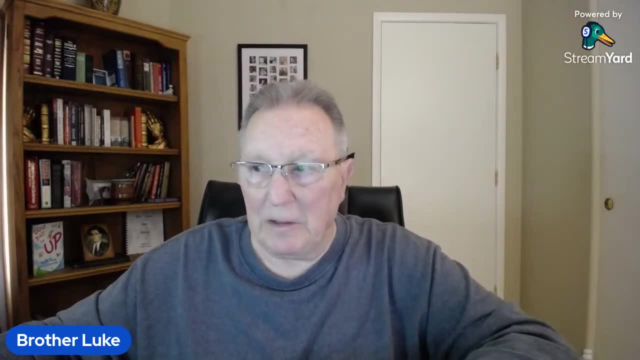 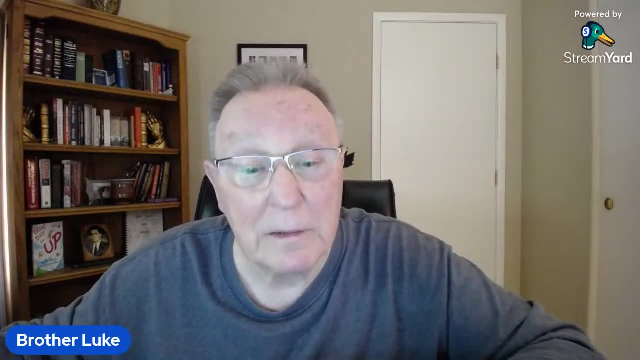 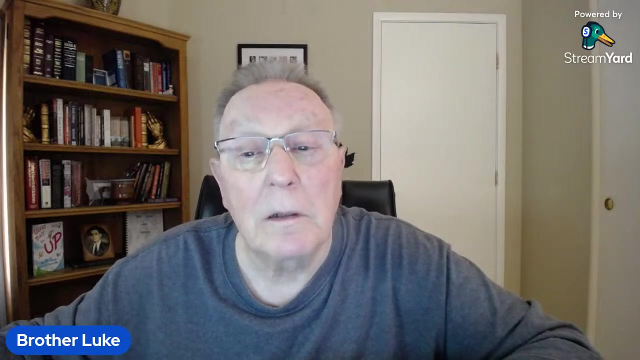 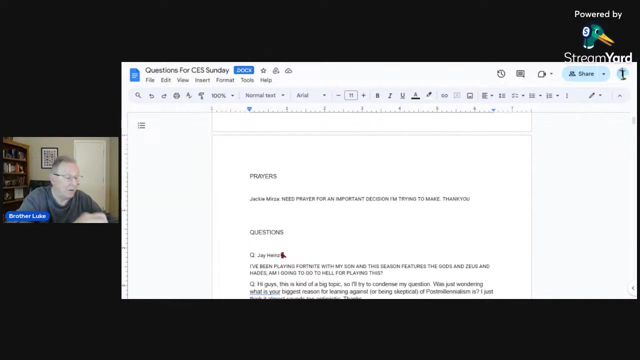 about as usual. um, so let me tell you the prayer request that was emailed. this one's from jackie marza. let me put it on the screen. that's a friend of mine here in town. i have to say no to him. um, okay, um, let's see. uh, yeah, here it is on the screen. uh, jackie wrote: uh need prayer. 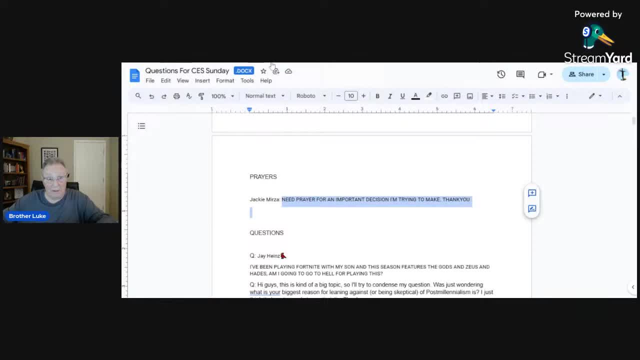 for a important decision i'm trying to make. all right, jackie has a big decision. ask the lord to guide her and, uh, you know, give her the right answer, give her confidence, confidence going forward, and then help her to uh move and do whatever she has in mind and get it. 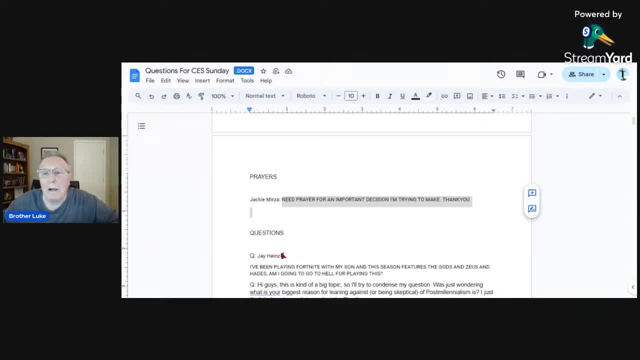 accomplished. um, let me see, i'll keep on looking for anything in caps from you as we go. um, i guess, uh, since i don't see any prayer requests, we'll just talk. we'll. we'll do communion. before i run out of gas, at least let's get a communion in. 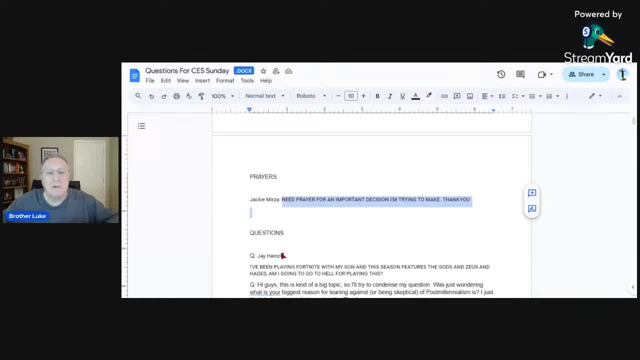 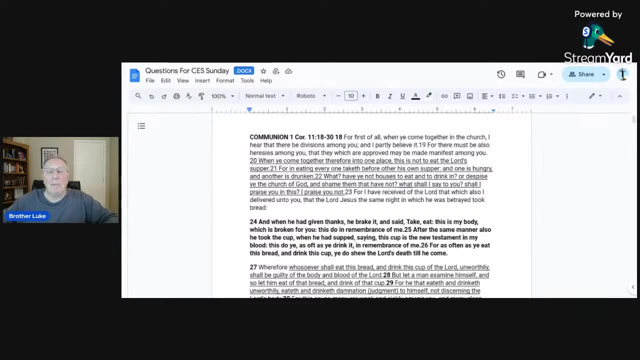 right now i'm showing on the screen the verses pertaining to communion that we discuss this. if you have your bibles ready, you can look at first corinthians, chapter 11, verses 18 through 30.. i'm going to read it all in context. 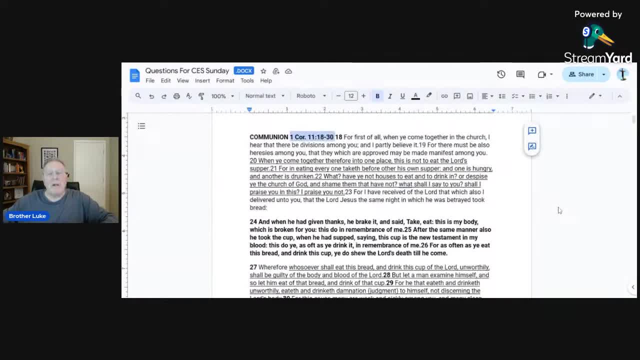 context and and then elaborate a little bit. it says um, for first of all, when you come together in the church, i hear that there be divisions among you, and i partly believe it, for there must be also heresies among you, that they which are approved may be mad, made manifest among you. 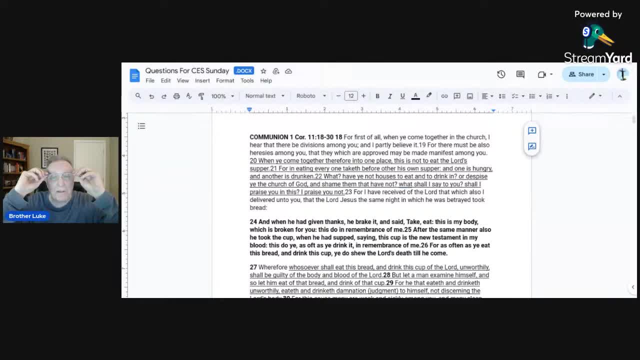 when ye come together, therefore, into one place, This is not to eat the Lord's supper, For in eating, every one taketh before other his own supper, and one is hungry and another is drunken. What Have ye not houses to eat and drink in? Or despise ye the church of God and shame them that have not. What shall I? 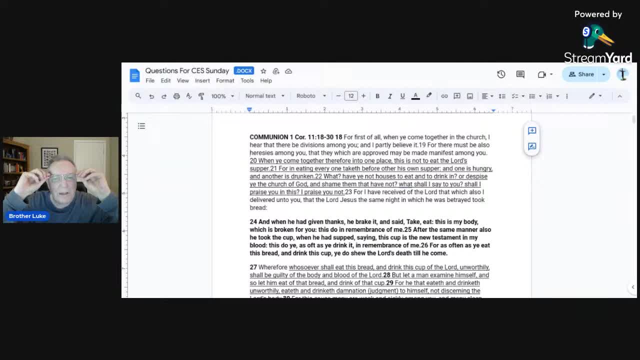 say to you: Shall I praise you in this? I praise you not, For I have received of the Lord that which also I delivered unto you, that the Lord Jesus, the same night in which he was betrayed, took the bread. I want to pause for a second. The portion I just read explains what the problem is. 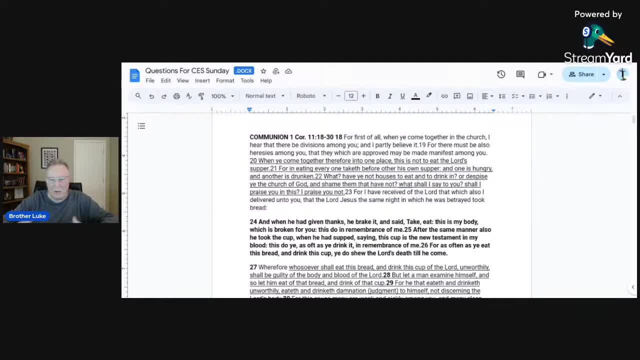 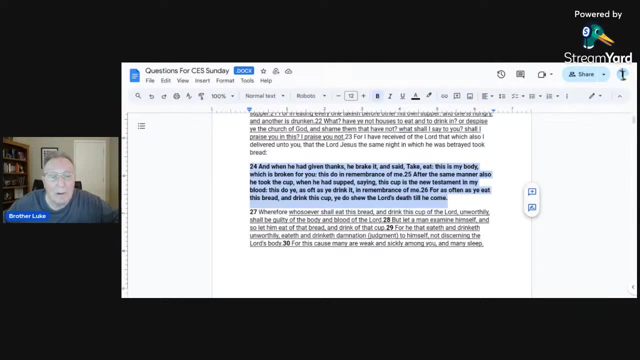 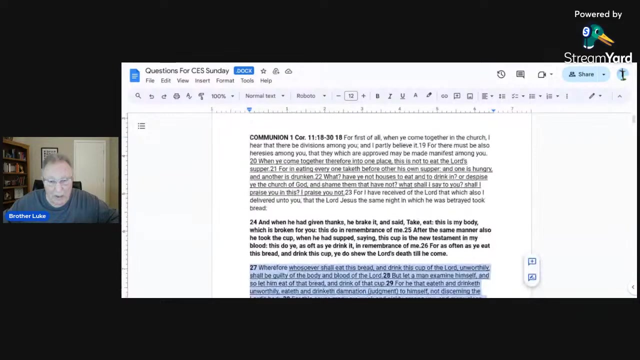 at the church at that time. that caused Paul to issue this warning. It's coming up. I'm going to skip the actual verse 24 through 26.. We'll do the communion when we read that. But then Paul goes on in verse 27,, referring to what he said originally. He says: 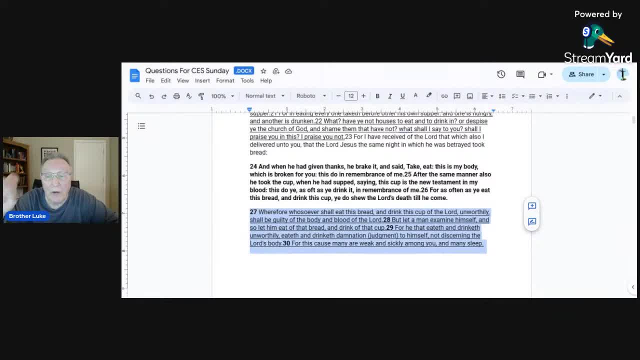 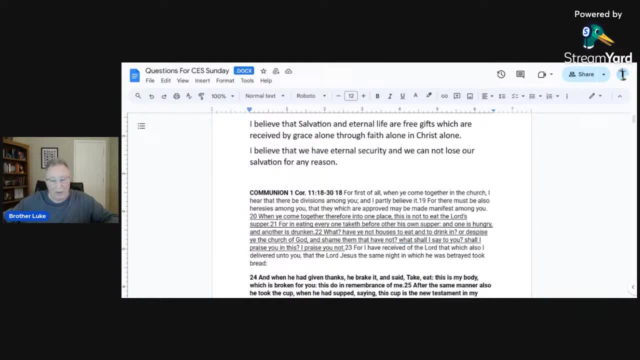 Wherefore whosoever shall eat this bread and drink this cup of the Lord, unworthily, Unworthily, is referring back to his complaint in the previous verses I read: They're eating and they're taking more than their share of food. They're being gluttonous. They're taking drinking too. 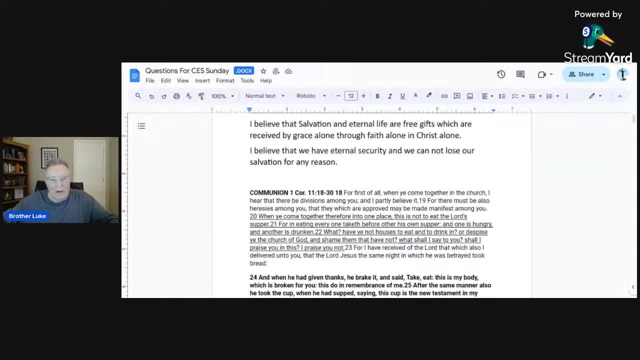 much, even getting drunk, And they're not respecting people. They're giving favoritism to people who are, let's say, have more status or wealth than the needy people. This is all going on And Paul says: if that's the way you're conducting yourself. 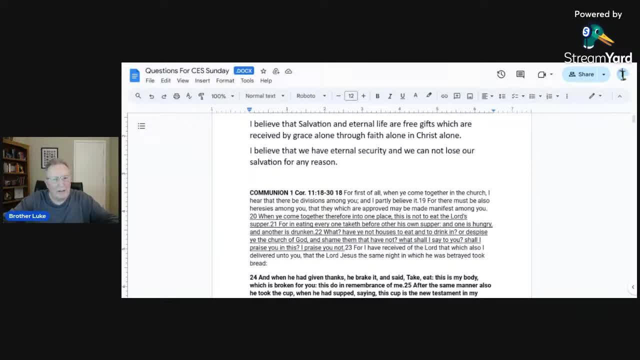 you're not doing this in a worthy manner. You need to repent of that, And now. instead, don't come here to try to have a feast and take advantage of the situation, get a lot of wine and free food and ignore the people who actually are hungry. So that's what the issue is. 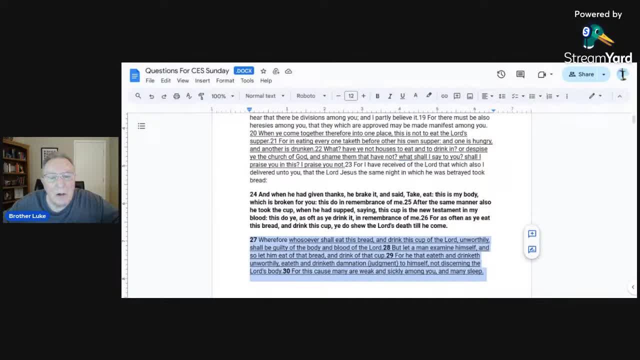 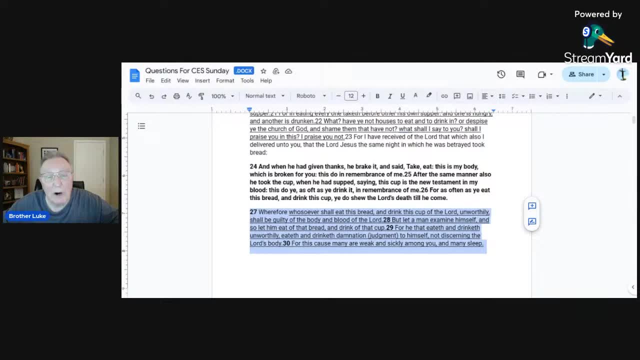 That's what he's referring to when he says: Whosoever shall eat this bread and drink this cup of the Lord unworthily shall be guilty of the body and blood of the Lord. In other words, the Lord's body was beaten and crucified and died. 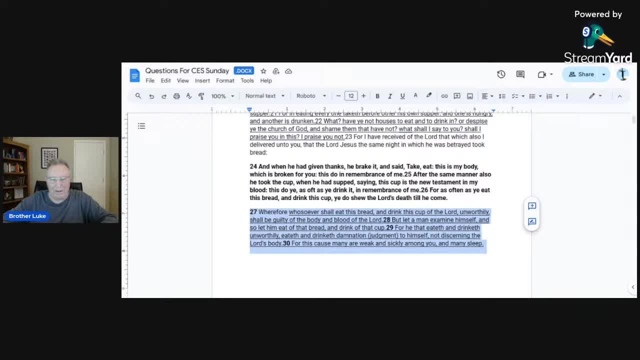 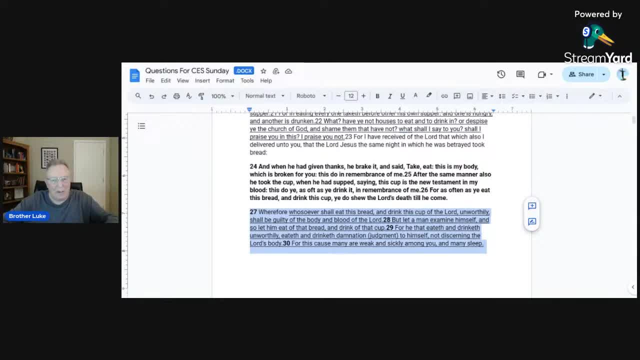 because of breaking Jewish laws. It was because he was paying for our sins. He said: this is the very reason he came down from heaven and became a man, He said. Jesus said: do not think I came to be served, but rather to serve. 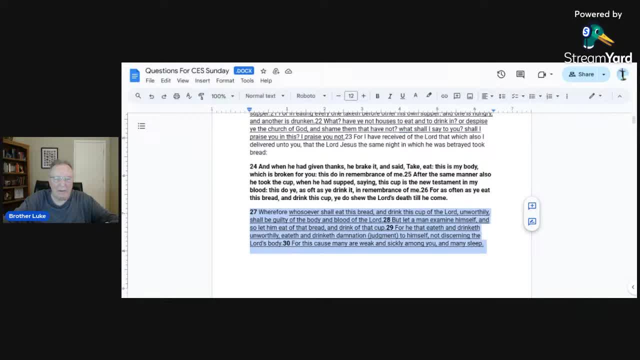 And to give my life as a ransom for many. So he came to serve, And by serving he gave us an example of how to be a servant. And he came to give his life to die as a ransom, as a payment. A ransom. 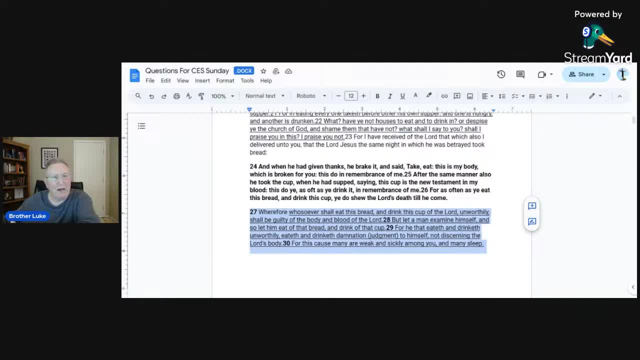 is a payment made to set a captive free, So his death serves as a payment to set us free from the penalty of sin. So that's really what Paul's warning is all about. It has nothing to do with the Roman Catholic position that taking an unworthy means you haven't yet gone to the priest to confess your sins and that makes you eligible for communion. That's how they would teach on this verse. 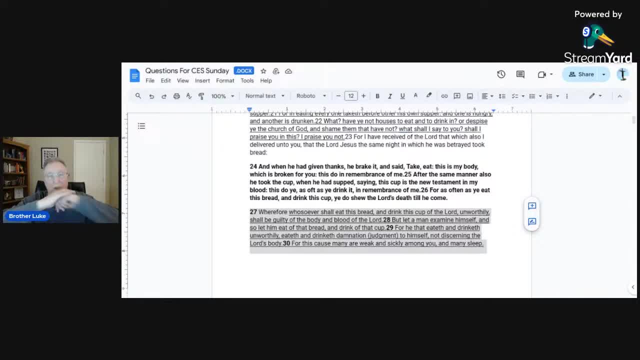 Even a lot of Protestants, I know, have interpreted this portion of scripture in that way. But that's the way it is, But that's not what the problem was. Okay, now that we understand, if you can take communion in a worthy manner, that means with respect and reverence for what it represents. 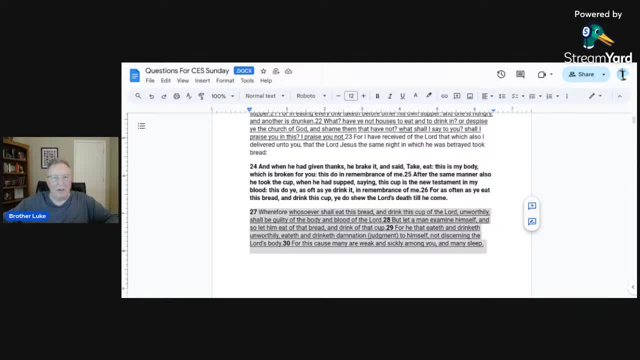 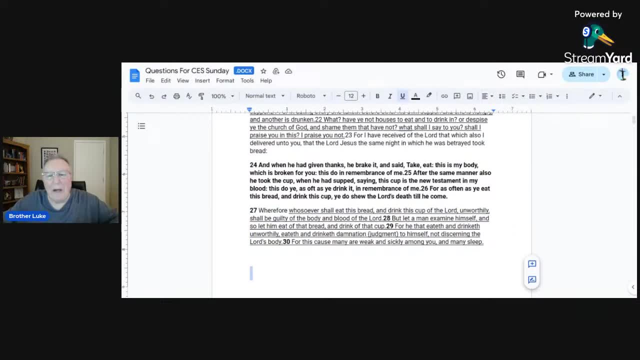 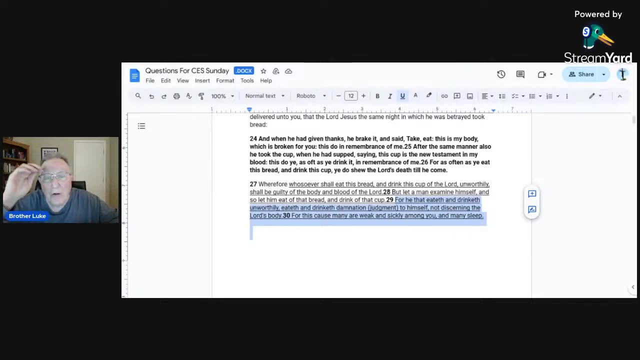 then I invite you to join us in communion, provided that you're a believer, Because when it says here at the end, it says: He that eateth and drinketh unworthily eateth and drinketh damnation or judgment to himself, not discerning the Lord's body. 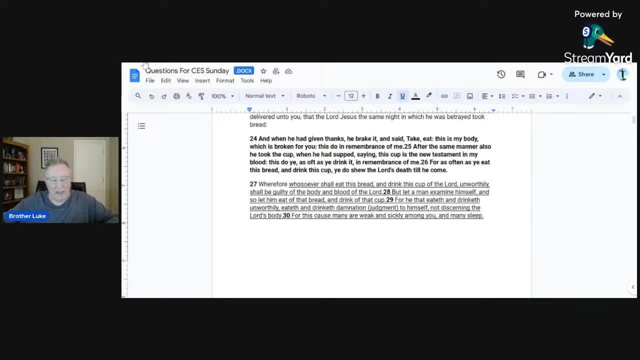 Not discerning the Lord's body. Renee has an interesting take. She says: not discerning the Lord's body is not recognizing the body of Christ. The members, all the believers, make up the body of Christ and you're disrespecting them by the way you're behaving. 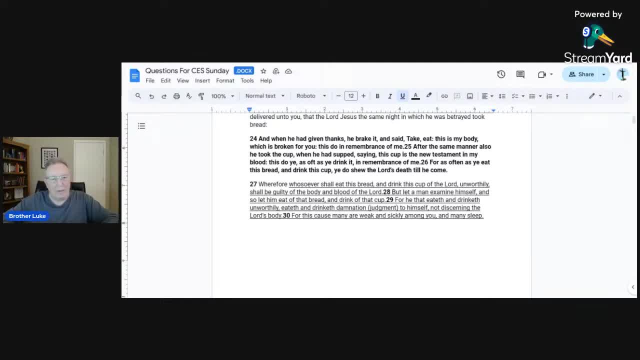 That's an interesting take on it. I think it means, though, that you're not discerning the Lord's body. You're not understanding. the purpose of this is to remember that he died for our sins. His body was broken, and he bled and died to pay for our sins. 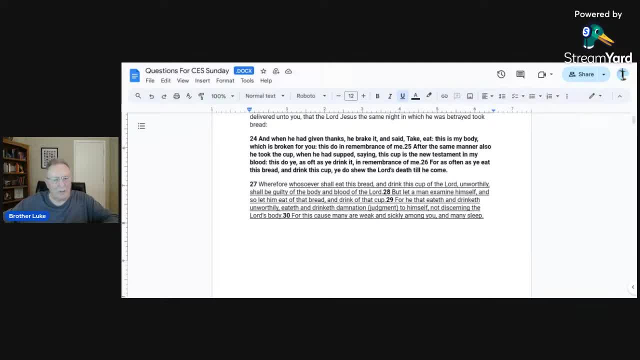 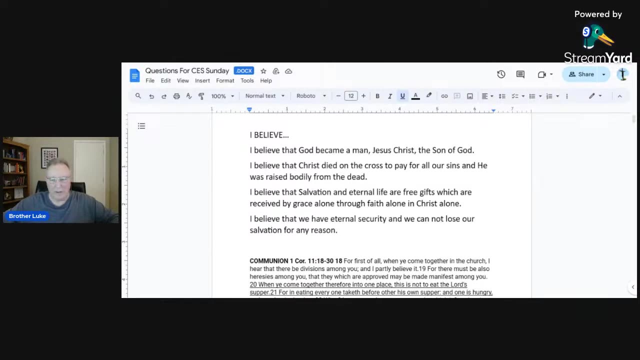 That's not discerning the Lord's body. if you don't understand and recognize and believe that, All right. if you're ready, let's see what is required for you to be considered a believer. I have four points on the screen. 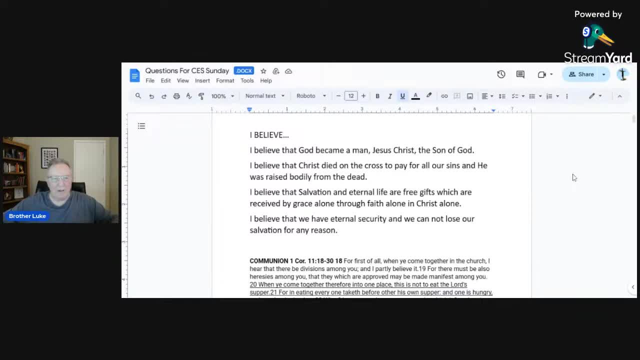 As I read each of these points. if you understand and believe it, say amen. First. I believe that God became a man, Jesus Christ, the Son of God, Amen. I believe that Christ died on the cross to pay for all our sins and he was raised bodily from the dead. 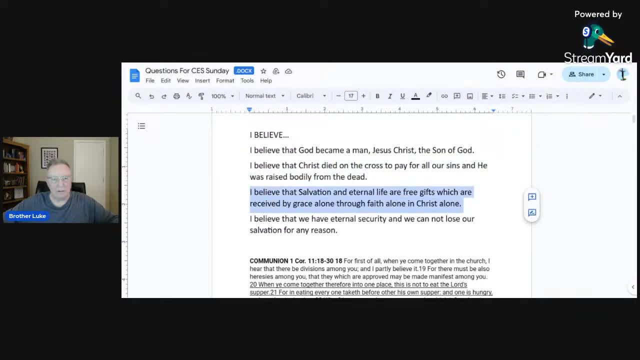 Amen. Second, I believe that salvation and eternal life are free gifts which are received by grace alone, through faith alone in Christ alone, Amen. And I believe that we have eternal security and we cannot lose our salvation for any reason. 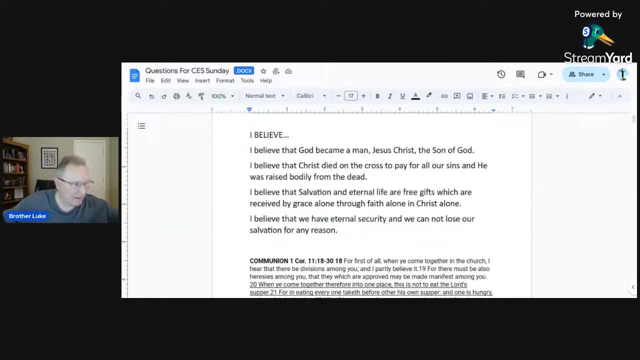 Amen. Okay, I think these are the basic tenets of the faith: The faith of Christ as it's written in the Bible. The faith of Christ, the doctrines of Christianity. Okay, so let me see Before we do this anything. 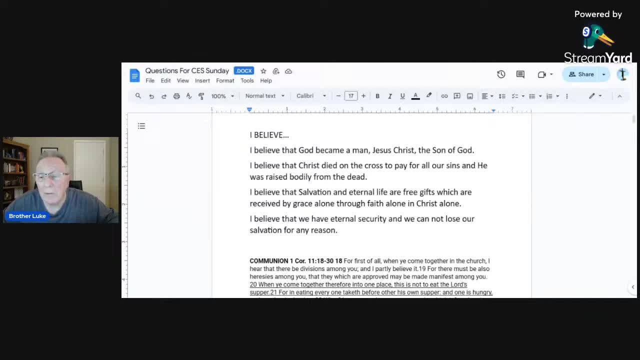 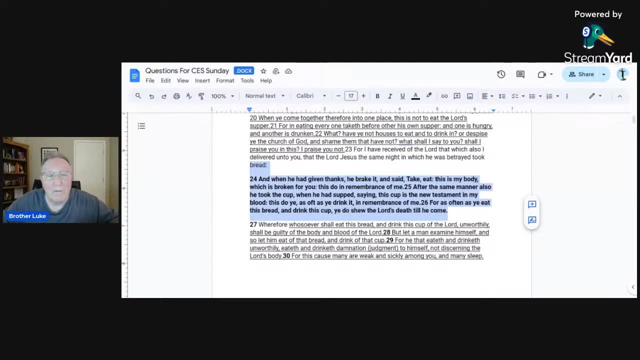 Anything in the chat room I need to know about. Okay, if you're ready, let's do our communion together now, And we're going to focus now on verse 24 through 26.. Follow along with me. And when he had given thanks, he break it and said: 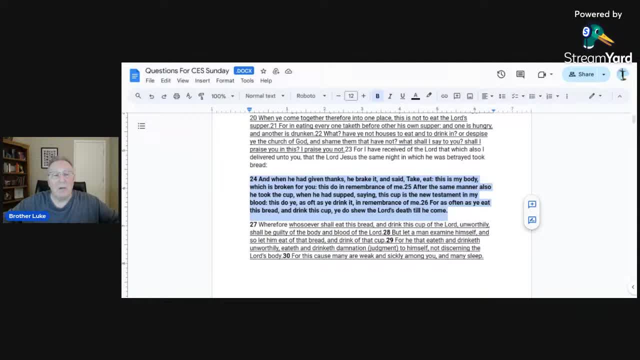 Take, eat. This is my body which is broken. for you. This do In remembrance of me. After the same manner also, he took the cup when he had stopped saying: This cup is a new testament in my blood. 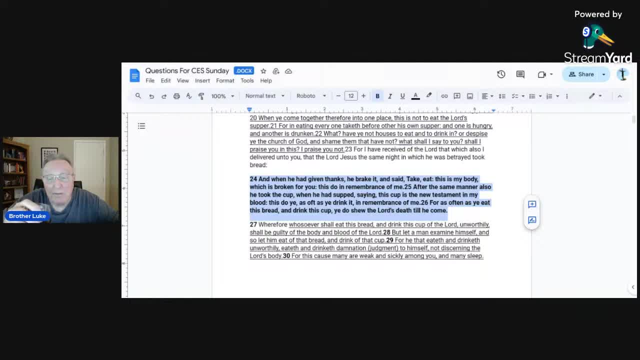 This, do ye as often as you drink it In remembrance of me. For as often as ye eat this bread and drink this cup, ye do show the Lord's death till he come. Okay, I'd like to have a little pop quiz now. 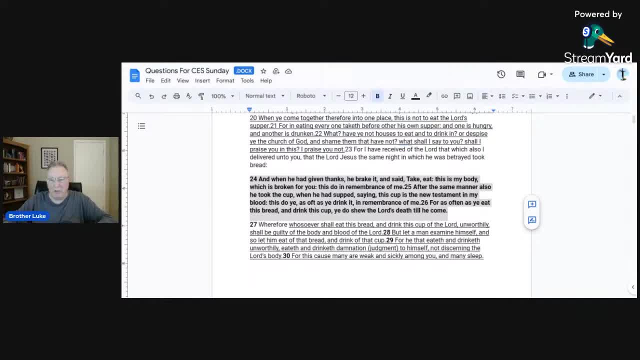 In all caps. if you want to answer my question, put it in all caps. And the question is: why Are we doing communion? Okay, I'll be looking for the questions in all caps. I'll be answering in all caps. 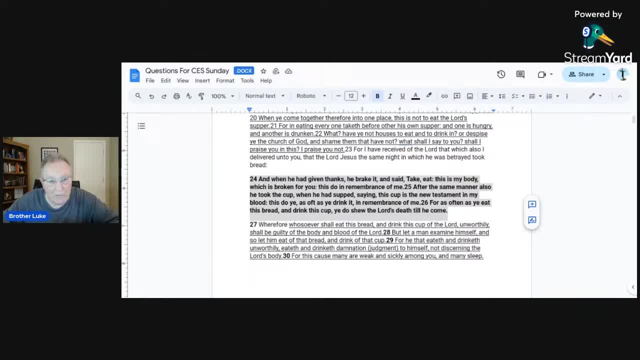 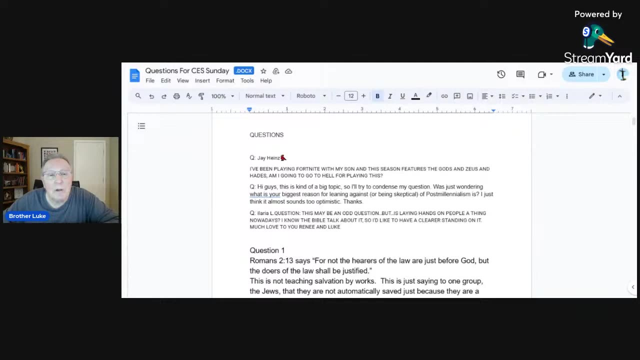 I'm sure most of you understand that, Particularly if you listen carefully. All right, All right, now that we've done the communion, we're ready to start answering some questions. First question here was by Jay Hines. He says: 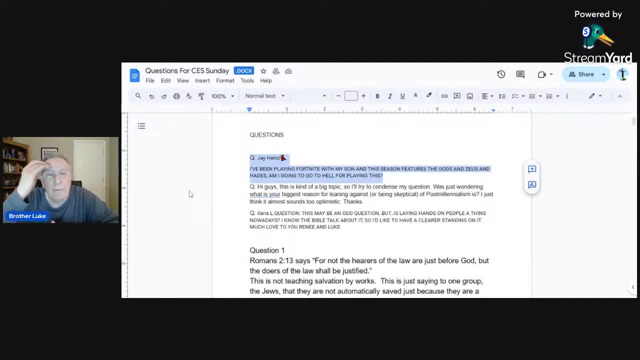 I've been playing Fortnite with my son And this season features the gods in Zeus and Hades. Am I going to go to hell for playing this? Of course we all know Brother Jay. Brother Jay is really advanced, Advanced, He knows. 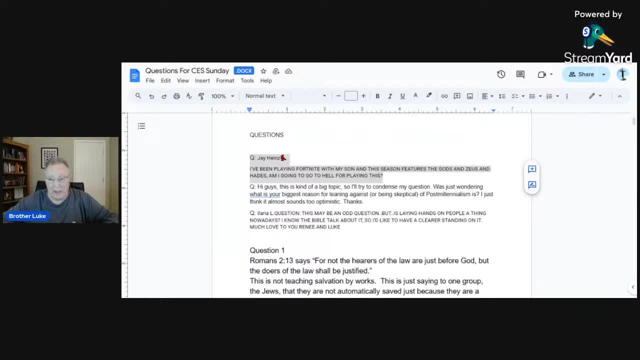 He knows the Bible, So he's asking this question rhetorically. He knows the answer to the question, So he's asking it so that we can discuss it for other people's benefit. I wonder how many of you have questions like that. 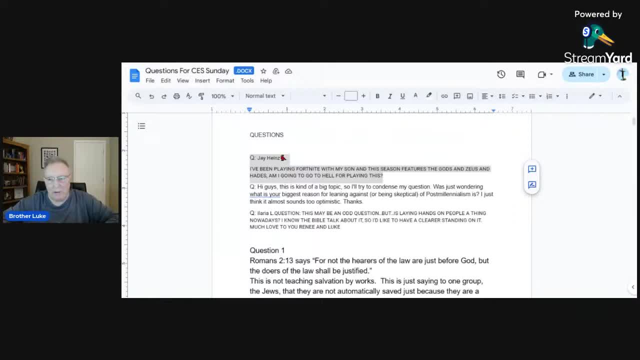 Wondering if this kind of a thing is going to cause someone to go to hell. Well, first of all, we know, based upon the tenets of the faith that we read earlier, that a person cannot lose their salvation. So if someone gets saved by believing these tenets that we just said amen to, 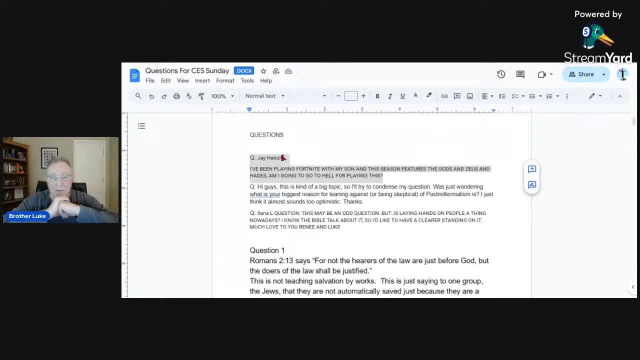 if you believe all that, then you're saved, And that's what you need to understand. I am saved because Jesus is my Savior. I am saved because Jesus paid for all my sins. I am saved, I am saved, I am saved. 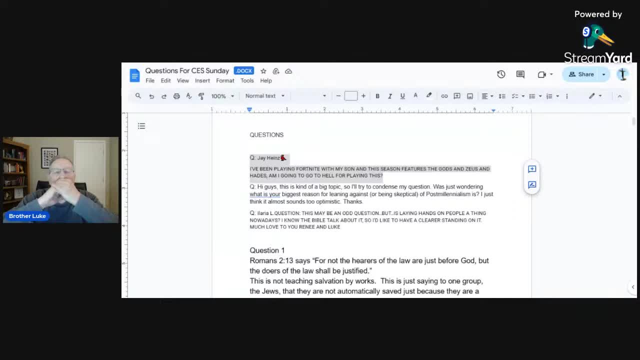 He says that he will never leave me or forsake me. So if that's the case, then playing Fortnite is not going to change it. But now the other question would be: is this a sinful thing to do? Because if we're believers- oh, here's Randall. 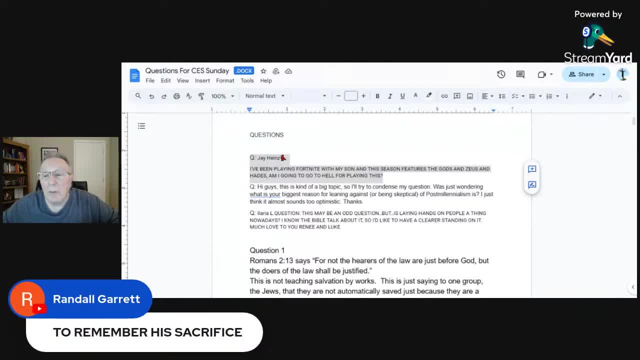 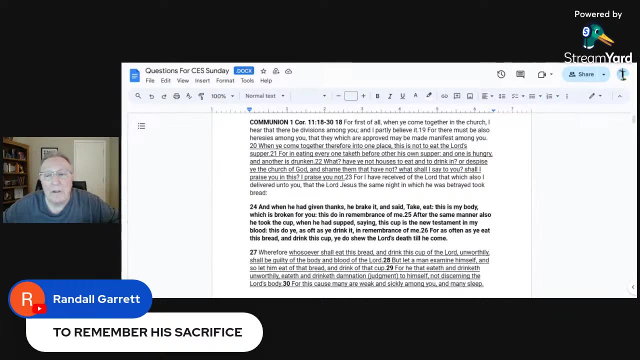 He says: Randall says to remember his sacrifice: Yes, Amen, Amen. In fact let's go back to that communion verse for a second here. And he says: in those verses I read, he says a couple of times: he says: 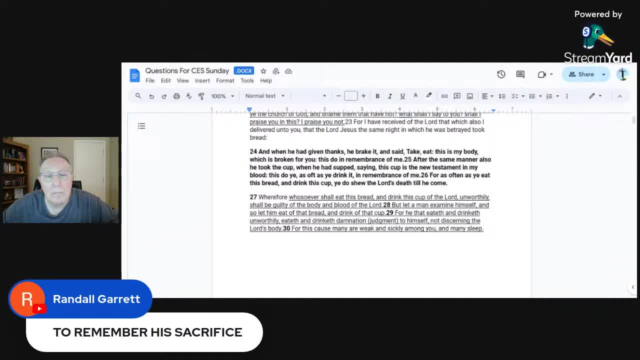 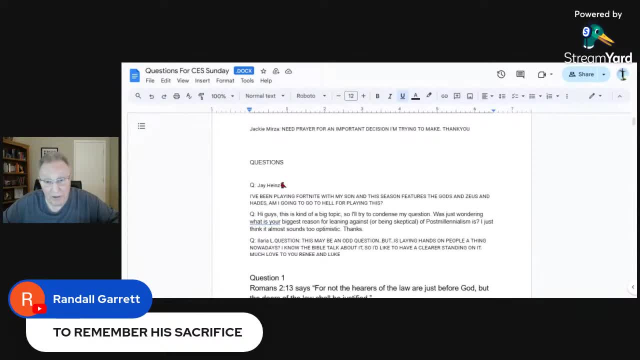 That's why we're doing it, our communion, Because he commands us to do the communion as a ceremony To keep in our minds and remind us what he accomplished for us. Okay, So now, getting back to Jay's question, I think it's time for another throat lozenge. 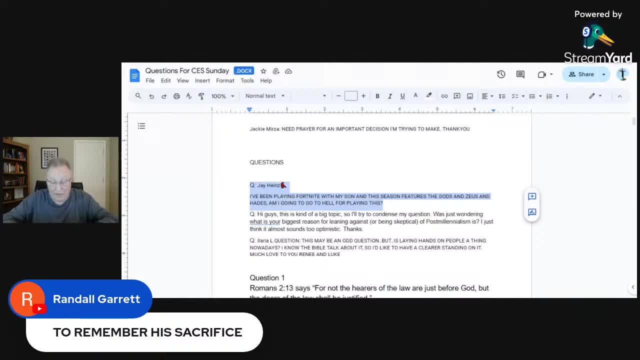 These things don't taste very good. They're my sister's favorite type of throat- lozenge Fisherman's friend. But they're effective. They certainly kind of ease my throat a little bit, But I don't really like the flavor of it though. 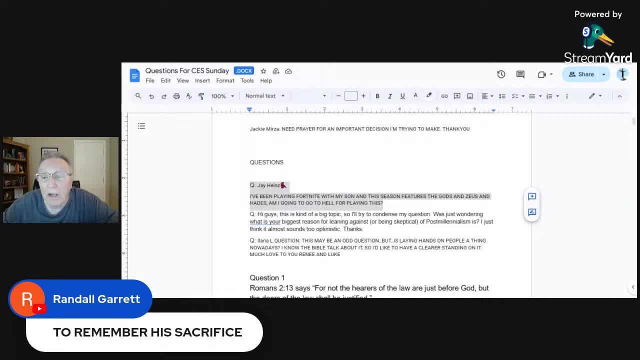 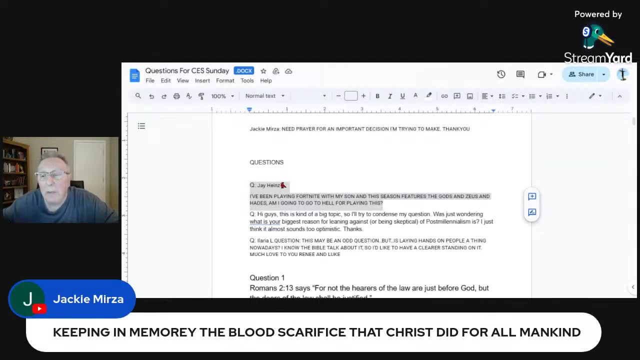 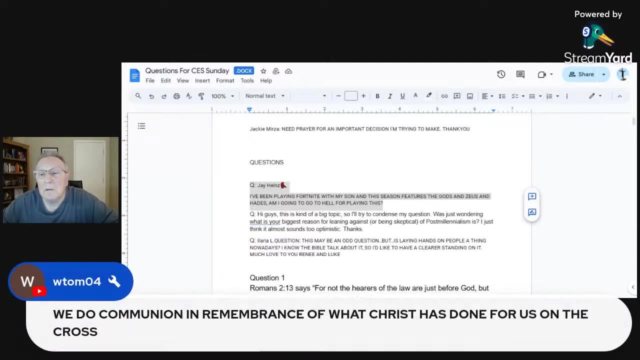 All right, thank you, Randall. Jackie says keeping in memory the blood sacrificed that Christ did for all mankind, Amen. Tom says we do communion in remembrance of what Christ has done for us on the cross. Amen, Amen, Amen. 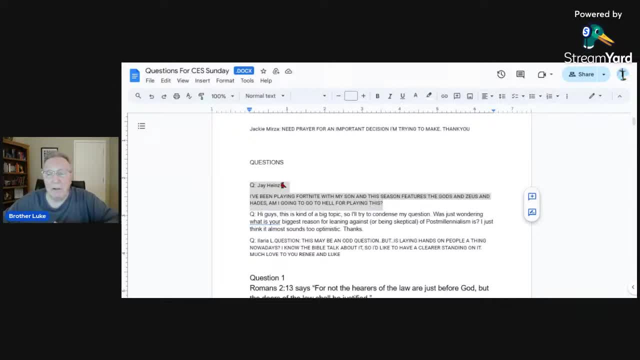 So, um, I know that many of you- maybe all of you- understand the purpose of the communion, But there are many people that actually believe and teach that communion is what saves you. That's part of the religious system in Roman Catholicism. 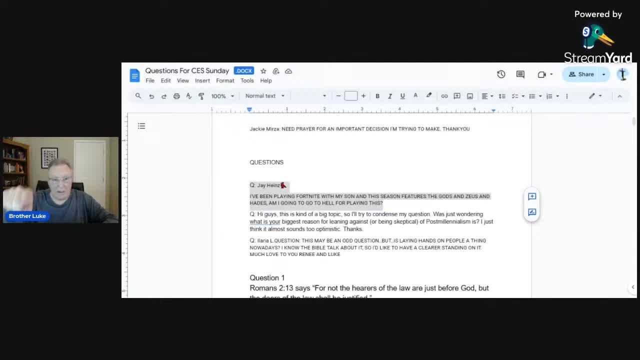 They think that salvation is like a continuous circle. Okay, Daniel 5-915.. Okay here, first step: confess your sins to the priest. Now your sins are paid for so quickly. before you sin again, go to the priest and get communion, get the sacrament. 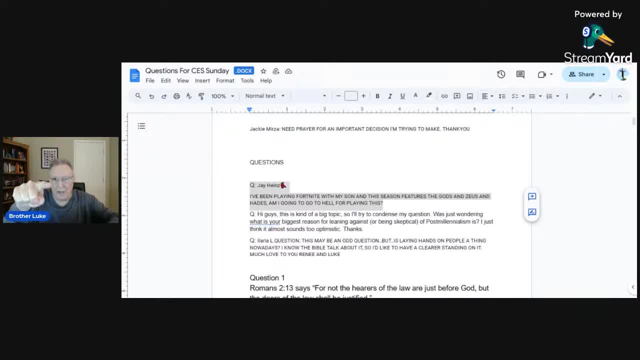 Now you've got salvation because you took communion, But next time you sin, you lost your salvation. oh no, oh no. I better go back and confess the priest again and get my sins forgiven and then take communion again, so I can. 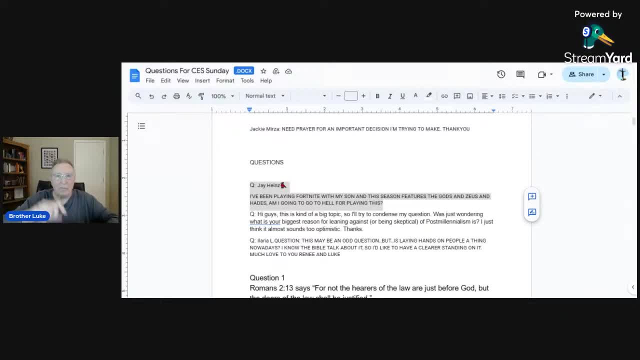 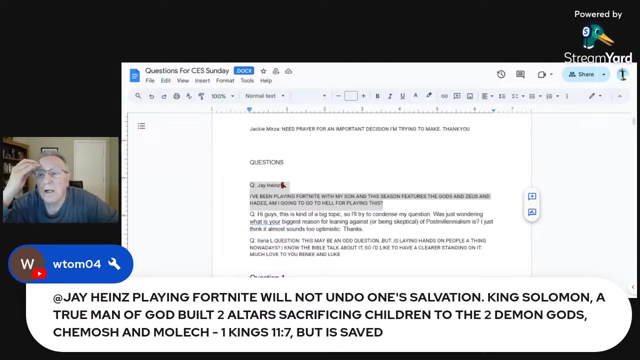 be saved again. a cycle like that. it's like she loves me, she loves me not. she loves me, she loves me not. i'm saved, i'm lost, i'm saved, i'm lost. what a horrible religion. okay, okay, um. so tom says oh, there is. tom says jay playing fortnight will not undo one's salvation. king solomon, a true man of god. 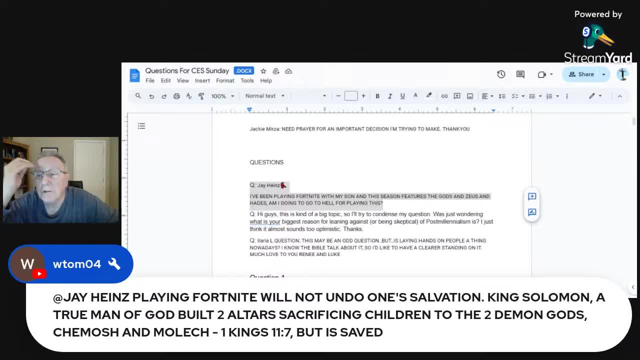 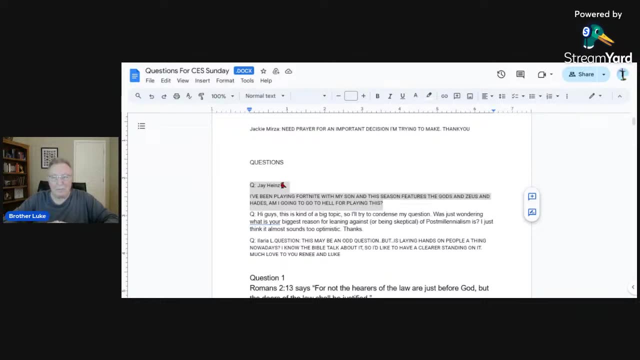 built two altars sacrificing children to the two demon gods, chemosh and moloch, but is saved. yeah, amen. uh, there are very few uh characters, prominent characters in the bible, uh, that have not done this document in the bible. they've done some horrible, sinful things, even murder, adultery, idolatry, all kinds of things, uh, and yet, uh, many of these people are. 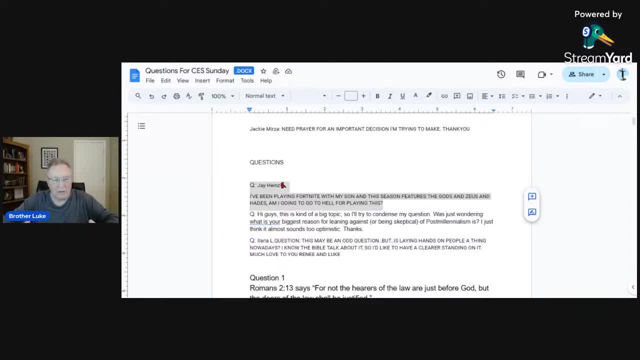 they're recognized as saints of the old testament, saved, because they trust we're trusting god. and so, yeah, that's a good example, brother tom. and uh, now, what about this game fortnight? i don't, um, i don't, i've never played it, but i i did start watching a tv series. 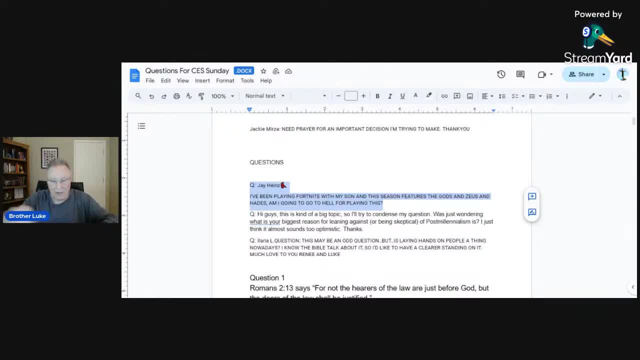 called halo and i think it's based on the game video game halo and the characters in that, and it's quite interesting sci-fi story. but these, these uh games and these virtual reality things that you can get into for for entertainment, uh is, is there anything wrong with that uh? 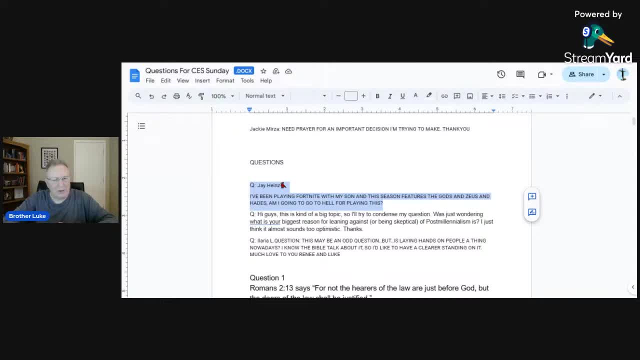 i, um, i suppose it would depend on the content. i mean, if you're murdering people and if there's all kinds of sexual explicit things that you're you're engaging in, uh, even though you're not doing it, it's your character, i, i would say that, uh, that would be sin, um, but i, i can't, i'm not. 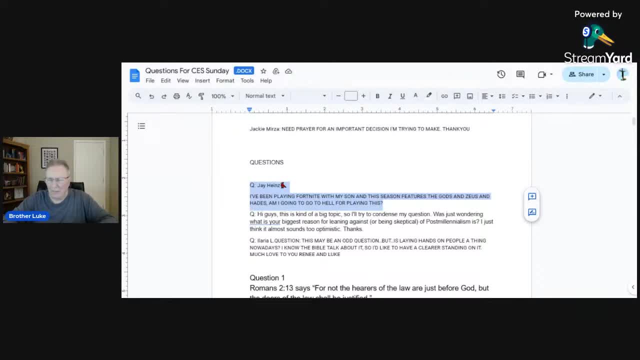 making a judgment against all games. um, and then you can even take a game like um, a game that's kind of, let's say, card game and you're not even gambling from. let's say, you're playing solitaire by yourself and you a person could say: well, is there any harm in that? 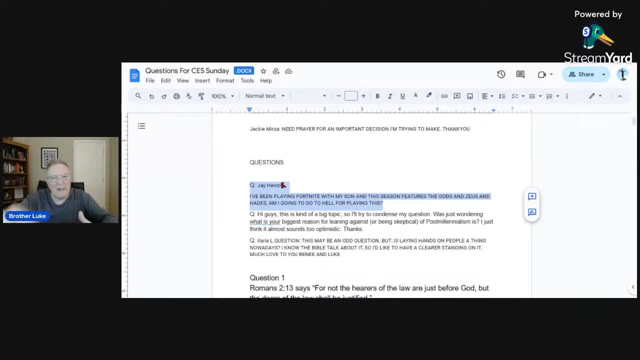 no, as long as it's done to a reasonable extent to get your mind off of things troubles and escape a little and go into a little escapism for a short time and relax. but if you're doing it too much and it's preventing you from doing other things that need to be done, then then it would be harmful. 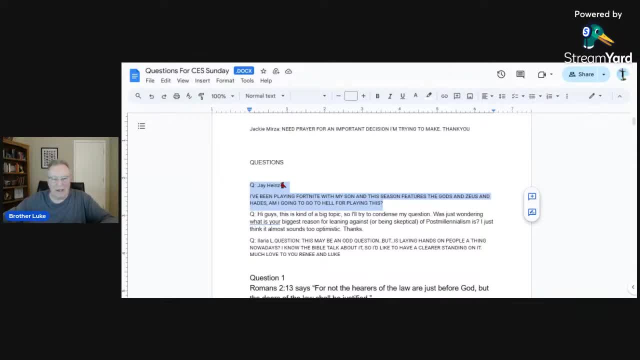 so i think that we need to have good sense, uh, and be able to discern what is um profitable and what is uh not profitable, as paul wrote that, uh, all things are lawful or permissible, but not all things are profitable or beneficial. okay, all right, jay. now as far as the gods of uh, zeus and hades, am i going to go to hell for? 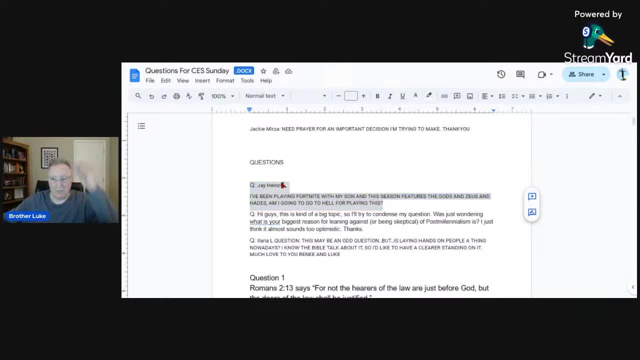 playing. yes, that's another interesting part of the question, um, because, um over this last year, i watched a lot of videos by michael heiser and by um nt wright and by uh tim from from bible project tim. uh, i'll think of his name in a minute. 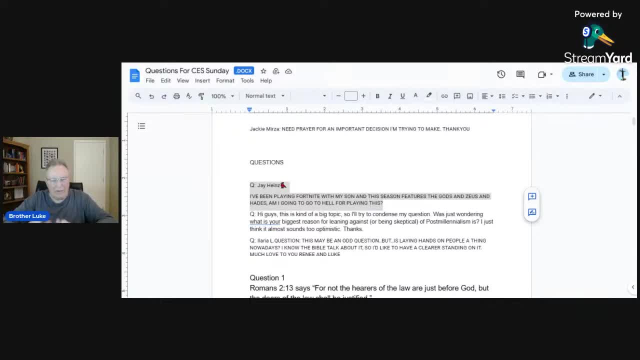 um, and they, uh, they've been talking about the idea of the, the idea of the god of the limiting palavra. they've been talking about the idea of the god of the limiting palavra and they've been talking about the idea of the god of the limiting palavra. 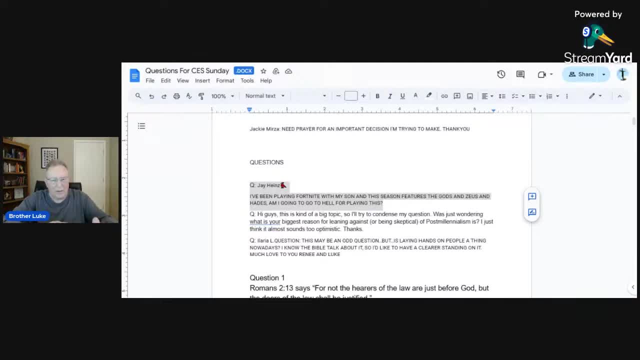 that we are monotheists in that we understand and believe that there is one true God, Almighty, one God who is eternal, who does not have a beginning, It always was and always will be, and everything else has come from that one true God, creating it. 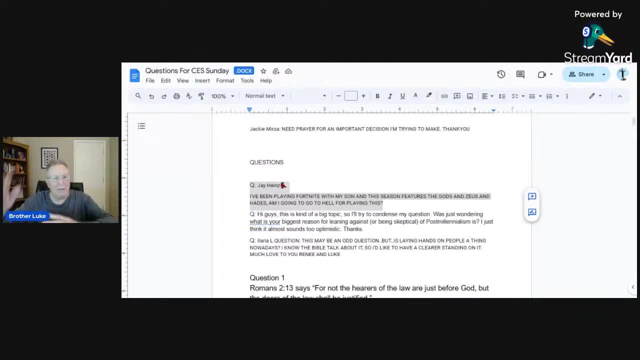 and so everything else is not eternal and cannot be. this one true God Almighty, the creator of all things, the God of gods, the Lord of lords, king of kings. That idea elevates the God of the Bible. we call him the triune God, the Father, the Son, the Holy Spirit. 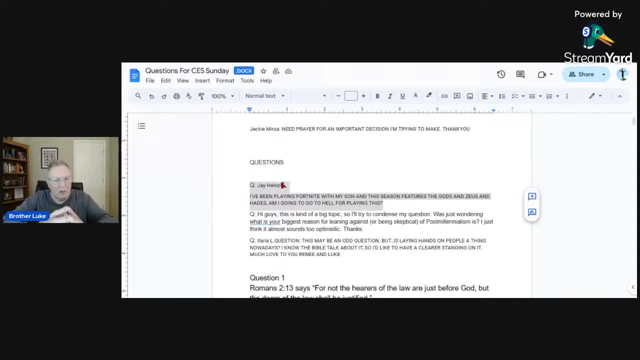 This one God is the one true God. but yet the Bible refers to many gods in the Bible. but these are gods in the sense that they are not human beings. they're created primarily to live in another realm, a non-physical other dimension that Michael Heiser calls the unseen realm. 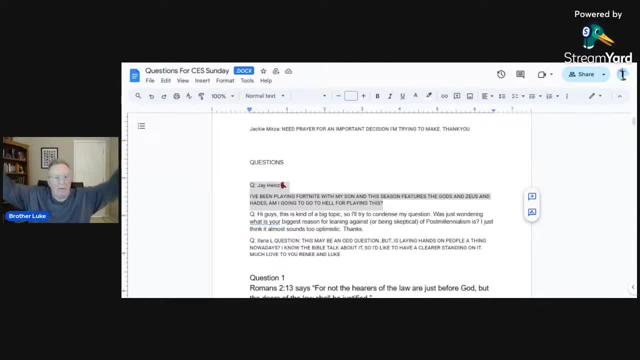 We could call it heaven or the heavens, And they can come to earth. but there's a story in the Bible about how, at a certain point, our God, the one true God Almighty, gave the whole world except for Israel, kept Israel for himself as the God of Israel, but gave the rest of the world over to these other gods. 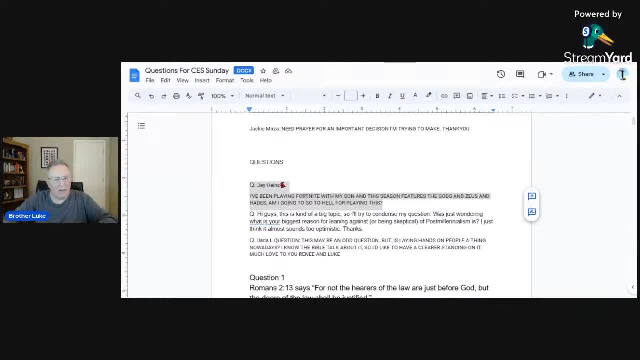 And that's where you get a lot of the mythological stories. In Greek mythology you've got Zeus and those gods associated with Greek or Roman mythology, and Neptune and Poseidon and those characters you've probably heard of. You've got Norse mythology, where you have Odin and Thor and so on. 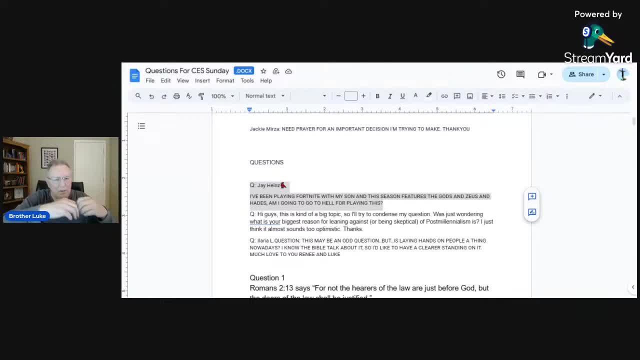 And all these different nations around the world, and the Bible says that God assigned all the rest of the world to all these other gods. But the Bible says that God had a council of gods. The sons of God is what it's called in Job, and I forgot where else. 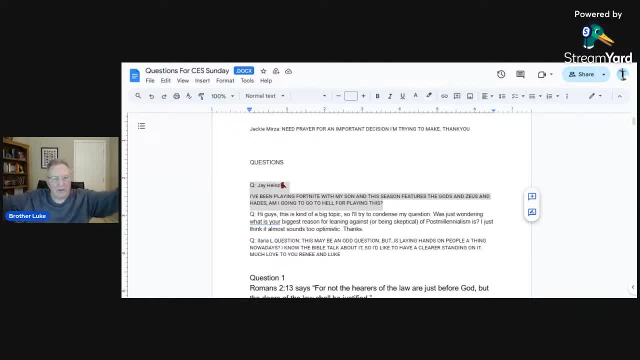 But so the world was given over, and that was. each country or part of the world had those gods that were kind of in charge. It started off as supposed to be like a delegation and delegating responsibility to these beings, And yet the people ended up worshiping them as God, as their God. 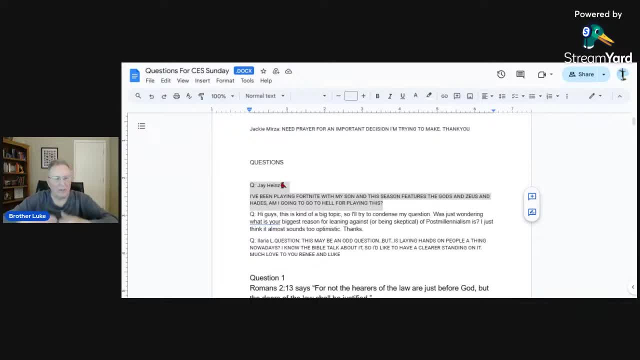 And that's when they crossed the line. when they accepted the worship, Then what they should have done was said: no, I'm not your God, You don't worship me, Don't worship me. I was placed here to be in charge for a while. 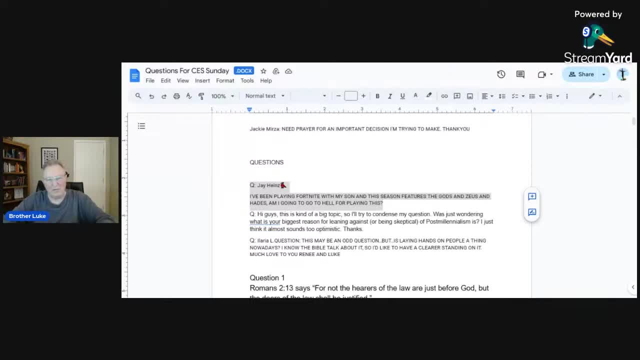 Don't worship me, I'm not worthy of worship. Worship the one true God who made me and all the other sons of God. So this is kind of my short version of the story you'll get from Michael Heiser And these other teachers I talked about that. 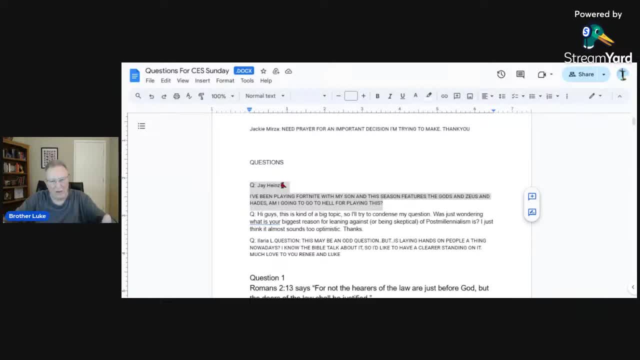 and giving the biblical account of the all these events that we find in the Bible a lot of time. I've read the Bible now for 37 years and I read a lot of these verses and just kind of skimmed over it, not realizing what it was really you know about. 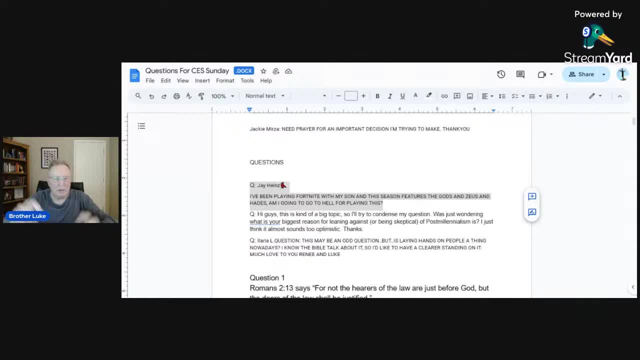 But these theologians have stopped and dug in and really dedicate a lot of time to studying this, And it turns out that, biblically, everything I just told you is supported by the scriptures. So what's going to happen is that the Lord has taken back charge of the world now. 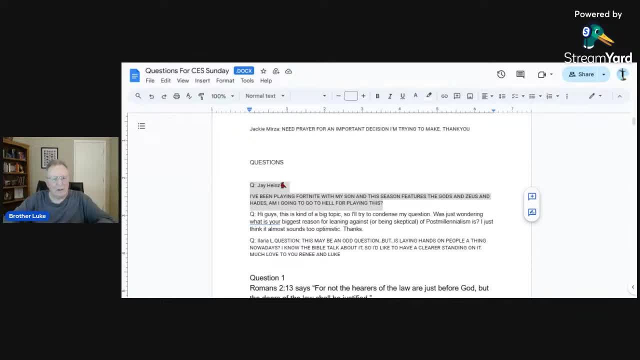 Now the whole world is. Jesus is Lord of Lords, And so God has reclaimed the whole world from all these other gods. The Bible calls them Moloch and Baal, and you know many other names. Yeah, Yeah, Yeah, The Bible calls them Moloch and Baal, and you know many other names. And so God has taken back charge of the world. So what's going to happen is that every single one of these different episodes is going to be written about the Lord in the Bible, not just through the Scripture, And the Bible calls them Moloch and Baal, and you know many other names. 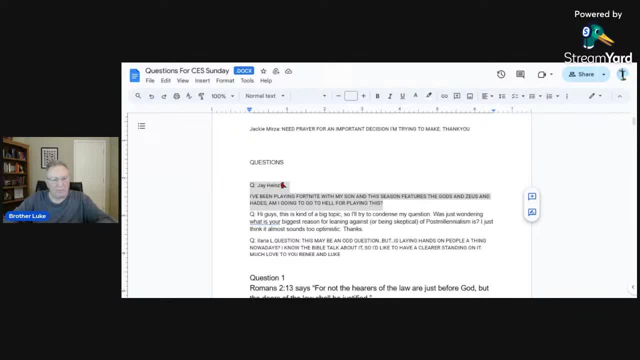 And so God has taken back charge of the world. And so God has taken back charge of the world. And they've also said all the things that we read in the Bible. those things that we read in the Bible, what those gods had to say and have said, are most clearly related to the way they saw us. 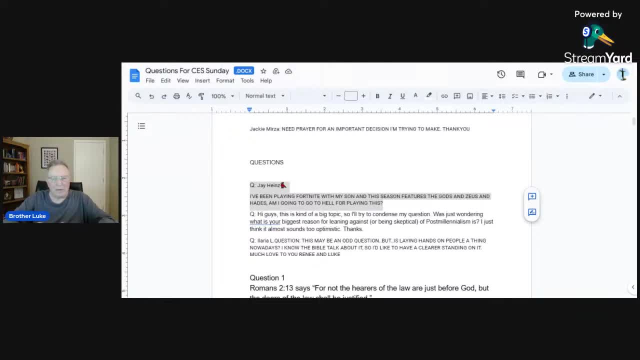 That has, that has really been the message that the Lord says that we have to be the only people to be instruments of the world you understand, And that we need to be gods now, as originally, man was delegated to be the um steward over the earth, where we are supposed to. 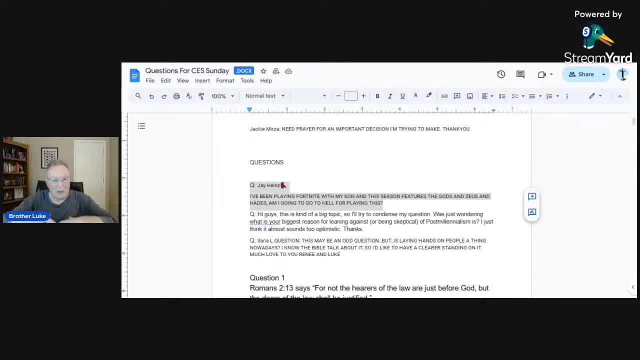 rule over all the animal kingdom and all of creation. god assigned that to man, and man failed and still continues to fail to be a good steward of the earth. but in the end, the end of the story will be that god's going to unite this heavenly realm and these, the, these beings, who, who he called the? 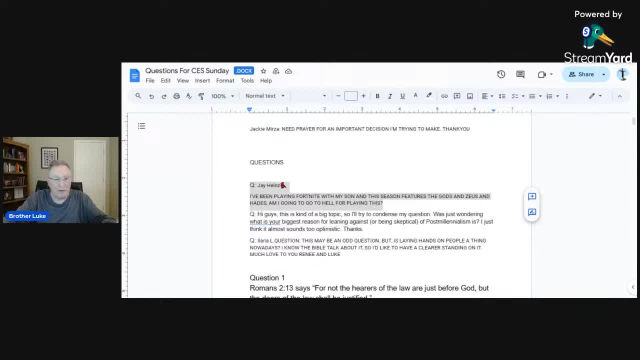 sons of god. before you and i were referred to as sons of god. so now the, the original sons of god, and the humanity that believed in jesus and became the sons of god, we will be reigns and ruling on this council for god somehow in the future. 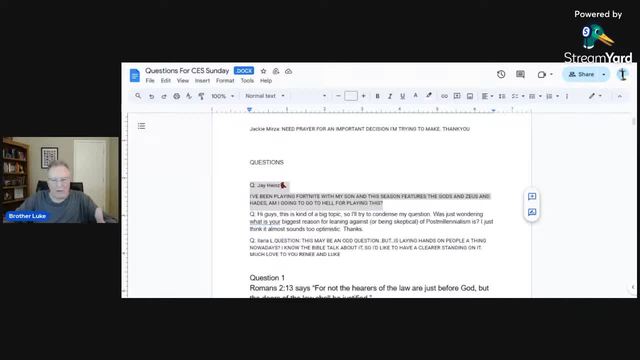 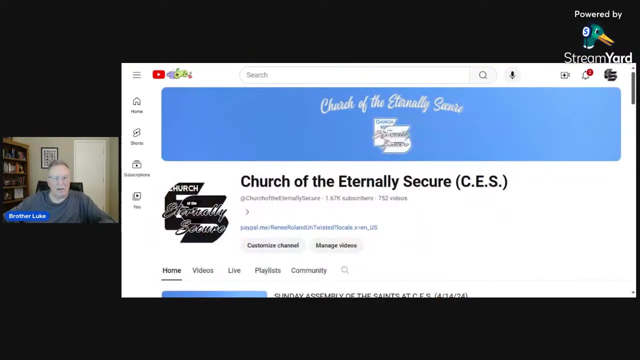 now, if this is interesting to you, then you can go to. let me see, let me look at the. this is, uh, this is the church of the eternally secure channel. uh, right here, uh, let's scroll down just a little bit and find feature channels here's. 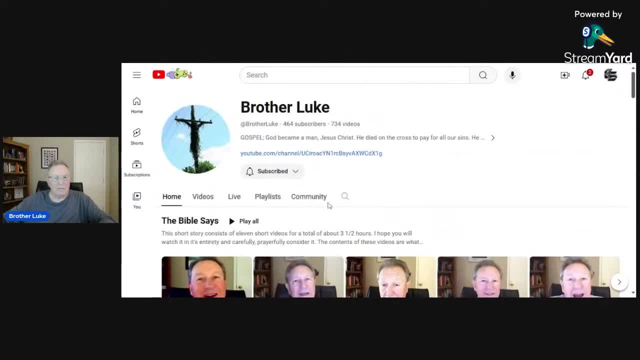 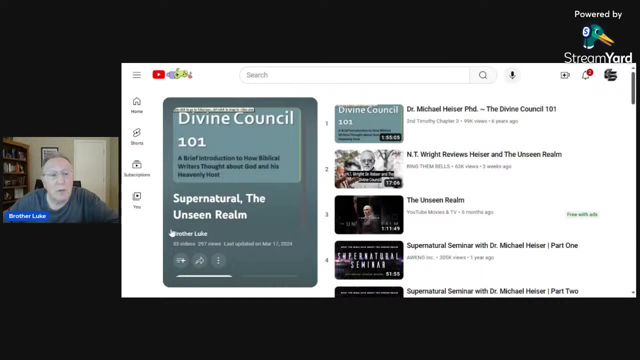 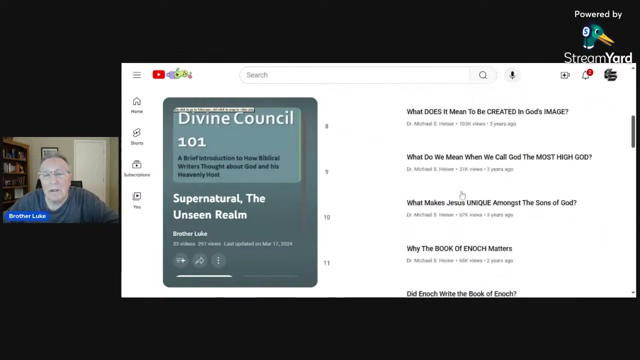 brother luke, let's look up unseen, unseen. see what that comes up with. okay, here's the view, the whole playlist. it says supernatural, the unseen realm. so here are videos by michael heiser and nt right um, i haven't put any added any of tim um, tim's uh videos, but i'm going to put them up here and i'm going to put them up here in the 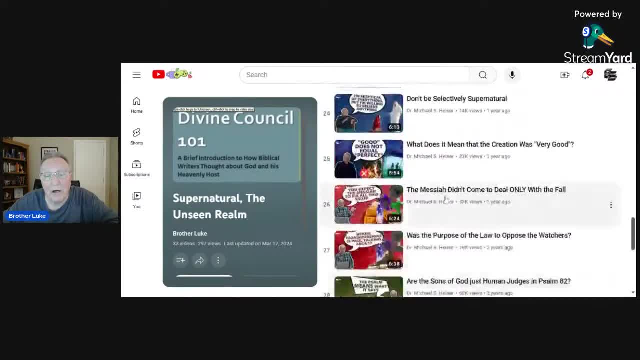 back here so you may have to watch a little bit of that. it's not like we're, like i said, a little bit of a tabla play, but there's a couple of videos to list yet. but if you go watch this playlist here it'll go into great detail, showing you in the bible everything i just gave you as 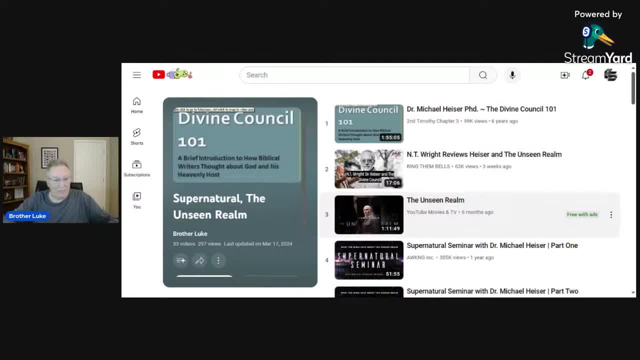 just um off the top on the head trying to tell you that story. but these videos they'll go through the bible and show you how. this is actually what the devil, the bible, tells us about this situation. okay, let me go back to that. let me go back to so that that's all related to your question, brother jay, about zeus and hades. 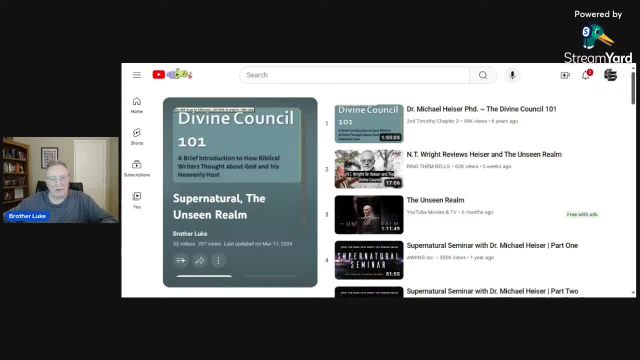 and hell and all these things it's all related to. so, uh, the gods of mythology are real, but they're not gods in the sense that, uh, they're eternal. they are. they're created beings, created by our god, the one true god. uh, and instead of uh, instead of accepting and serving god in the role that, 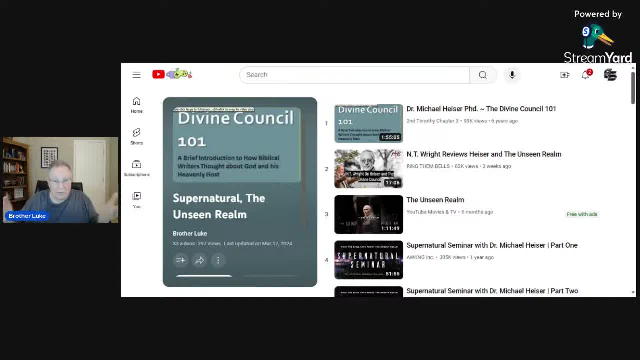 he gave them. they got puffed up like what we call the our um the adversary. the word satan means adversary, so most of the time in the bible the word satan is perceived by the word the. it should be understood as the adversary, this, uh, this son of god, this being that god created, that is, uh, not eternal because he had 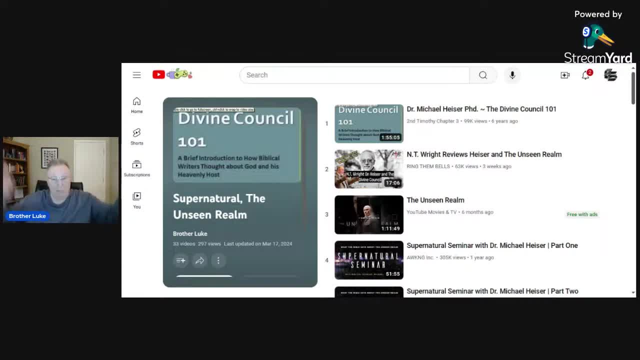 a beginning. but, uh, he thought too much of himself and wanted to be in charge. and uh, that's what happened with all these other gods too. they, they, side with him and decided that they were worthy of worship. okay, jay, uh, let me look at the chat room and see if 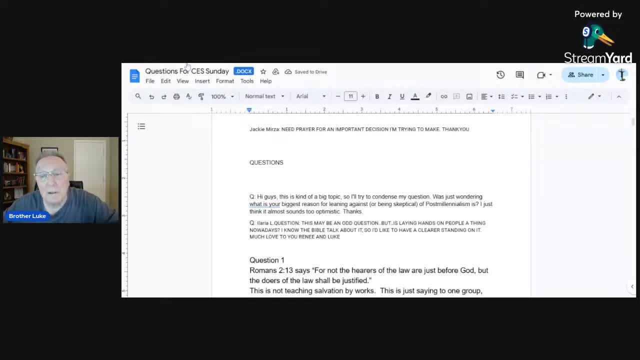 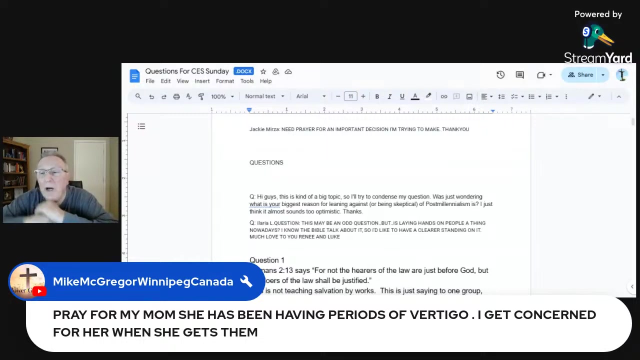 see if anybody is uh interested in what you're saying. okay, okay, here's uh. mike says pray for. she prayed for mom. she has been having periods of vertigo. i get concerned for her when she gets them. i'm not sure if she's going to be able to get them. i'm not sure if she's going to be able to get. 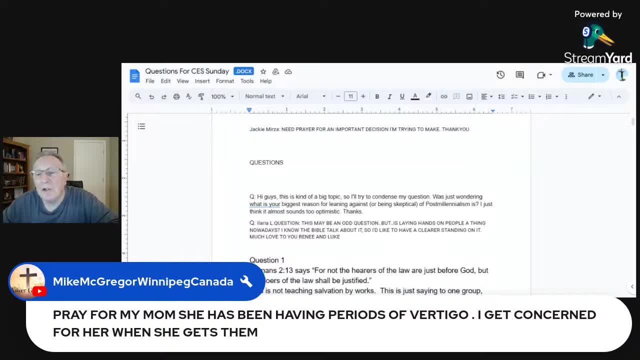 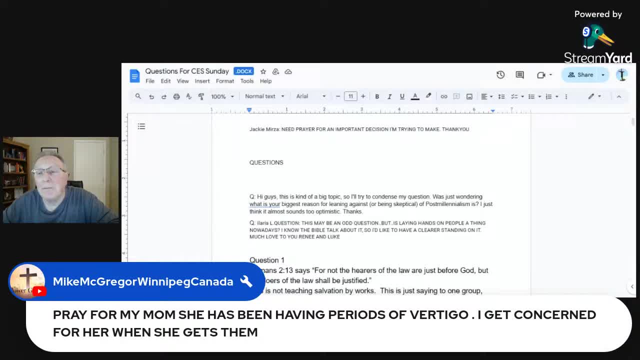 or are you talking about sister shelley, who we? or are you talking about sister shelley, who we know, as mom know, as mom know, as mom, mom, it doesn't matter whoever this is, that mom, it doesn't matter whoever this is, that mom, it doesn't matter whoever this is, that mike's referring to us. let's pray for them. 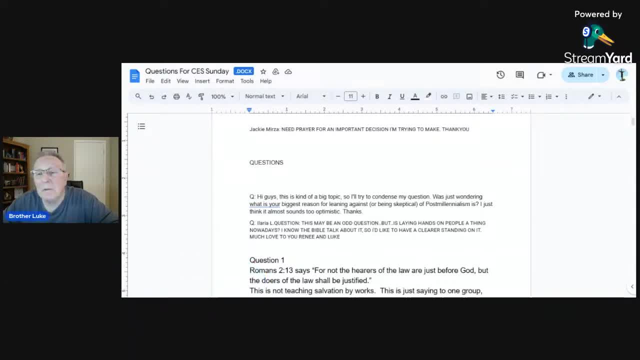 mike's referring to us, let's pray for them. mike's referring to us, let's pray for them. and their vertigo. okay, yeah, um brother thomas says brother luke. i yeah, um brother thomas says brother luke. i yeah, um, brother thomas says brother luke. i have heard that. 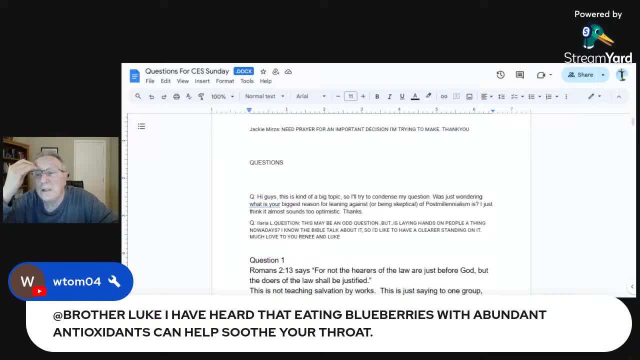 eating blueberries with abundant antioxidants can help soothe your throat. thank you, brother. i i do. i eat blueberries every day. it's part of my regular diet. so some of the foods that i eat each day, um, i've chosen to put it in my daily diet one. i do enjoy them, i like to eat them, but they're 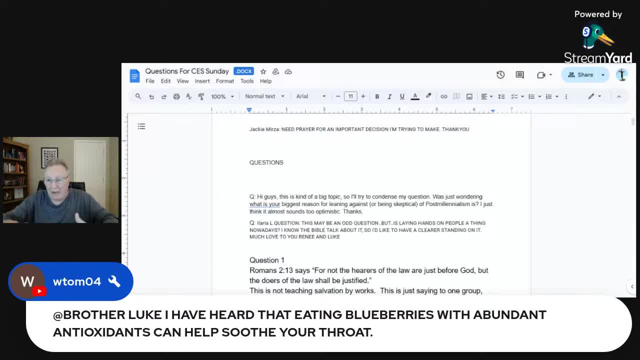 selected, kind of like you would select a medicine. they have qualities like the one you're telling me about here. tom, with the blueberries- a lot of really good benefits from eating blueberries. so blueberries and some other things i've added to my diet and i look at it as almost 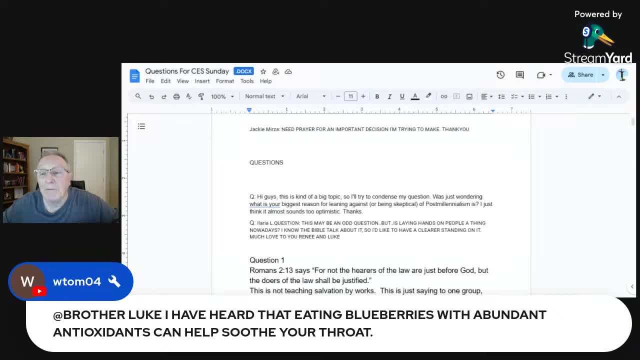 like taking my medicine, but it's done through diet and food. but obviously, regardless of what we do, regardless of our diet, our exercise, uh, our- some people have really better genetics where they're less inclined to be sick. all these things are factors, but you can't cheat death and time eventually given enough time. 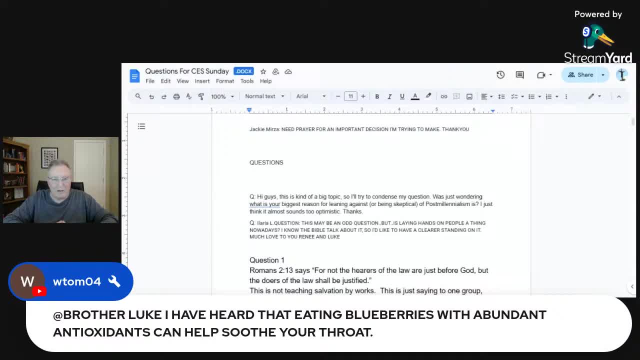 your body will fail. so we can try to improve it by quality of our life, so we feel better and have more energy and and uh, and we can try to extend our lives. but it's a losing battle but thankfully we are promised resurrection and life everlasting. okay. 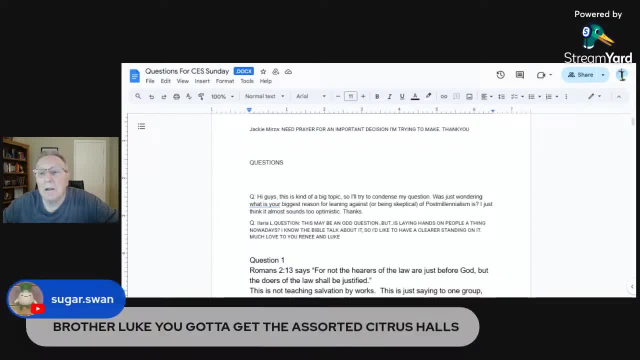 okay. and sugars, one is recommending, uh um, assorted citrus halls. yeah, okay, maybe i'll get those, if i, if, if this doesn't clear up right away, i'll run out. i'll have to get some more. i'll have to get some more. i'll have to get some more. 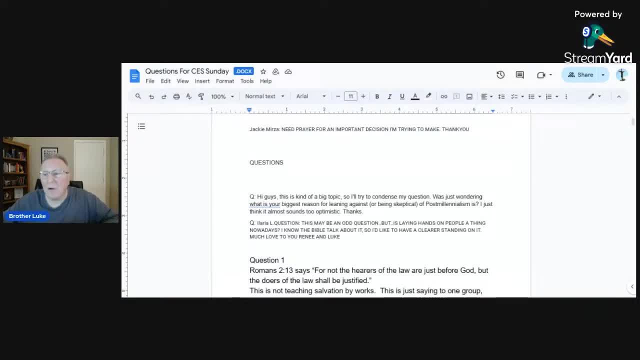 all right, okay, let me go to. i don't see another question in the chat room. let me bring up something i'd like to want to talk about. we we talk about, uh, hermeneutics, sometimes hermeneutics. now, a lot of you probably know what that means, but some of you may be new. 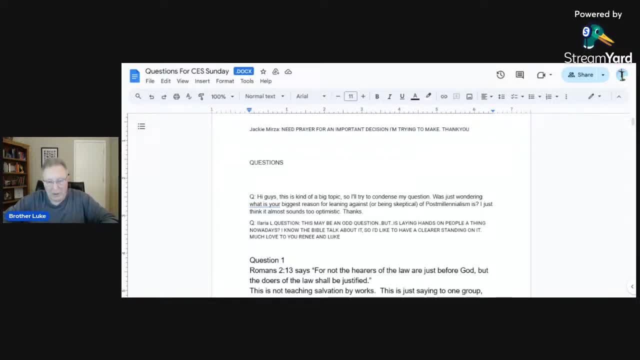 just beginners studying by the bible and theology. hermeneutics simply means it's, uh, your method of studying the bible and trying to understand the bible. what approach are you taking to try to understand what it's telling you? that's hermeneutics, and there are certain principles. 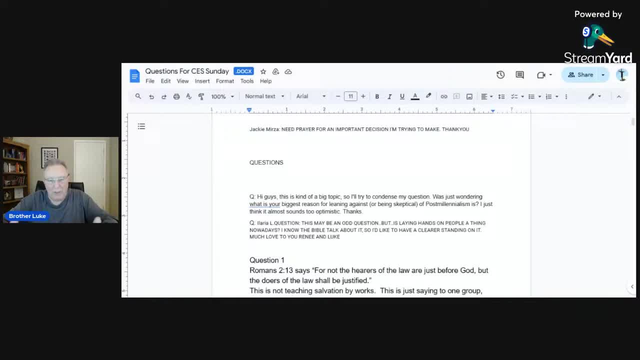 in hermeneutics and that should be applied. not everybody agrees on which approach is best, but one. one thing that is i think is important is i used to call it the universal or particular application, but another way i just heard is the descriptive or prescriptive. 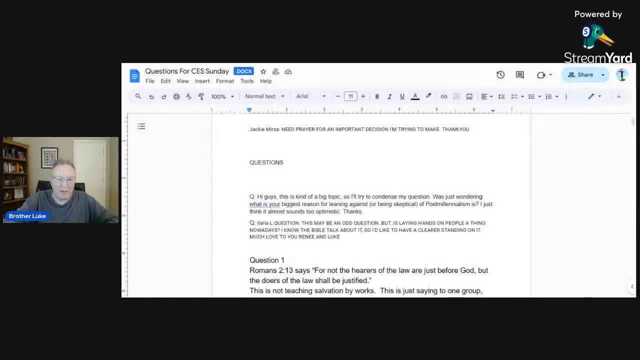 in other words, is the verse there in order to describe the situation that's going on? is it a particular way? or is it a particular way? or is it the necessary way to describe a situation? or is it the certain way so we can understand the scenario? or is it there prescribing for future generations a, a a way of doing things? 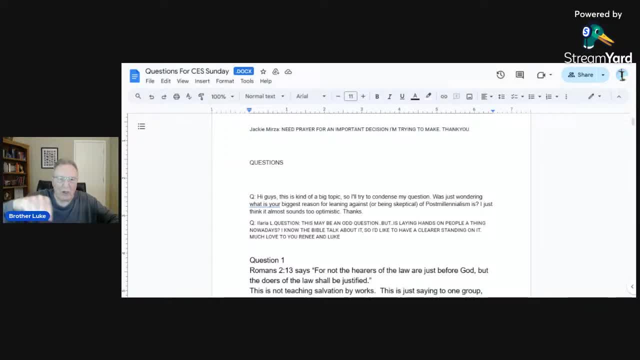 or was it? is it particular for that particular route because they had a particular person or a group of people who were created, a specific problem that required a particular prescription, or should it be applied universally to all churches, all people of all times? so that's something you have to keep in mind as you're studying each of the verses. 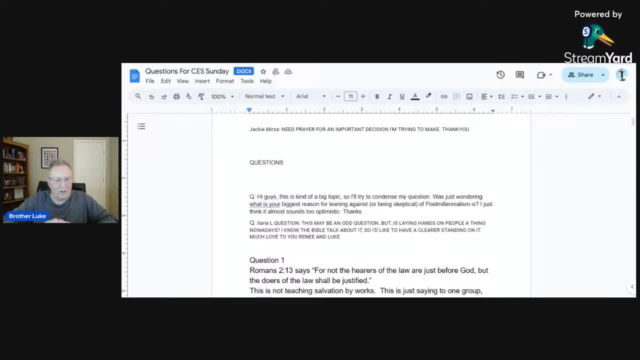 for example, the, the verses that we've talked about when we're discussing the subject of women in the church. what's the proper role of women in the church? should they be held down and not allowed to reach any level of responsibility, authority, or like teaching and preaching, and 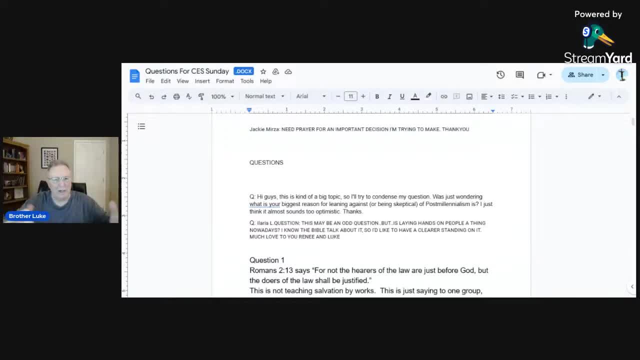 leadership or or are they truly equal with the men and and and there's no barriers to help what they're allowed to do in serving much of the church, have taken the idea that there's a a subordinate role that women must maintain. it can't ever be equal with the men. 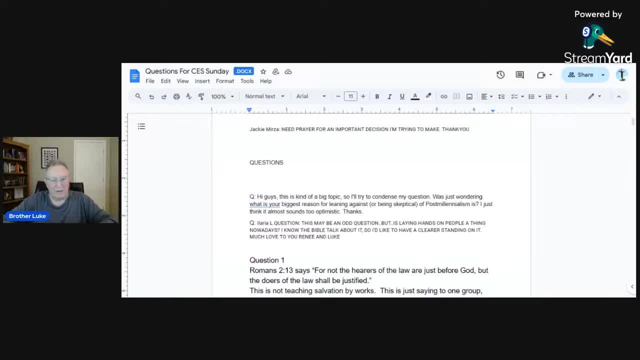 and some of that it comes from some of the things paul wrote in. i think it's first corinthians, chapter 11, i think, and first and second timothy, where he's talking about women are not, are prohibited to teach, and women must keep silent, and so on, if you want to. 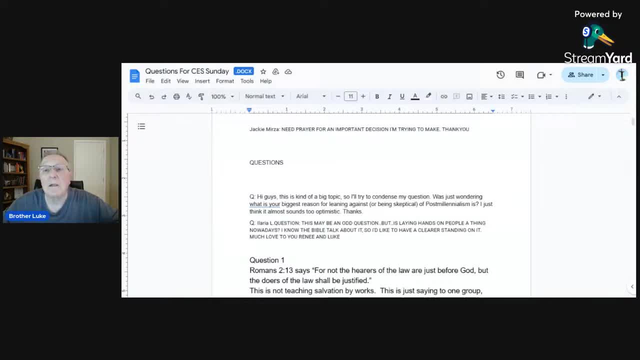 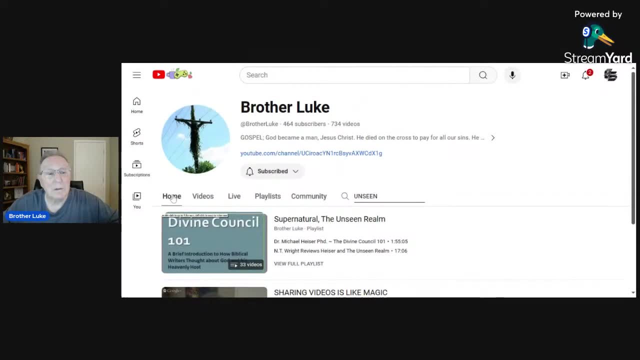 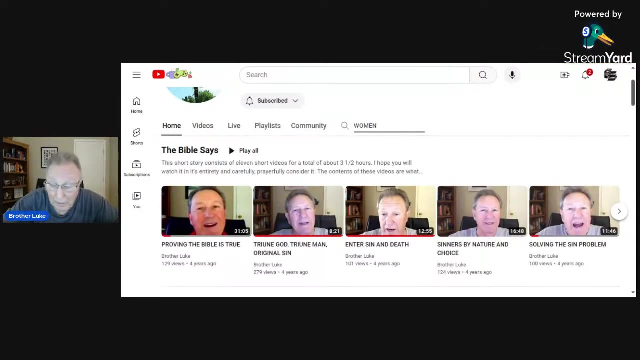 know about that subject. let's go back to this again. okay, this uh to the brother luke channel time and let's look up women, women- okay, women's role in the church. here's the playlist. if you go through here and look at all the videos, there's 14 videos on this. 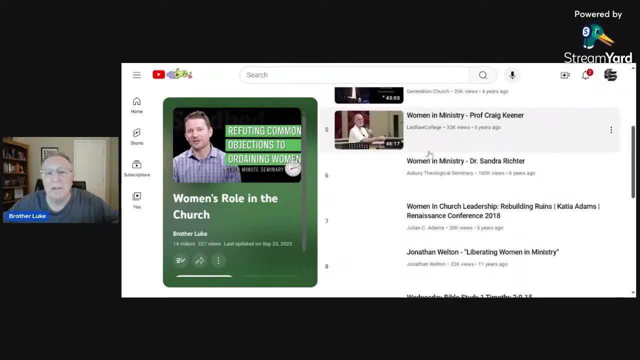 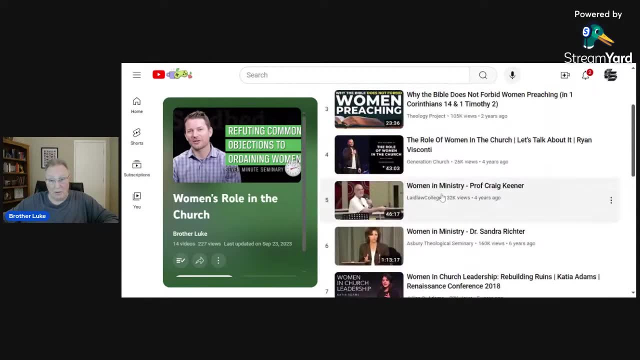 playlist: some really, really excellent teachers, including renee, and i have done some videos on this subject too. you've heard us talk about a lot over the last few years, of course, because we've had to defend it. in fact, we had to denounce resh впalere when weka had added that to the badge ofos. 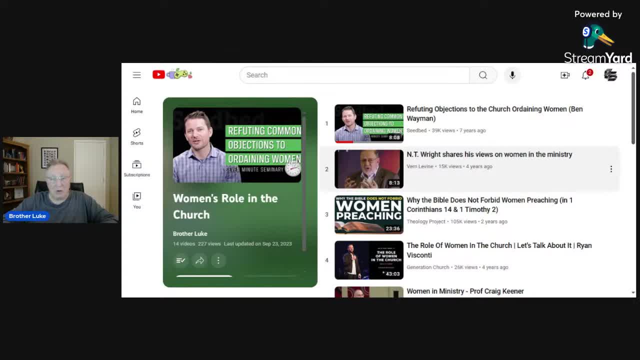 of course, because we've had to defend Renee's role in our church and there are people who don't approve of it. But I think if you watch these videos you'll understand that some of these verses should not be understood to apply to all women all places, at all times in church. 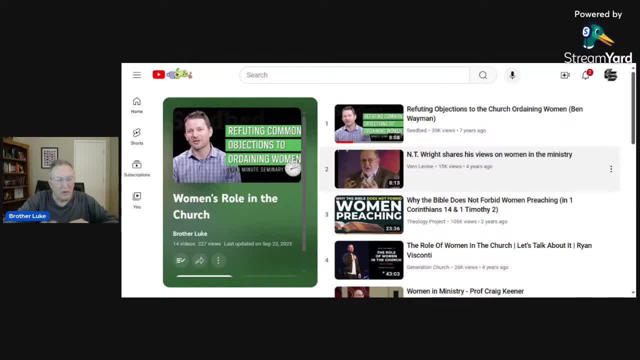 history, It should have been understood to deal with a particular woman, a group of women in a particular time in history, where the culture was a certain way and the women were not allowed to be educated beyond a certain point. All those things have to be kept in the context. 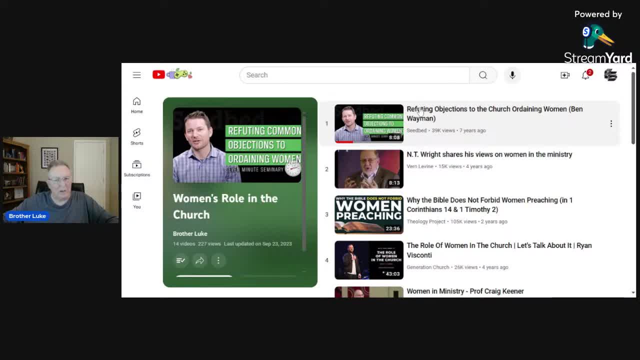 So if you're unfamiliar with this question, then I suggest you go to that playlist. Let me look. I'm going to try another shot of this cough medicine. There's no codeine in it. I would maybe be better off if there was some codeine, but 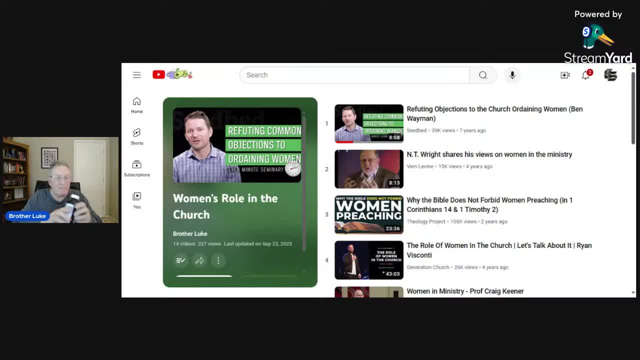 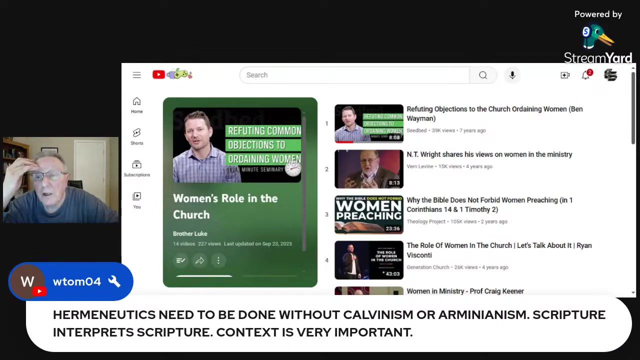 I don't need a spoon, It's just me, so you don't want to be affected by it. All right, Okay. Okay, Here's. Tom says hermeneutics need to be done with a script, without Calvinism or Arminianism. Scripture interprets scripture. Context is very important. 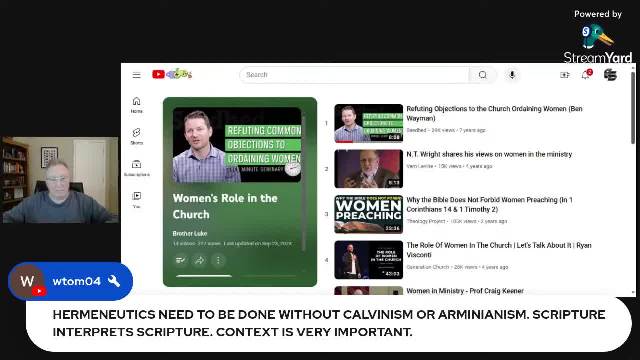 Yeah, Amen, Most people, unless you're a complete novice and you have no preconceived ideas- a set of pre-assumptions, suppositions, assumptions that you're bringing with you- well, let's call it baggage. You're bringing your baggage in when you read the Bible. 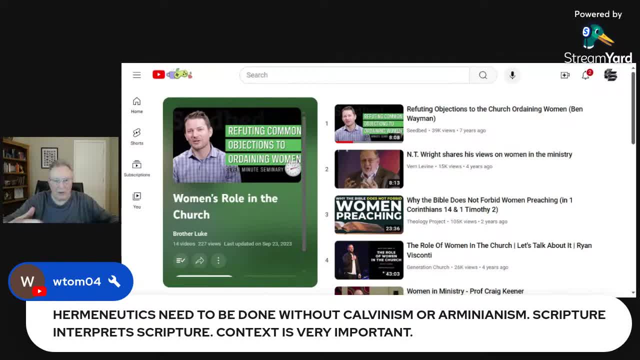 and you're using this as a means of understanding the Bible, the baggage you bring in. Well, that's wrong, because you can come to completely horrible conclusions, because you're looking at through the lens of your own experiences or your own prejudices. So one, of course, is to 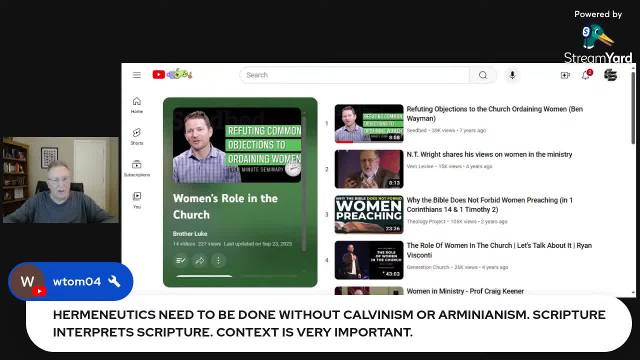 look at the context. but I'll tell you, context is much more than just okay. what does John 3.16 mean? Well, maybe we ought to look at John 3.15 and 3.17, too. Well, of course, that's expanding the. 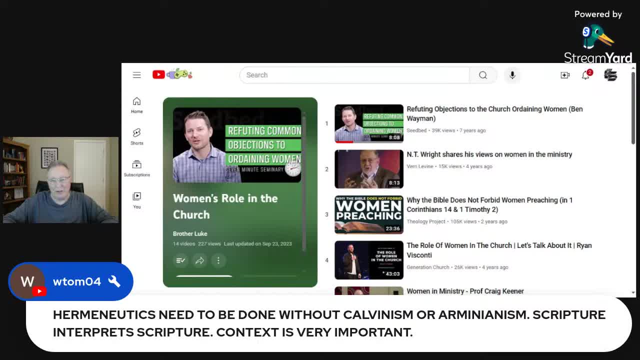 context, but that's not expanding it very much. We need to look at the context of the entire conversation. Maybe there's five or 10 or 20 verses that are all relevant to this particular context. Maybe there's five or 10 or 20 verses that are all relevant to this particular context. 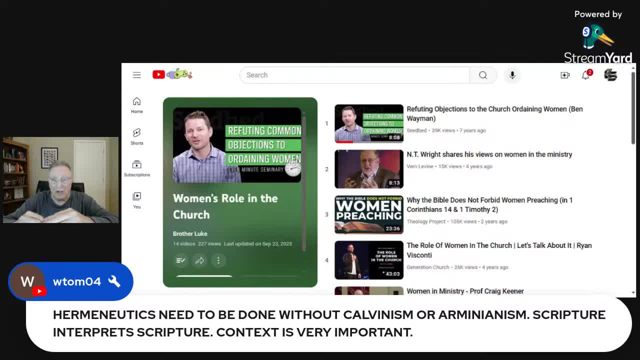 conversation. Then we also have to keep in mind the context of who wrote the book and what purpose was it and what's the main theme that they're trying to convey. And then we have to also understand the context of how that book fits in with the overall story of the Bible. All these 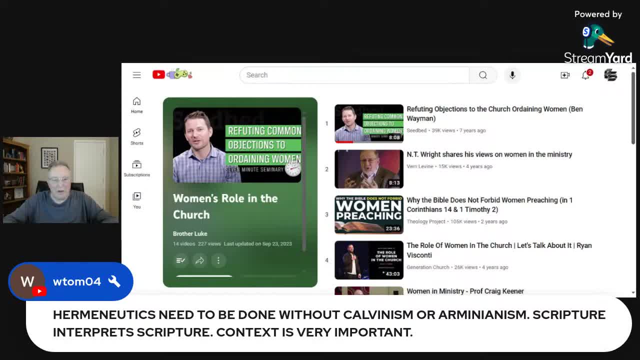 things are part of context. For example, I believe one of the biggest failures in context is people will apply context up to a certain point, but they forget that there is a particular God of the Bible, God Almighty, And there are a lot of really clear, specific details that were given. 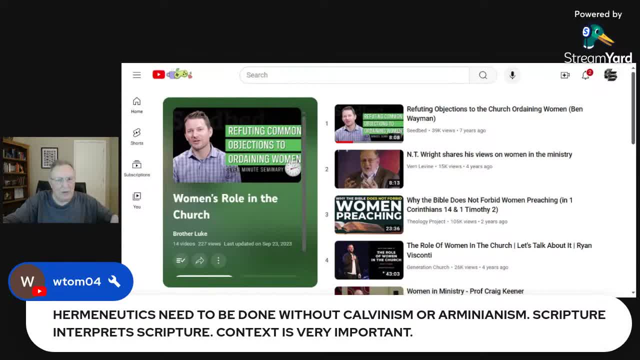 about our God attributes, qualities, characteristics, about our God attributes, characteristics. But it's also quite distinct, in a way. There are a lot of really clear, visible clues. I had, uhh, a bunch of symbolic سミuri. 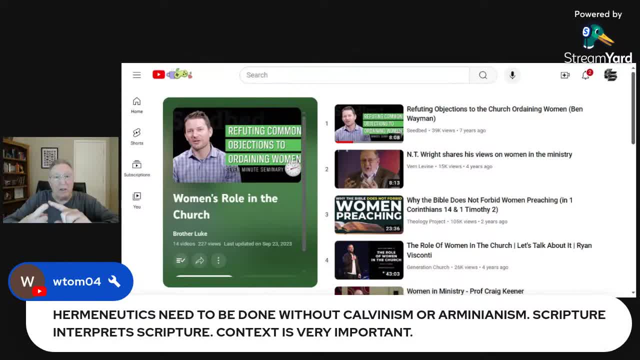 my, I had, uhh, a bunch of symbolic سミورية that each of the Bibles we seem to see in context, which makes us wonder: can we find them? There's all sorts and we've handfuls of thesegie that have similar знак: ballons with number th usually. 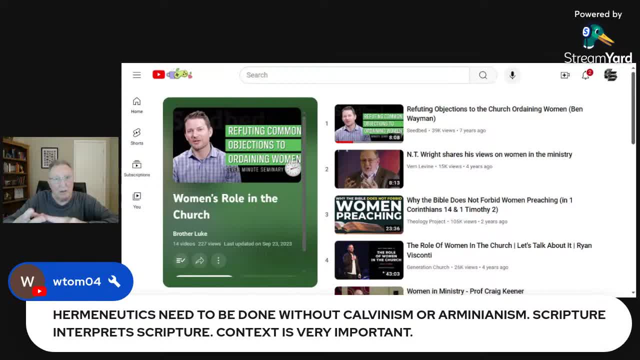 In times of någon tv wisdom that are written down. what were the main factors? wen 소개? Michael's message from people voice says is: the God of the Bible is love. The God of the Bible is just. The God of the Bible is merciful. 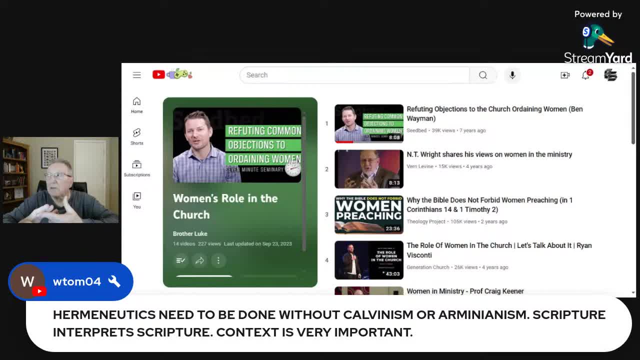 The God of the Bible is omniscient, omnipresent, omnipresent, omnipresent is Omnipresent. God exists and has manifestedase for any object or nature, And if you are one of them, omnipotent and omnipotent, omnipresent, and what's the other one? omnipotent, omniscient. 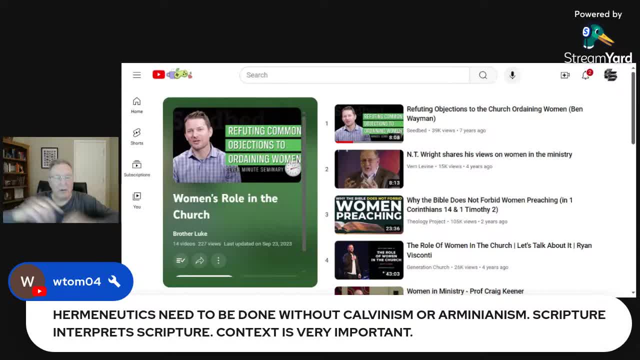 and omnipresence. yeah, those are the three, but the point in making is that, uh, the bible, when we study the bible, we learn the bot. the bot, our god has certain attributes and if we understand that, one of the attributes, for example, is: the bible says that god is honest and god 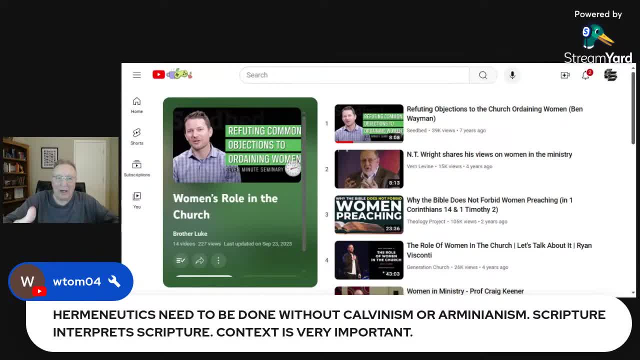 cannot lie. okay. so if you, if you have a verse in the bible that says that says, say god's lying, you know that god cannot lie. therefore, that verse cannot mean what you're saying. it means it must mean something else. let's dig into the context around it and find out exactly what that's. 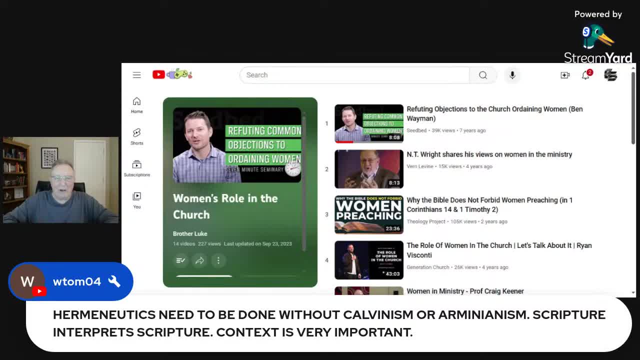 talking about. you know, um, if we say that the god of the bible is just and then we someone says: well, what about this god's god's very unjust because of this? well, no, it doesn't change that god's now he's unjust. it just means you don't understand those verses properly, and i think this applies a lot when it 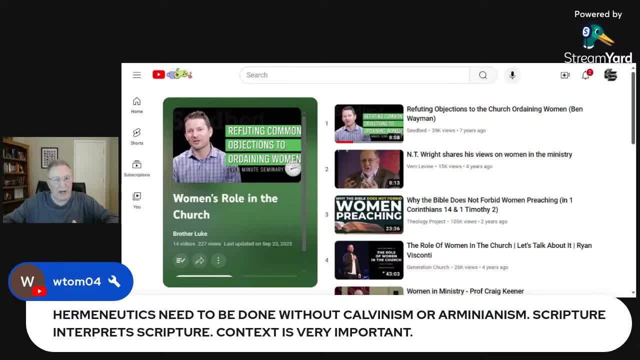 comes to the problems with calvinism, that that god of calvinism is not the god of the bible, and i believe it also applies to the, the doctrine of eternal conscious torment, that god is not loving, merciful and just clearly punishing people for things that he made them do, because they don't even have free will. he makes 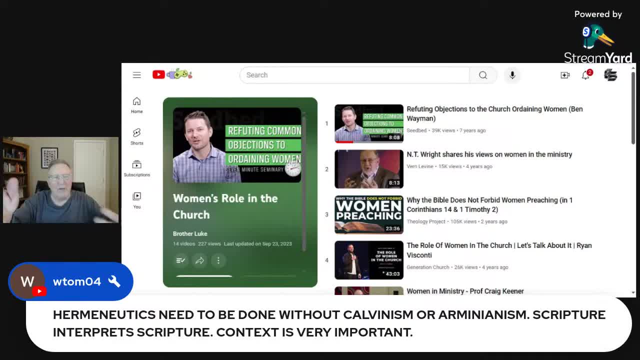 them do the most horrible things, all the most horrible things that have ever been done, that you've done, i've done, and hitler and jeffrey dahmer and all the worst people in the world. all those horrible things god made them do it. they didn't have a choice. god made them commit all those. 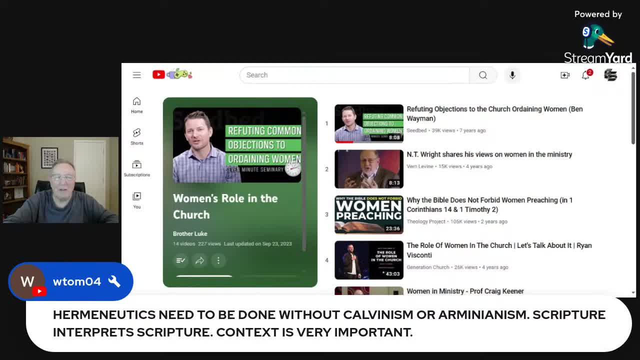 atrocities and then he's going to find them guilty and punish them for what he made them. do you see? that does not make sense. if the god of the bible is just, is it so? uh, the context to me. one mistake is we. we need to remember that context is so broad, it even goes to the 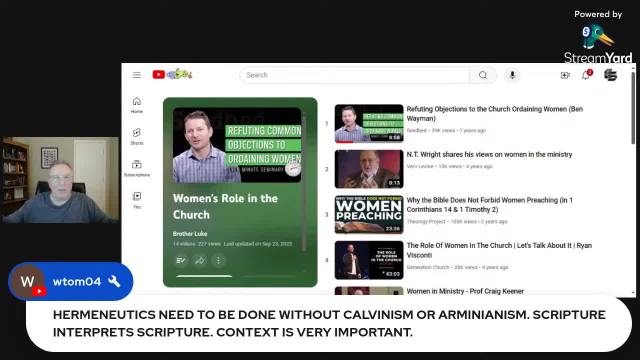 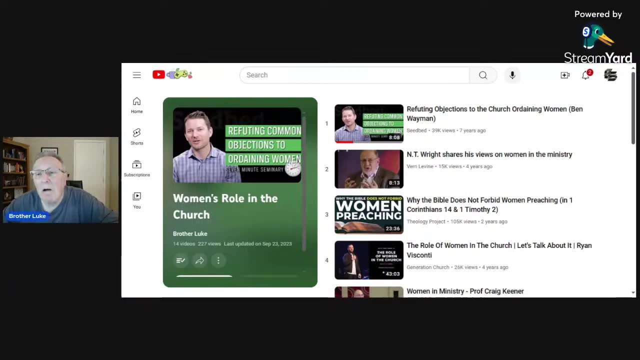 description of who is the god of the bible, because we cannot interpret the bible the way that it turns our god into some evil monster. okay, let me see i'm not seeing any other questions. oh, all right, let's try. look at something else. you know a lot of people are uh. 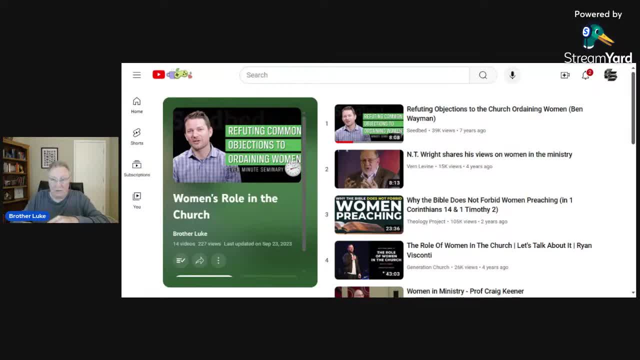 um, some of you here right now have some kind of pain issue. i've learned to live with chronic pain for many, many years now. i've had surgeries and medications and all kinds of things to try to deal with my pain and it helps to a certain extent, but i'm always in pain and but, on the other hand, 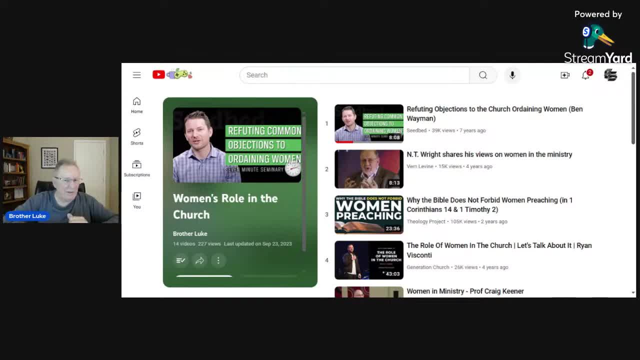 um, what if there was no pain? if there was no pain, we, we might wonder: how could god be a good god? look at all the pain and suffering that people have. well, there's some kind of suffering and pain. uh is very, very important. for example, if you, um, if you stepped on a nail. 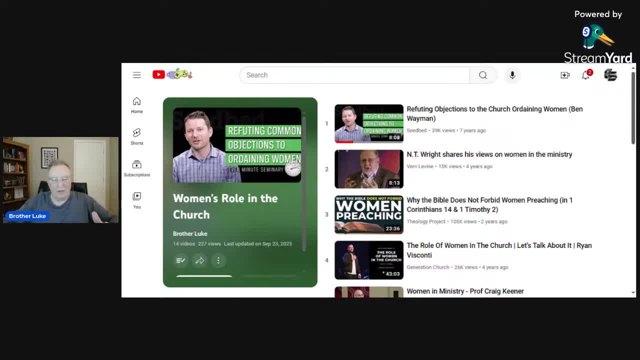 and it hurt. that pain tells: oh, pull my foot away. and now you know the pain is causing you to say, oh, no, there's an injury and you have to deal with it. if you, if, if you had no pain, you wouldn't be aware that you are damaged and something's wrong, and whether it's physical pain or even, uh, pain, 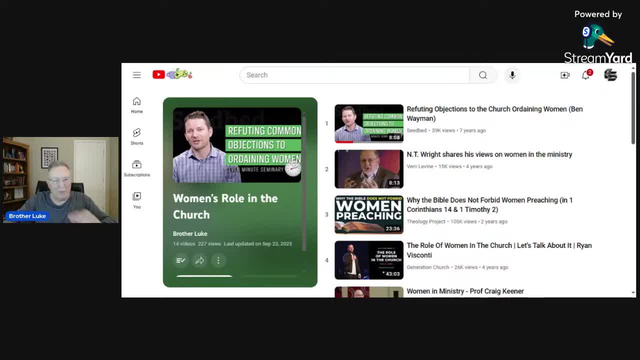 between people in relationships, some kind of emotional or pain, that's um non-physical pain. these things are there to to make us pause and stop what we're doing, because what we're doing hurts. maybe we should all stop and ask ourselves about the pain we're we're dealing with and uh, 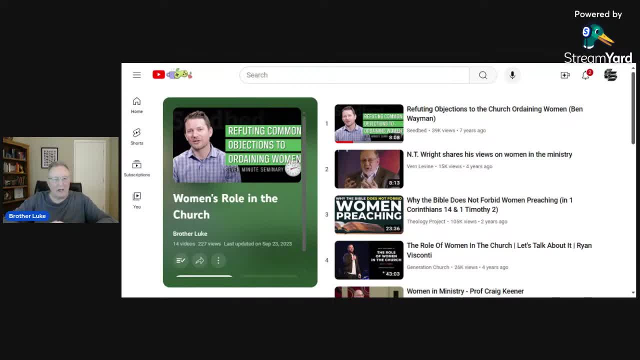 instead of being angry about it, i realize that wait a second. there's a lot that we've spent day to day. it wait a second. the pain tells me something's wrong. maybe maybe I can fix it by changing my diet. maybe I can fix it by by doing particular exercises. maybe there's a surgeon that has the 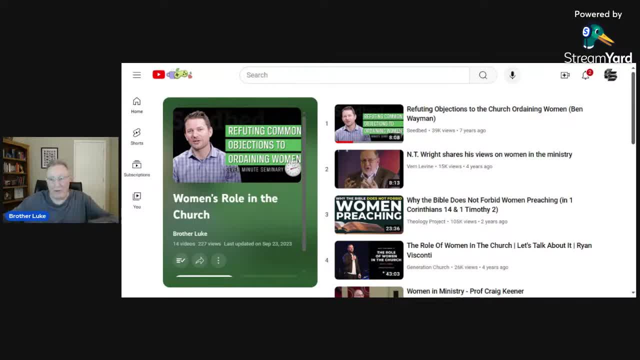 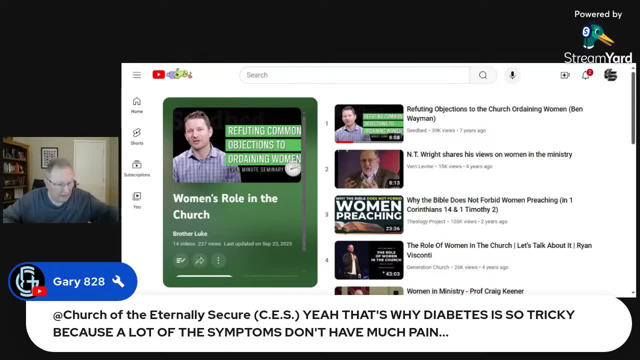 fix for this, but the pain tells me there's a problem needs to be dealt with. Gary do says: yeah, that's why diabetes is so tricky, because a lot of the symptoms don't have much pain. oh yeah, that's everybody is aware. if you've been with the CES very long, you know that I lost my beloved. 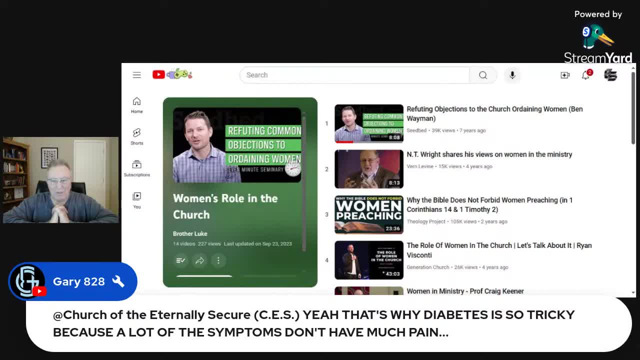 wonderful wife Cindy. last year has been ten months, you know ten months ago, and if she had pain from her cancer she had bladder cancer. by the time there was an indication that there was something wrong and it was just a slight bleeding. a little bit of blood told us something wrong and we got it checked and found out there's a problem. but if 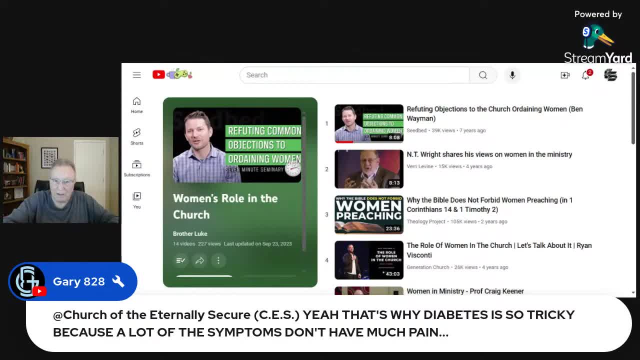 she had blood earlier, much earlier, or pain associated with it, maybe a year or two years earlier, because this had to be a problem for a long time, because by the time we found out that there's a serious problem here, it had advanced so far. it was horrible, it was. 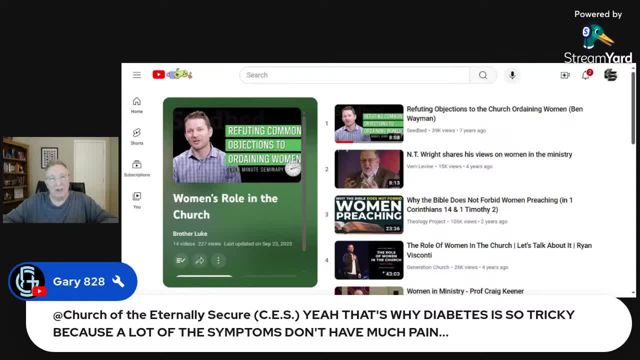 it cost her her life. but if she had been caused, if it caused pain a couple years earlier and we could have been able to fix it, if it was small, what probably would have been fixed quite easily. and that's true, I guess, with diabetes. I don't know that much. I mean, I know people who have diabetes. 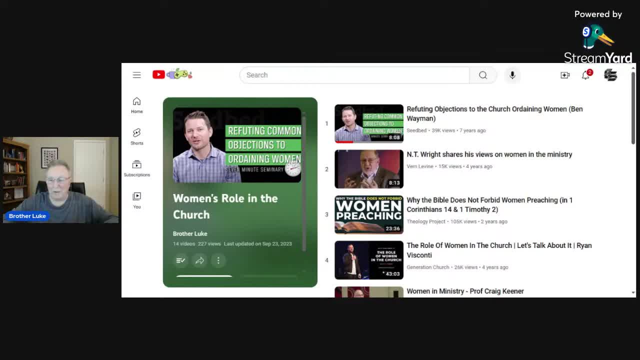 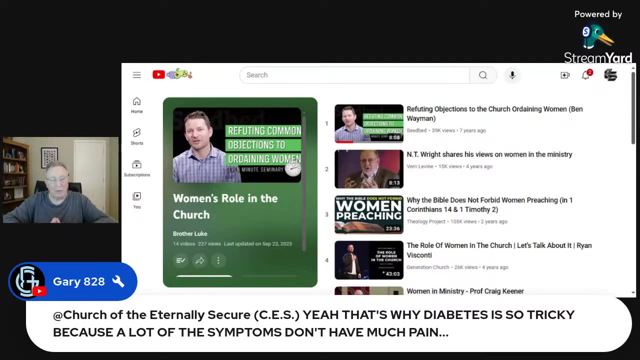 I know people who've lost appendages from diabetes. uh, I don't know what all the symptoms are, Gary, but um, yeah, so sometimes you have to be thankful there's pain. I I just wish there was some pain. that has warned us about my wife's illness. 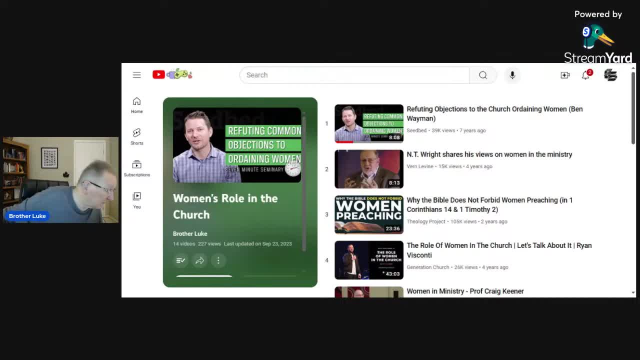 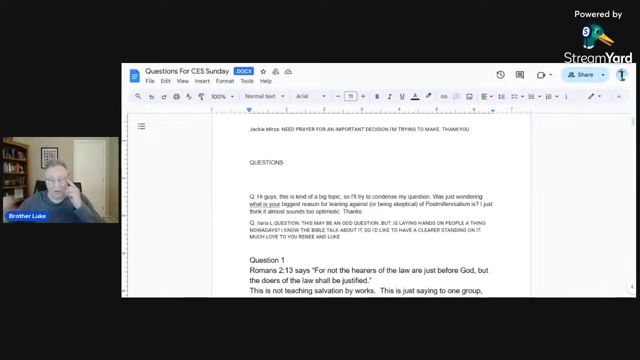 let me see. all right, um, here's an interesting um point, that uh, interesting point that I learned recently from one of the Bible teachers I listened to. um, we know that, um, in the garden of Gethsemane there was a test for for Jesus, and we should will. he go on, or the agony he suffered in the garden. it was so hard for him ate. he did take a look at his life, the things the bible teaches us about what he was shouting, and it's that. It just sciences, and it looks bad to me especially and the schizophrenic just talks bad about. it's just. But you're seeing pain in the people. his mom hacked him into the wall right and there's nothing but pain in his mouth- and about the pain in their cosmic. simone, obviously joy becomes ok. we, We know that, uh, in the garden of Gethsemane there was a test for it for Jesus, uh, and we, when should? will he go on? 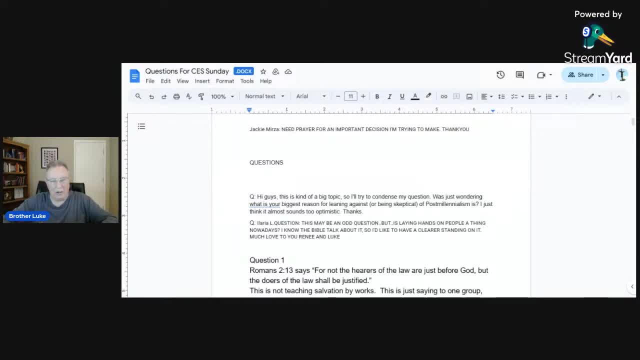 and he will no longer get high for his church as per the ket grams. would he go on? we know that, but we did that after a few. it was so difficult knowing what he, how he would have to suffer. the extent of it was so horrible that he sweated blood. that's how agonizing the thought of 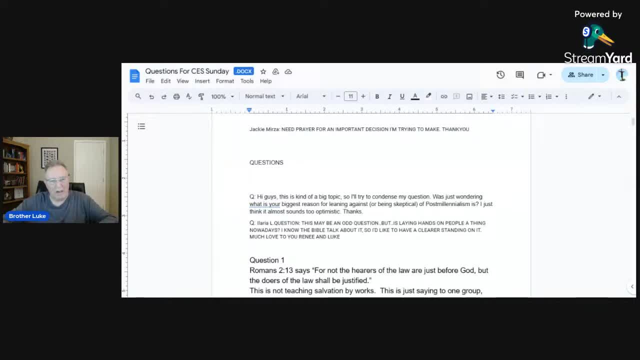 knowing what he was going to go through. and and he asked father God, if there's any way of taking this away from me so I don't have to go through this. can we do it, he says. and yet, not my will, but your will be done, you know, if you relate that 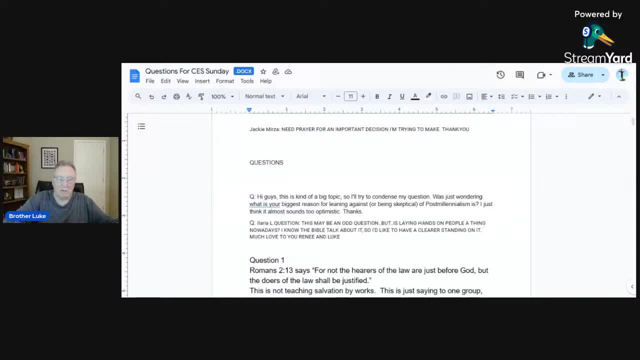 kind of scenario to the garden with Adam and Eve. Adam and Eve had a kind of a similar situation that they're in. they were asked to live according to God's will. don't eat from the tree of the knowledge of good and evil. God even told them- I don't know why nobody said this. I've never heard. 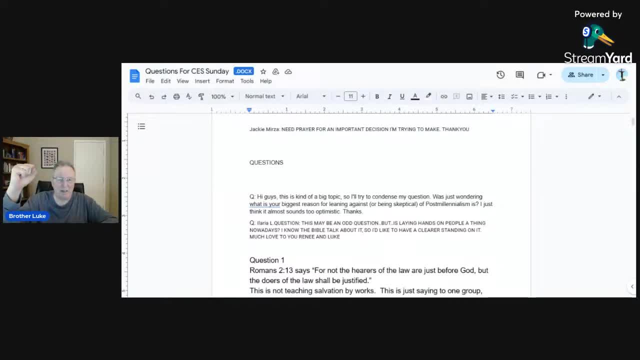 any theologians say this, but to see me, this is quite, quite obvious. if, if you had, if you have a child and you're in a forest or something, and you see that they're going to eat from us, eat from us of various trees and bushes- and you see them about to eat from a tree that is poisonous, you say: don't. 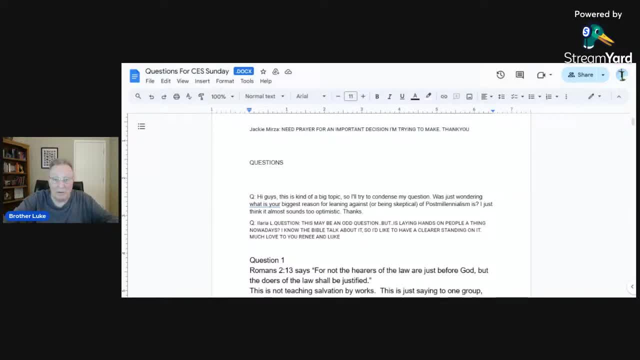 eat from that. it's poisonous, it'll kill you. well, that's really what the tree the knowledge of good and evil was. that tree was poisonous. it caused their death immediately. their spirit died. God withdrew his spirit. so now they're there: they have a living body, a living soul, but a dead spirit. 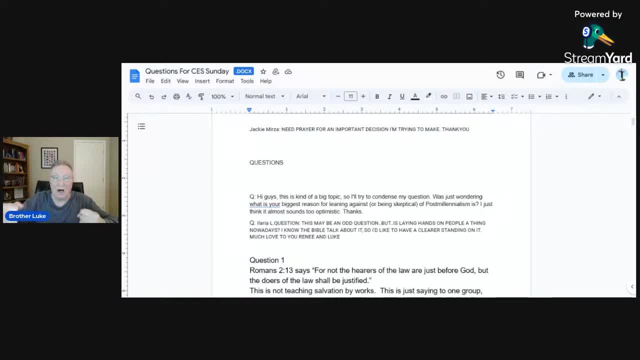 they're no longer a complete triune being in the image of God like they. that's why they. what has to happen for you and me and for everybody else now is we need to get the Spirit of God back. that's really what this is all about: regaining the spirit that was withdrawn in the garden with 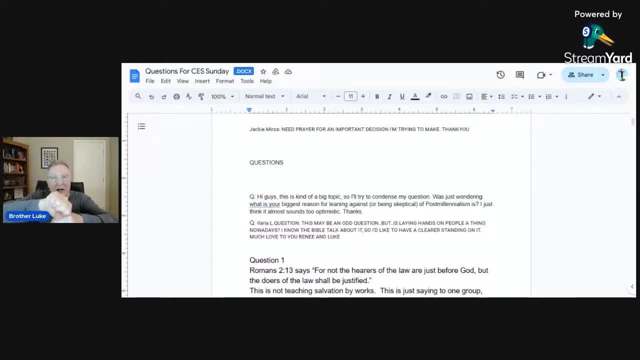 at the fall and we get the Spirit of God back. he not even with our spirit, but with God's spirit. that brings our spirit back to life when we have faith that Jesus is our Savior. but the point in making is it. I don't hear anybody comparing it to saying hey, don't eat from that tree is poisonous. 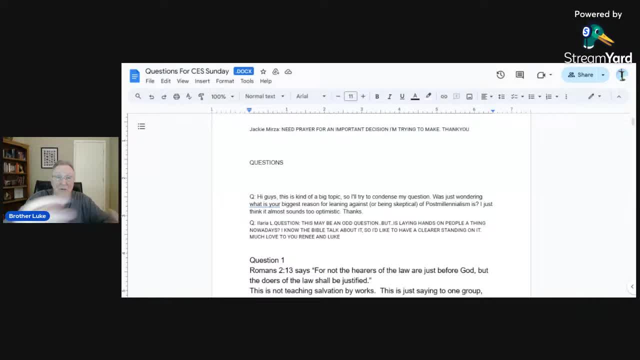 you know, the Bible says: don't eat from the tree. if you do, you'll die the very same day. it says they'll die in the very same day, by the way. and yet they live hundreds and hundreds of years. they, Adam, lived nine hundred years or roughly, I don't remember how long, Eve, I don't. 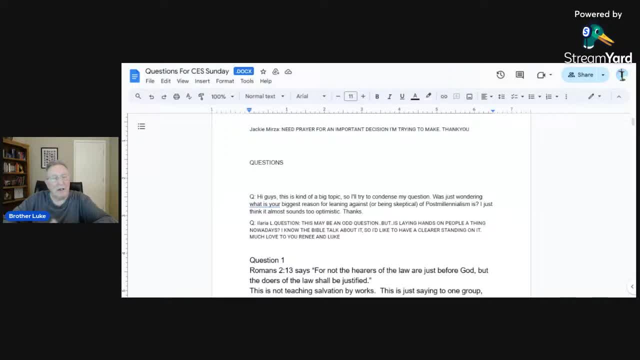 know if it says how long Eve, but they live, say, 8, 900 years. they didn't die the same day today, or did they? they died the spiritual death, the death of the spirit. so, and then the sentence of death was on them and all of us. so, because now, from the moment of the death of the, well, the 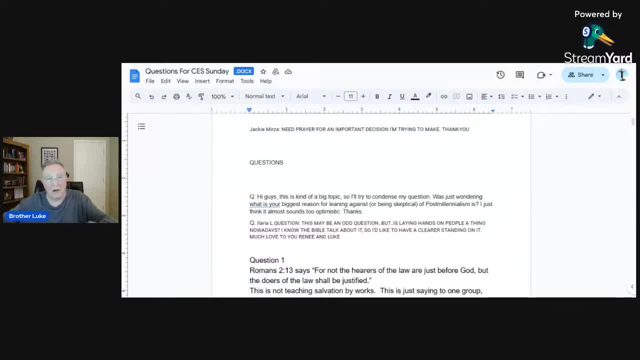 that point forward. we're all mortal with the sentence of death on us. but the point i wanted to make really is that their position, as they're standing in front of the tree of the knowledge of good and evil, is uh, is it god's will be done, or is it our will be done? 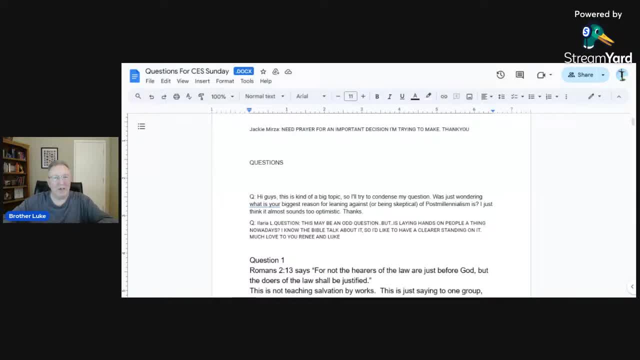 see they chose. no forget about god's will. god says: trust me, let me guide you, let me provide for you everything you need. look at the world: i provided you. look at the air i provide you to breathe. there's water, food. everything you need i've provided for you, and and life i've given you. 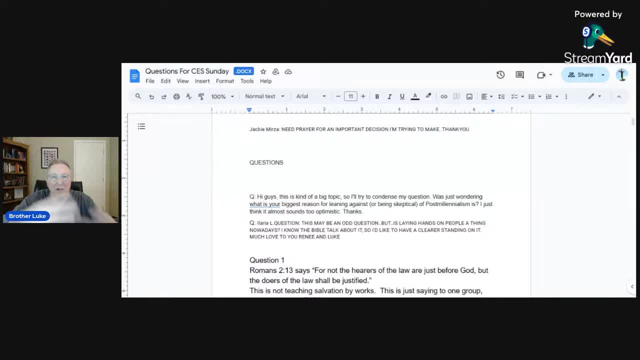 just keep trusting me to be your god and and let me be lord and in charge you and i'll guide you well and and you'll be blessed and happy and live forever. but uh, they were told by the adversary that god was a liar. if they ate from that tree, they would not die. 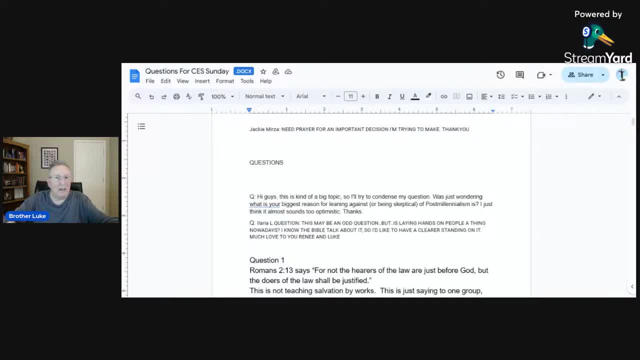 instead, they'll be like god, knowing good and evil, knowing right and wrong, and then they'll be in a position to make those decisions for themselves, so that their will could be done, not thy will be done. so they failed this test and said: no, my will be done. jesus passed this test in the garden of gethsemane. 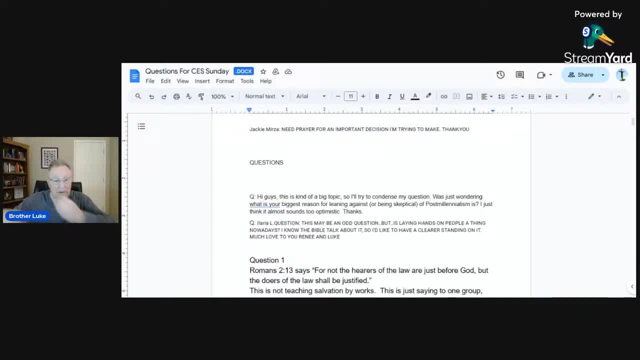 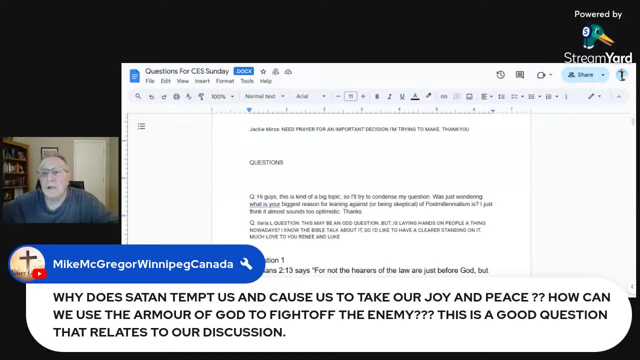 when he said: not my love, but your will be done. okay, let me see. ah, at least i'm kept quiet. zombie mark says: why does satan tempt us and cause us to take our joy and peace? one type of breath normally say someone is better than th? Loop. 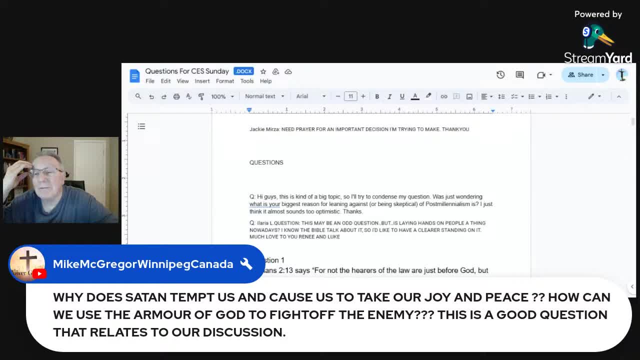 declaring yourself that you're. that's a good question, but i'm going to talk about it. why does satan tempt us? i, i don't think satan is tempting you, mike. i got it very much. there's over seven billion people in the world and satan, the being that you're referring to, uh- is one individual. 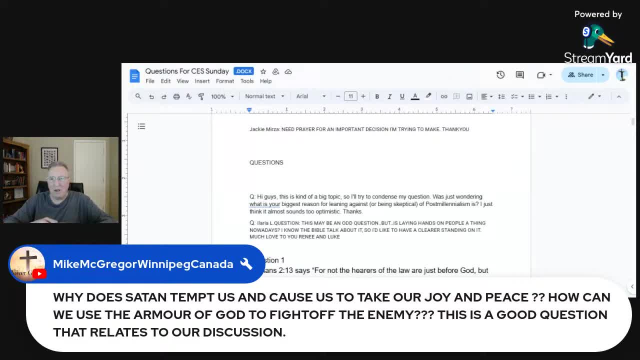 and he's not omnipresent. he's not everywhere at the same time. like god is, he can only be in one place at a time. why is he in canada, at your house? why are you so important to satan? the satan is tempting you the whole idea that when people think that satan himself is the one that's doing it to them. 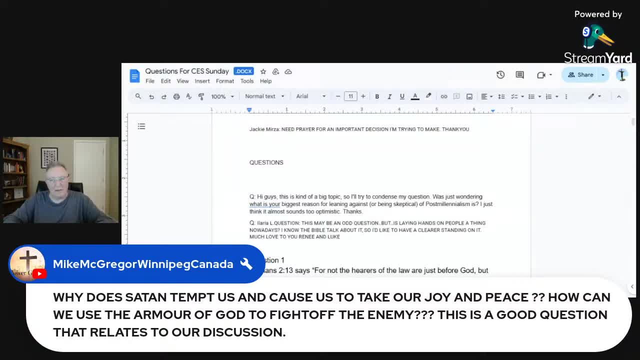 is quite absurd, isn't it he? he's not omnipresent, he's not omniscient, he's not. he's not god's equal, he's a created being. god could squash him like like an ant, anytime he wants to. so, uh, your problem with these temptations? don't blame it on satan. it's not satan, it's you. 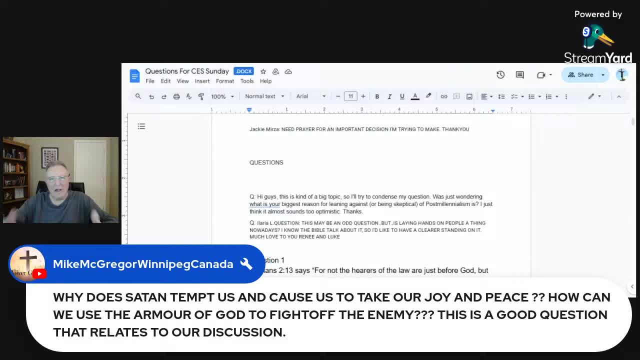 it's that natural. you're a natural born sinner, just like me, just like all of us. we're natural born sinners. no one taught you how to sin. you have a natural gift for it. of course, as individuals we have different proclivities for sins. 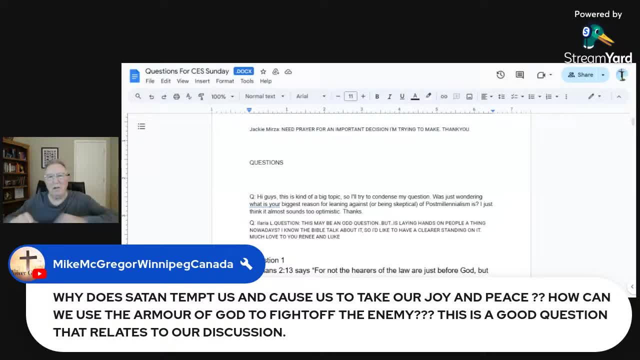 some sins appeal to me that wouldn't appeal to you and vice versa. but we all have these sinful desires and then, once you're born again, you have this conflict going on within you that paul talks about in romans, chapter 7: the struggle between the old man, the natural born sinner, and the new man, the child of god. 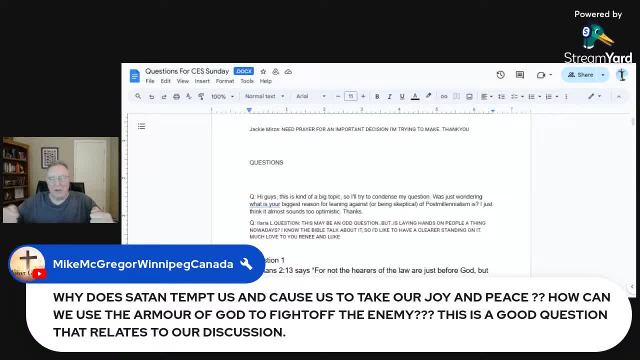 there's, the holy spirit is in charge here, and, uh, your flesh is in charge here, and the flesh wants to resist what the holy spirit is trying to get you to do. so there's a conflict going on, And the one that wins is the one you feed. 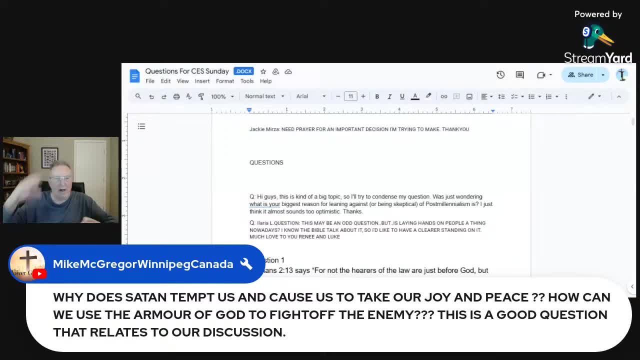 If you feed the flesh by thinking and doing fleshy things, you make those desires stronger. If you starve the flesh and feed the spirit with Bible studies, prayers, fellowship, ministry works- all these things are feeding the spirit And then the spirit gets stronger and dominates in your life. 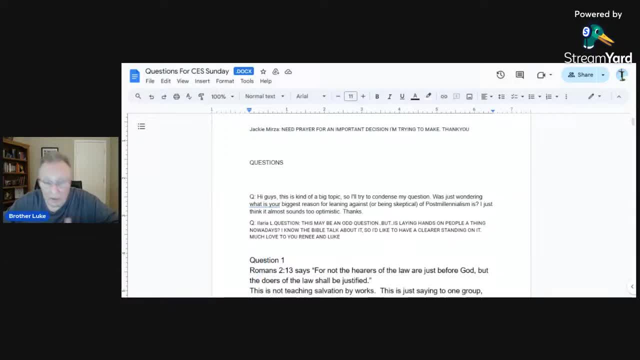 Okay, Mike, There is a. I mean, there are demons. there are demons trying to influence. Well, there is a spiritual war going on, but let's not think that any one of us is so important that Satan himself is dealing with you. 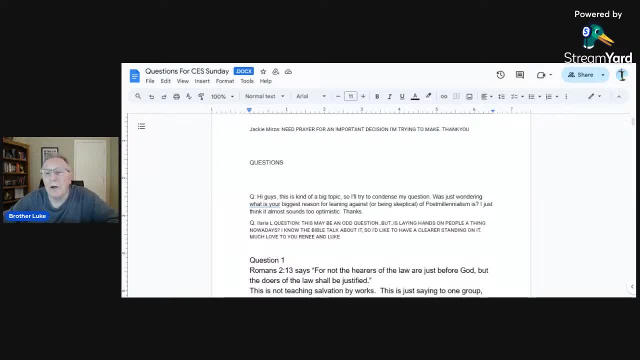 Screwtape Letters is an interesting book on that subject, about the spiritual warfare. Not that it's all correct, but it's interesting ideas You might look at. CS Lewis wrote Screwtape Letters. Okay, Okay, Mm-hmm. 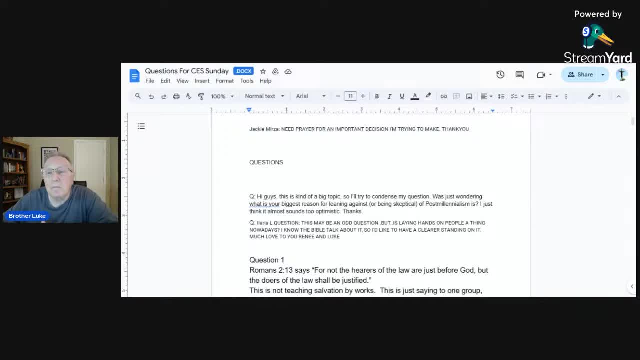 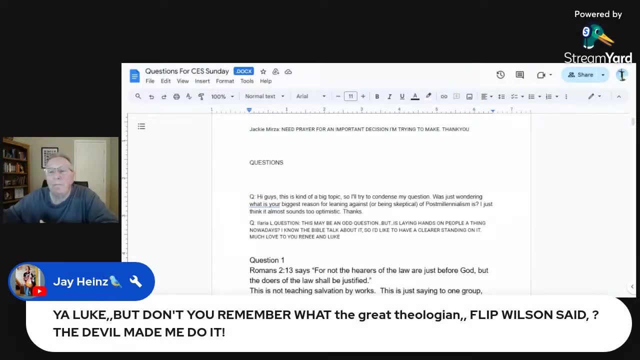 Mm-hmm, Mm-hmm, Yeah, Mm-hmm, Yeah. J says yeah, Luke, but don't you remember what the great theologian Flip Wilson said: The devil made me do it. I mean, yeah, the devil does, is involved, but the chances of you and I- he's involved with us directly is quite slim, I think. 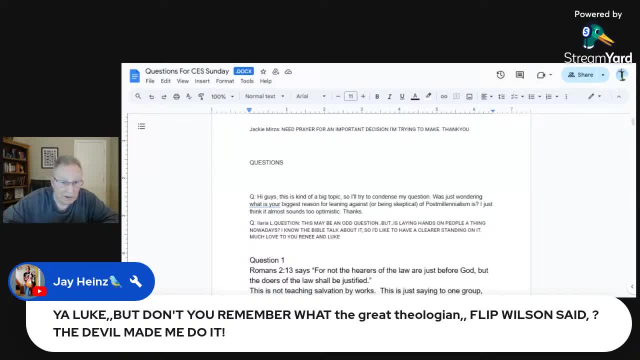 I think if you're really really an important person as far as affecting the world theologically, that he's probably going to be concentrating more trying to influence you the wrong way. but the rest of us, who are pretty insignificant in the big picture comparatively- 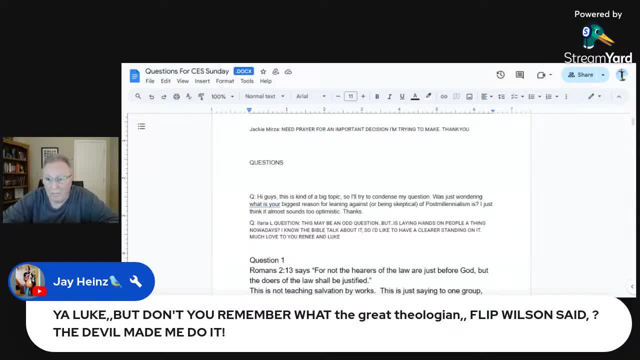 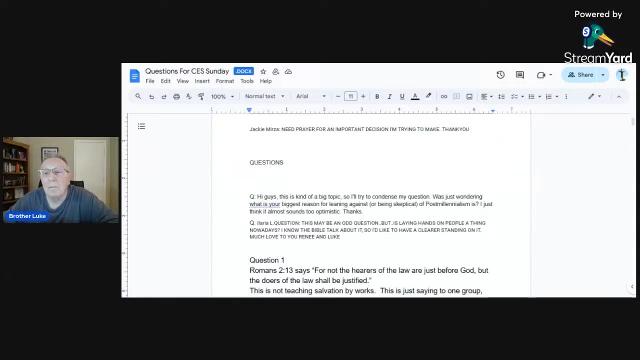 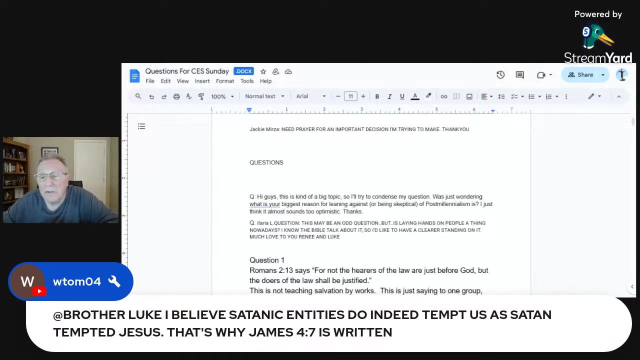 there would be maybe other demons if scroop tape letters has the plan, correct that they would be involved with us, not Satan himself. yeah, Tom says I believe satanic entities. yeah, satanic entities, but not the Satan. I mean, maybe the Satan did tempt you or me sometime. 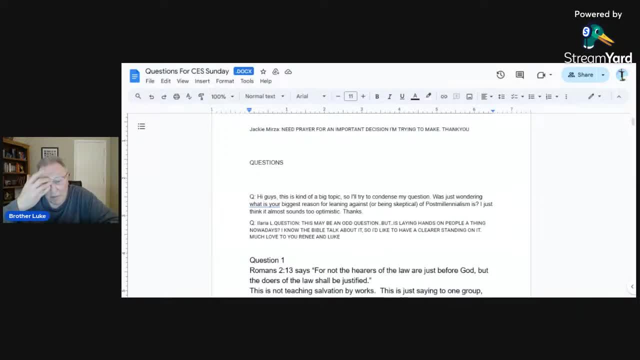 I doubt it, but, as I said, let's not give more power to the Satan than he actually has. that's one of the big problems in the world. much of the world thinks that there's two opposing forces, good and evil, God and the devil, and they're equal in power and strength. 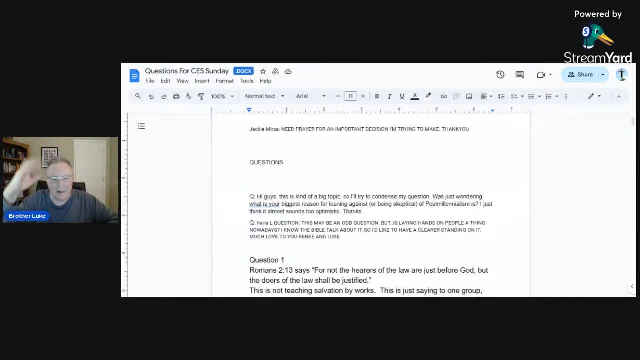 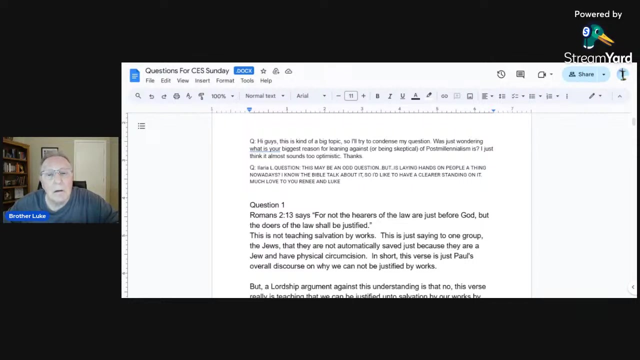 and there's struggle between them. but no, God is all powerful. Satan is nothing compared to God. as I say, he has none of the attributes of God. it's a mismatch completely. so let me look and see, let me see if there's another question here. okay, here's a question. 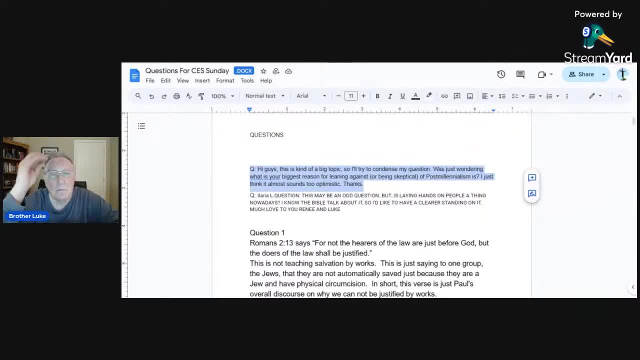 that was sent. hi guys, this is kind of a big topic so I'll try to condense. my question was just wondering what is your biggest reason for leaning against or being skeptical of post-millennialism? I just think it almost sounds too optimistic. thanks, okay. 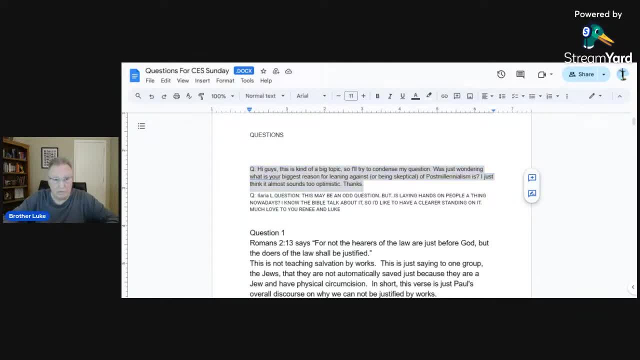 alright, I can't answer that question without telling everybody what the, the, the, the, the three millennial viewpoints are. you got pre-millennialism, which is the popular view in America today, but it has not been the popular view around the world throughout history. it's, it's um. but it's the idea that at some point Jesus will return and after his return he'll set up a millennial kingdom on earth for a thousand years. he'll set up a millennial kingdom on earth for a thousand years, which means he'll be returning prior to the millennial kingdom. and then the millennial will start. that's what I believed and Renee believed and many of you believe. but, um, Post-millennialism and all-millennialism are really both post-millennial in that, in that the idea is that Jesus returns after. 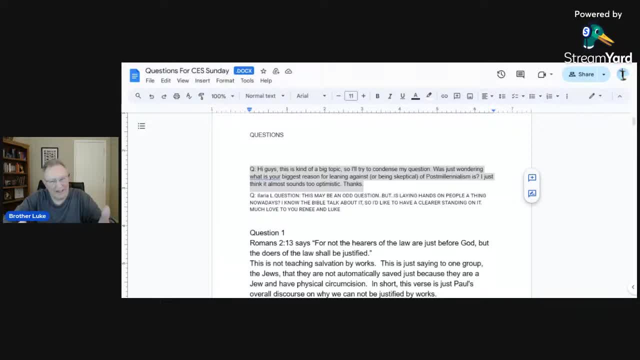 this millennial kingdom, which is millennial kingdom by allons. by the way, it's not in the bible. try finding. maybe you can find in a modern translation somewhere. but i look in the kjv and you won't find the phrase millennial kingdom. you want to find the? 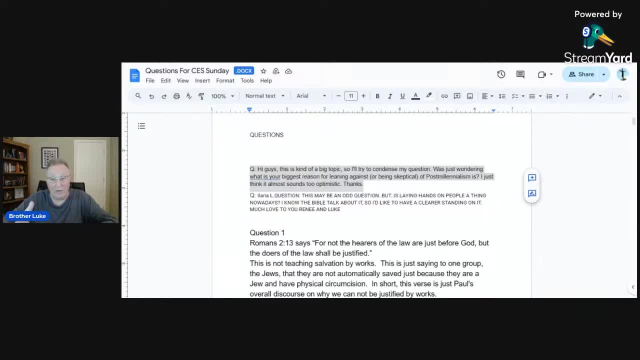 word millennium or millennial, you find the phrase 1000 years a couple of times and then they they translate that to mean it's a millennial, it's a thousand year period, when it should be understood as a just a long period of time. and jesus said: and it should be. 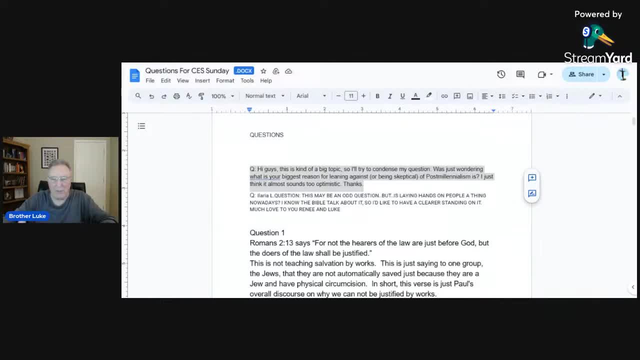 understood as the kingdom- the kingdom of god or the kingdom of heaven- that jesus talks in the accounts, talks about. so this kingdom of god and the kingdom of heaven is the same thing, and jesus says that it's here now. he brought the kingdom with him, he started the kingdom. he. 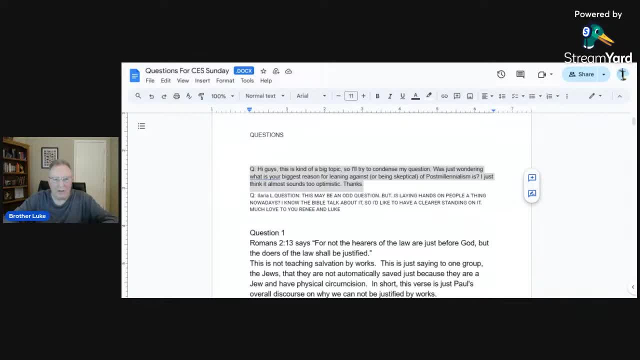 he is the kingdom and you and i are the kingdom. you're all. the kingdom is within you, jesus's kingdom is within you. the kingdom is among you. in other words, i'm representing the kingdom, i'm establishing it. now. i'm the king. so he established. 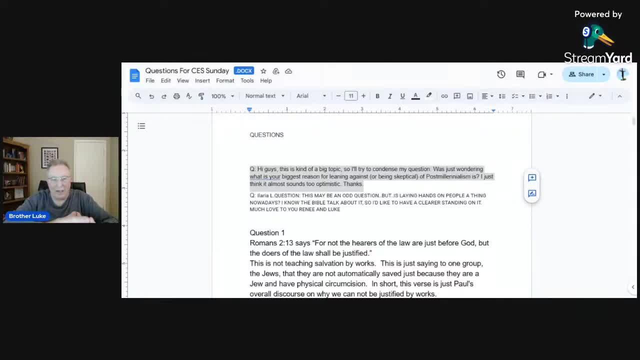 the kingdom when he first came, and the kingdom has been going on until- uh, okay, he's, he, he's died, he was buried, he was raised from the dead, he was. then he ascended 40 days later and we're waiting for him to return again, and when he returns again, that millennial kingdom will end in that sense and we'll start off with. 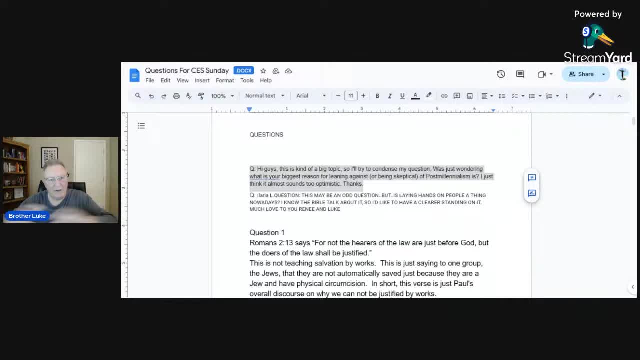 the eternal kingdom at that point when he returns again, the eternal kingdom where heaven and earth are united together forever. uh so, but the point is, but the difference between post-millennialism and all millennialism is not when the kingdom is we. we agree that it's before. 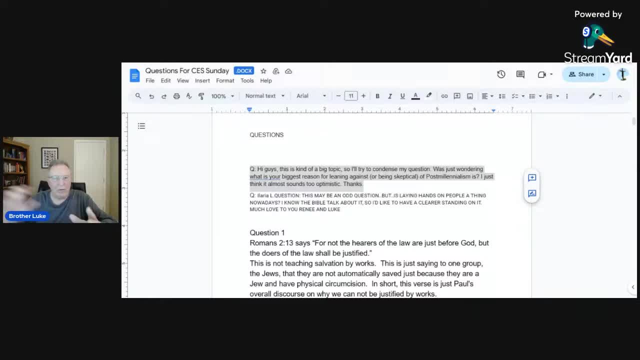 jesus's final coming. but the post-millennial view primarily is an optimistic view. it's the viewpoint that the world is going to become more and more christianized until almost everybody in the world is a believer and then jesus returns. so it's called an optimistic. 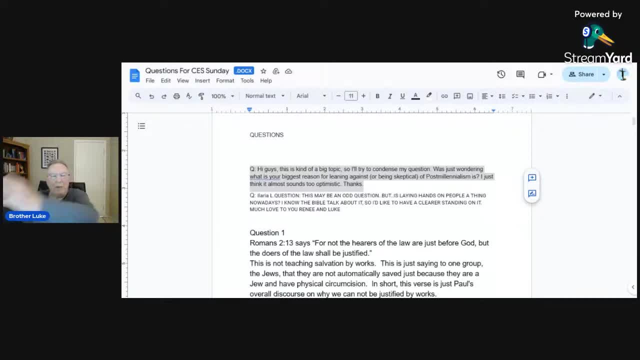 viewpoint that the world is going to get better and better and better because of christianity being spread around the world, and then the, the all-millennial view. normally, as i see it too, is a more of a pessimistic view, where we think that the world- no, it's not going to get better and better before he returns. 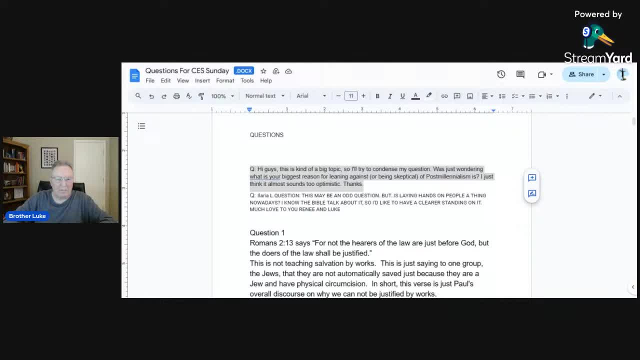 if anything is going to get worse and worse, um and that christianity, uh, during this kingdom, it's never going to reach the point where it's. the majority of people, most people in the world, are christians. jesus said that narrows the way, widers the road. many go one way. only a few go the right way, so that means only. 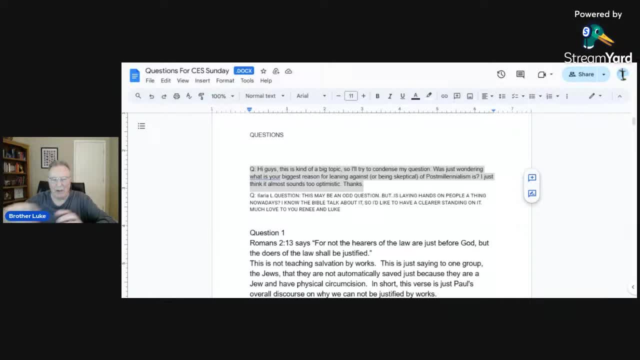 a few throughout all of history, only a few. the bible refers to this as a remnant. a remnant is a little tiny piece of the whole, only a few throughout all history. um will our children of god, and so, uh that, if that viewpoint is correct, i i believe what jesus said it. so, therefore, how could the world 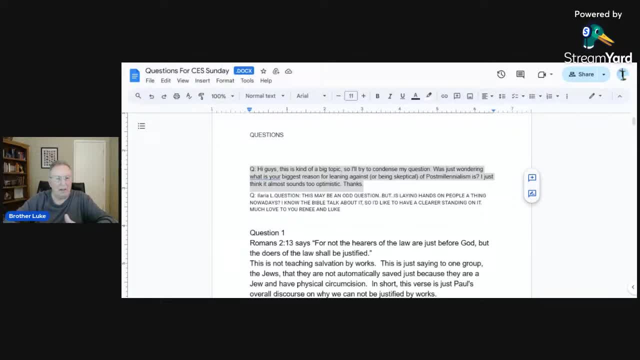 become almost entirely christianized? uh, if only a few. so i believe that, even though the total number of christians will grow and grow and grow, the percentage of people who are christians probably remains pretty constant, and we've done the math before. i think it's roughly about three percent. 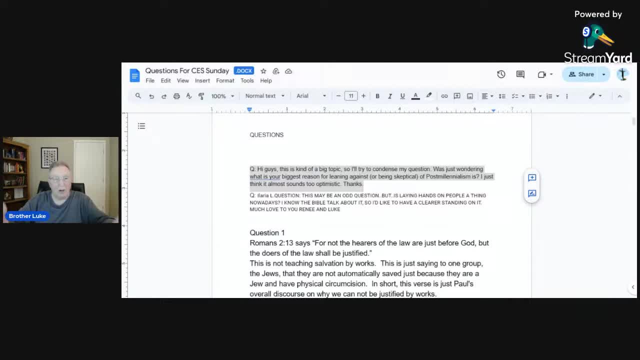 of the whole population. i believe, understandably, christ, christianity, the way that we do that. it's grace alone, faith alone, christ alone. we don't earn our salvation. it's a gift from jesus. so, uh, how many people in the world understand and believe in that way? a very small fraction of people. so that's the question about. 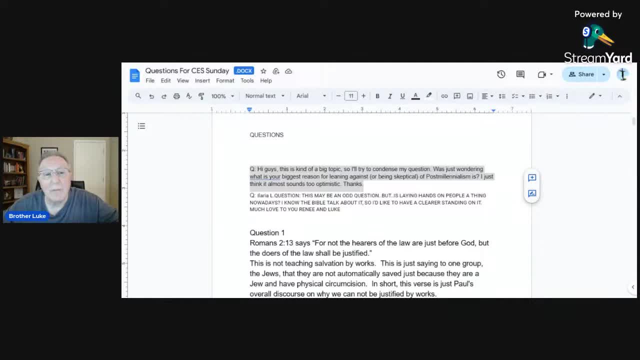 post-millennialism. uh, that is the. the main distinction is the optimistic viewpoint compared to the optimistic viewpoint of christianity compared to the, i think, the realistic or pessimistic viewpoint that the world's not going to get better and better because of the spread of christianity. okay, let me see if anybody 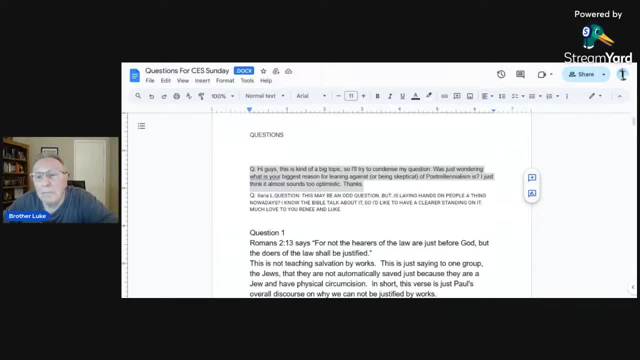 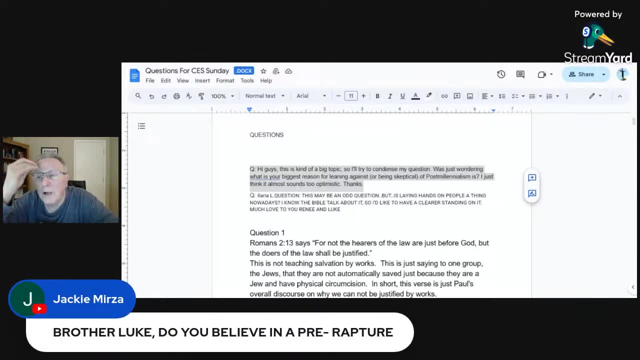 let me see. jackie mercer says: do you believe in a pre-rapture? no, i used to. i used to believe- as most people do today, by the way- um- the idea of a pre-tribulation rapture and then a tribulation period, and then a coming of jesus, and then a millennial kingdom for a thousand years, so on. 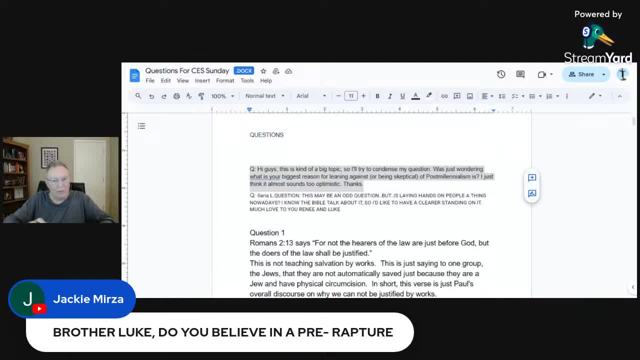 that scenario is pretty new. it really was developed in the 19th century, in the middle of the 19th century, in the middle of the 1800s. um, i mean, there are a couple of tiny elements of it you can find in the early church, but as far as the details, the way you understand it today, 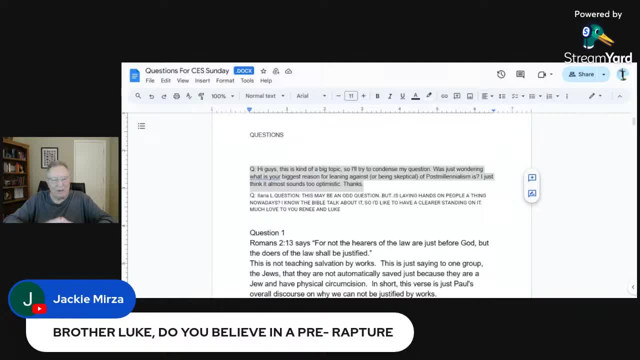 uh, that's, that's pretty brand new. so you'd have to think all the theologians of church history somehow were blind to this until john nelson darby figured it all out and put it in the form of charts and graphs and timelines, and all that with 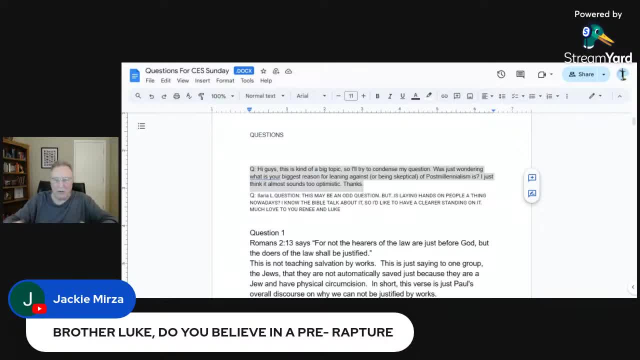 clarence larkin and peter ruckman and all those people who contributed to it, so that, so that that viewpoint is the popular viewpoint in america today, but it's not the popular viewpoint around the world. it never has been. okay, uh, so the pre-tribulation rapture is the position i used to hold. renee used to hold it. 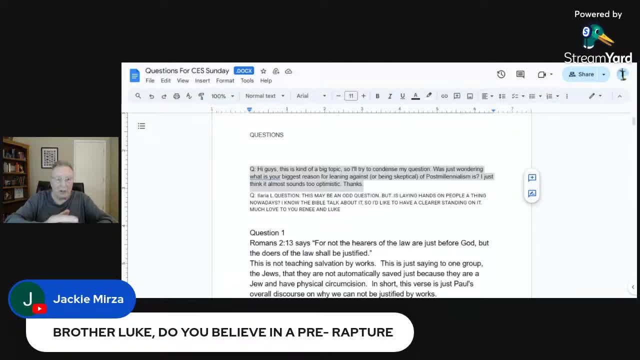 but now we understand that the, the rapture, that's when jesus has all of the people who are alive, who are believers, when he returns, get somehow changed in midair and and we get, uh, glorified bodies and we don't have to die and we get to live on eternity without 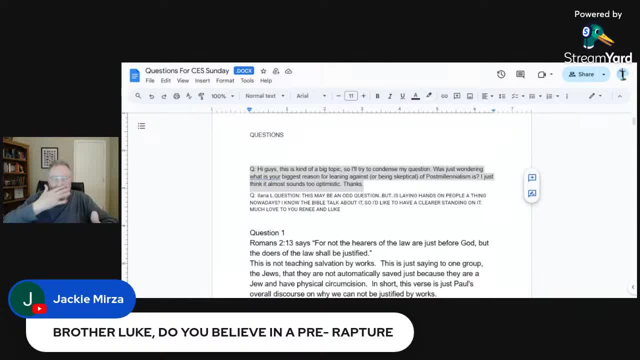 having to go through death. that's what you could call it the rapture, but it's really the same thing. it happens at the same time as the general resurrection. the general resurrection: if you study- do a word study on the phrase the last day, you'll find out. on the last day certain things happen. 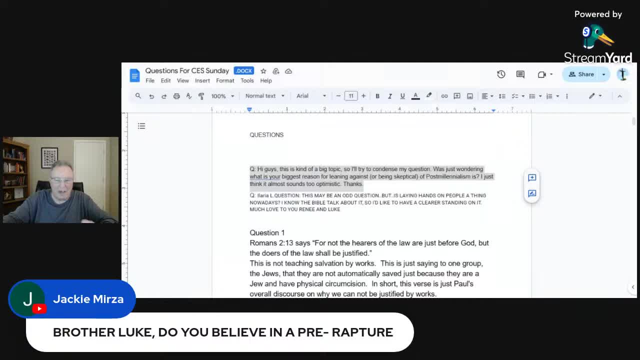 a lot of things happen on that last day, and one thing that happens is the universal general resurrection, the resurrection of all mankind. every person who has ever lived is raised from the dead. on the general resurrection the bible says: the resurrection of the just and the unjust, the saved and the lost. all people are raised. 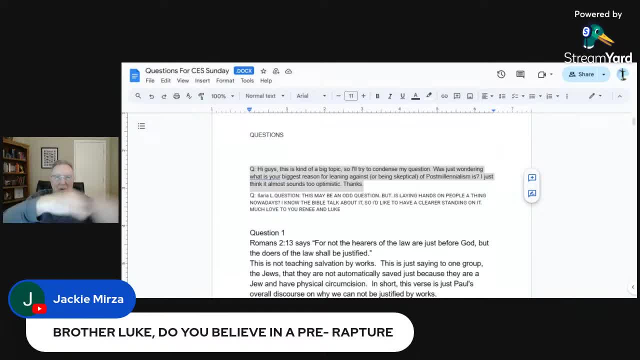 and the, the unjustified, the people who are lost, they get raised to go to their judgment. and and the believers who are dead, and they get raised alive to go be, to be, to be with christ, and, uh, the people who are alive, at that time they don't have to get raised because they didn't die. 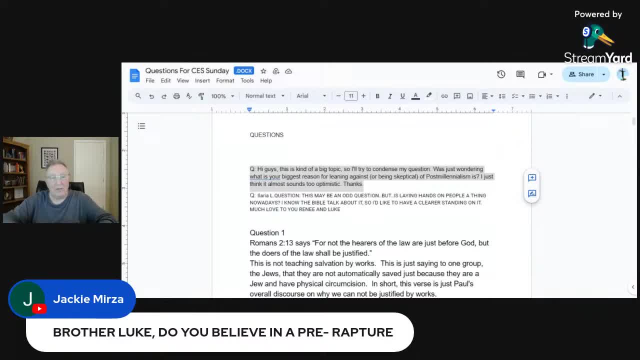 they're alive, so they just get glorified. but the glorification of the living believers, uh is? we call it the rapture, but that happens at simultaneously, at the same time as all everybody's raised from the dead. that's the way the church has historically understood this, and i know i think it is jackie. 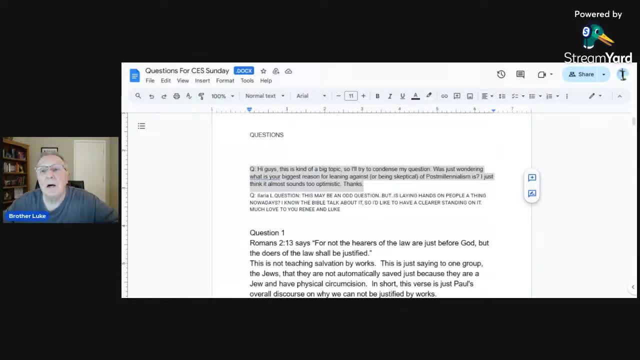 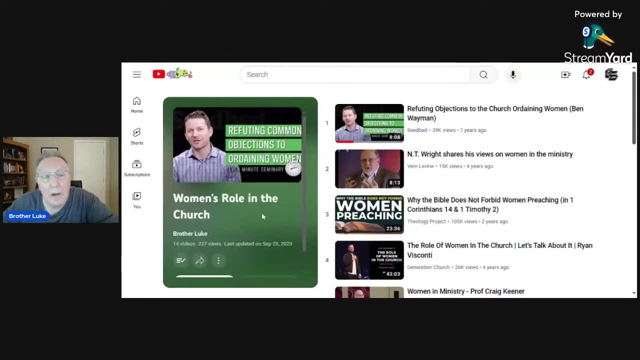 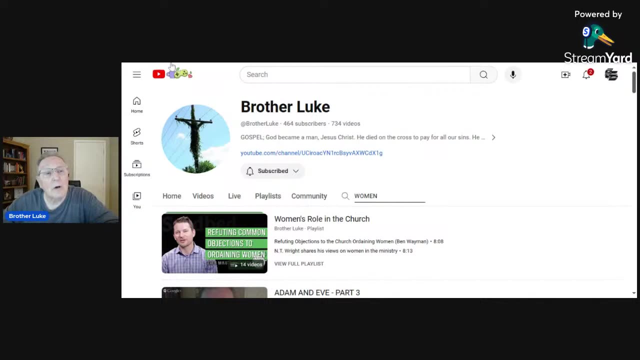 laughs: uh again. you could go to um, uh, uh, excuse me, let's look at uh. yeah, let's look at uh uh. here, let me go back one more, one, one more, yeah, one more i'm gonna. why can't i get? i'll just go to the church channel here. 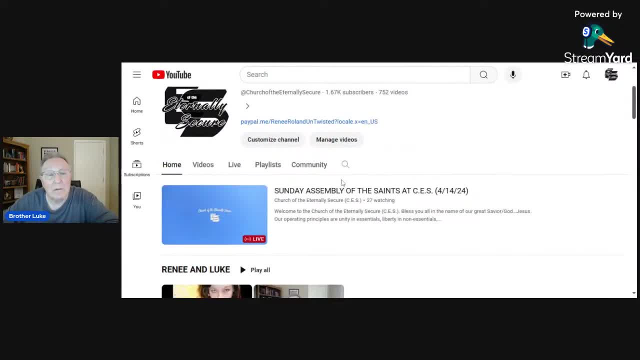 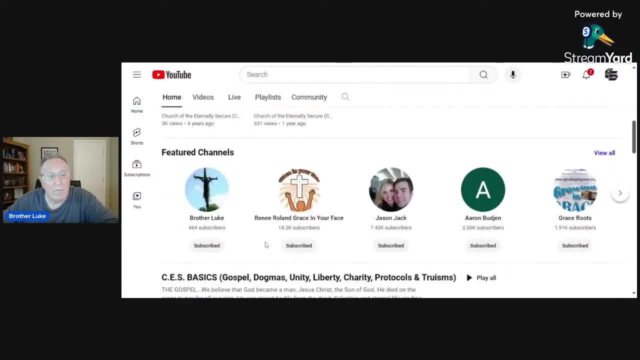 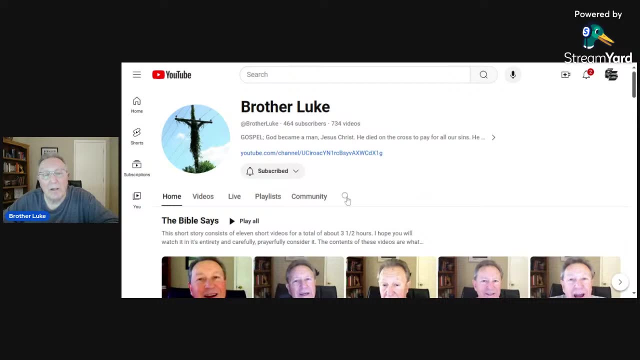 Okay, Here's the CES channel. I'm just going through these extra steps so you know how to get here. So you go to CES, you scroll down and find Featured Channels. Brother Luke, Click on that. Now you can just type in here Eschatology or End Times and find it, But you can also just 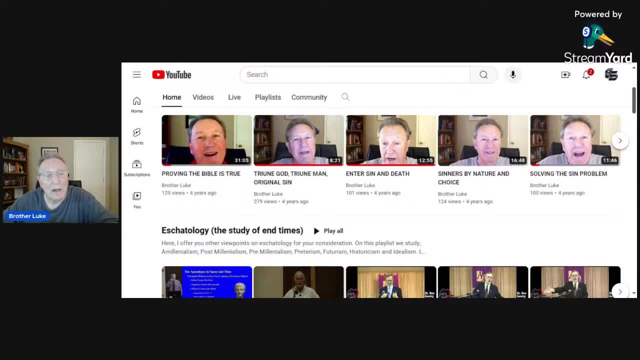 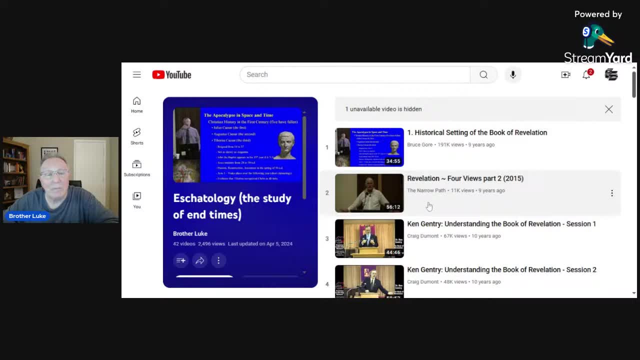 scroll right here. It's the second playlist. here Featured Eschatology, the Study of End Times. If you click on that, I had like 150 videos on this. I narrowed it down to 42. So I've streamlined it. But everything about End Times in terms of the four different ways to understand the Book of 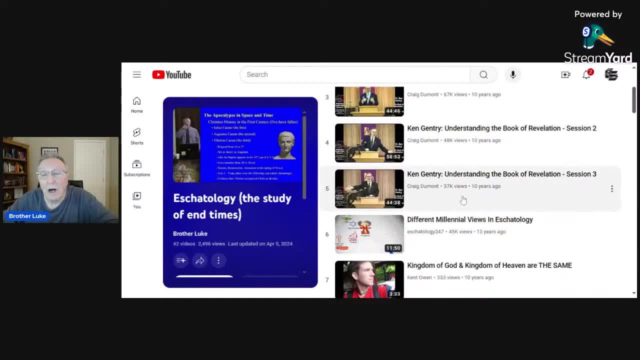 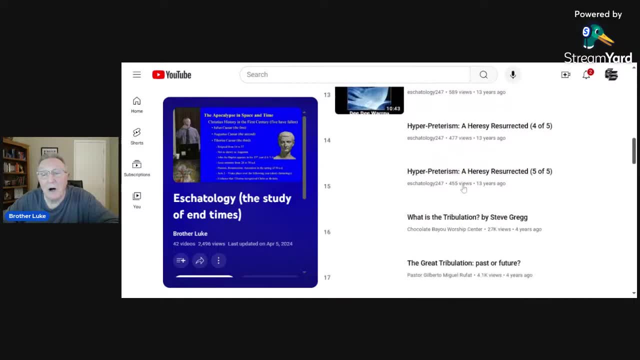 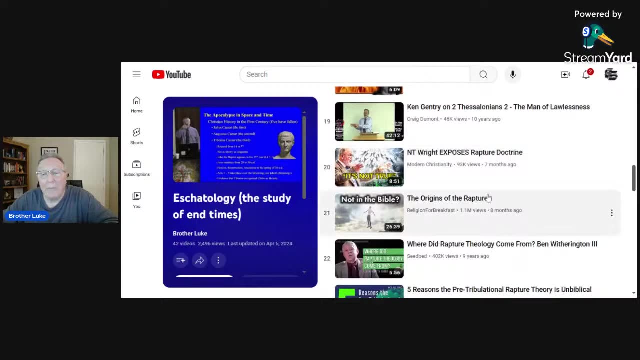 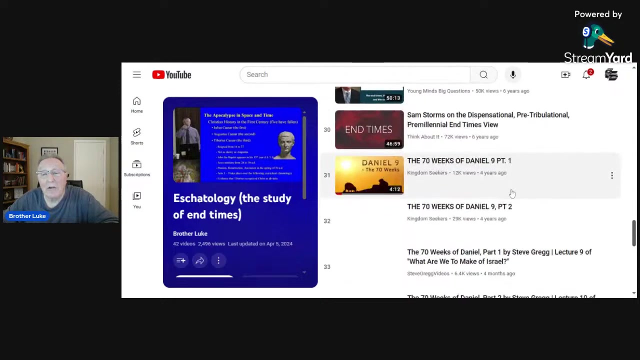 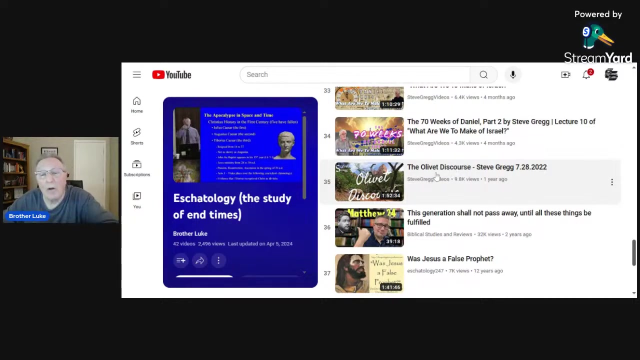 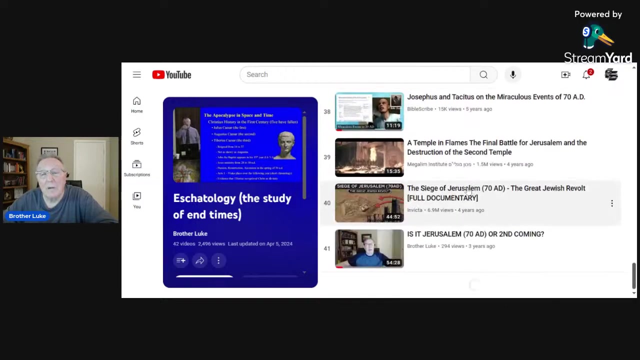 Revelation: four different viewpoints looking at it. what are millennialism views? what are the different views on the tribulation, the rapture, dispensationalism, Daniel's 70th week, the Matthew 24, the Olivet Discourse, when Jesus predicted the destruction of the temple. All these things are on this. 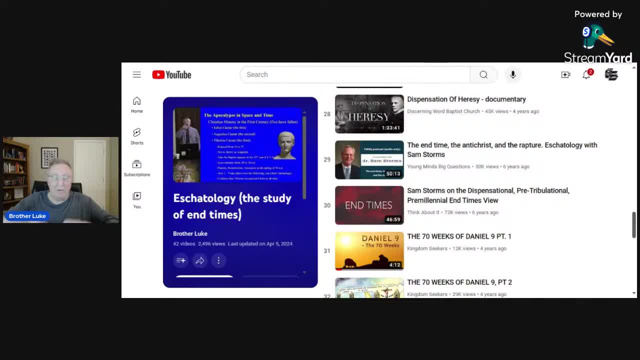 playlist So that you know on Sunday we're going to be talking about. you know we're going to be talking about the rapture. So on Sunday, when you ask me a question about the rapture and I give you a. 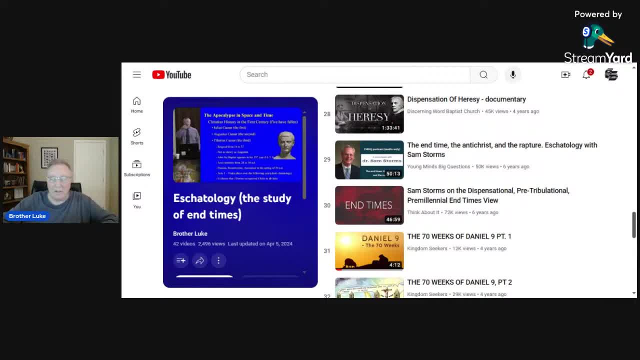 five-minute answer. you can go to that playlist and dig in for hours getting all the details and see the reasons that I've come to the conclusion that I have. Okay. Okay, All right, Let me see. Maybe I can answer one more question here. 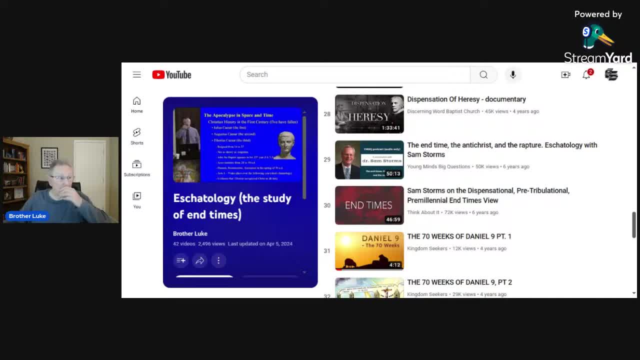 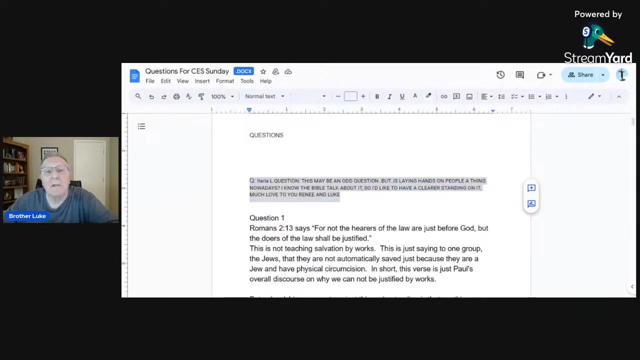 Okay, This one is from Ilaria. Let me try one more spray. I think this will be the end. I think I'm going to finish up with this. Excuse me. Oh, I need to put that on the screen. Here you go. All right, This is another question that was. 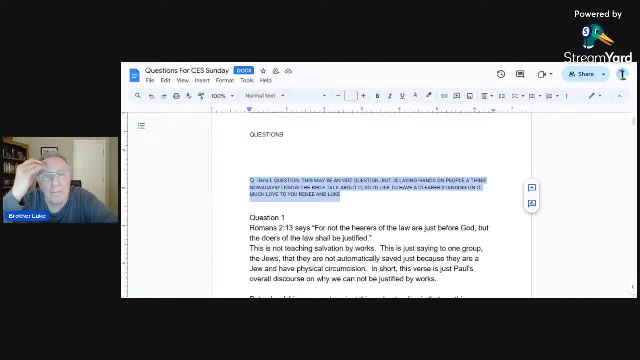 posted. It says Ilaria wrote: this may be an odd question, but is laying hands on people a thing nowadays? I know the Bible talks about it, So I'd like to have a clear standing on it. Much love to you, Renee. 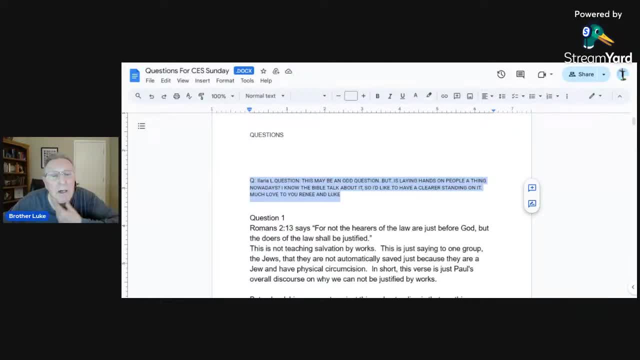 Renee and Luke To you, Renee and Luke. Okay, So the laying on of hands. what do we have to say about that? I don't see anything. I'm not. nothing comes to mind about the laying on of hands no longer being. 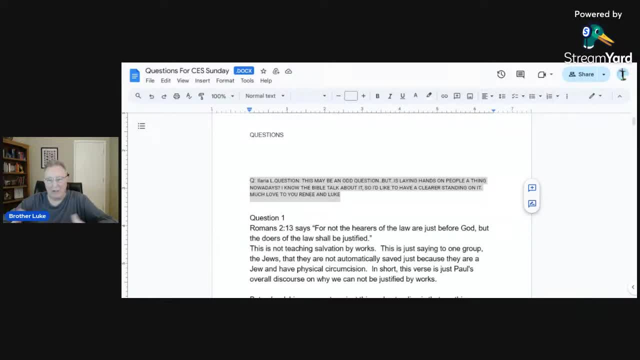 a practice, I don't see any reason why it would not continue to be practiced. You can pray for people and lay on hands, and you can many times. laying on hands is a way of ordaining people and sanctioning them to go on into a particular ministry and blessing their ministry. You can lay hands on them as you pray for healings or prayer needs. 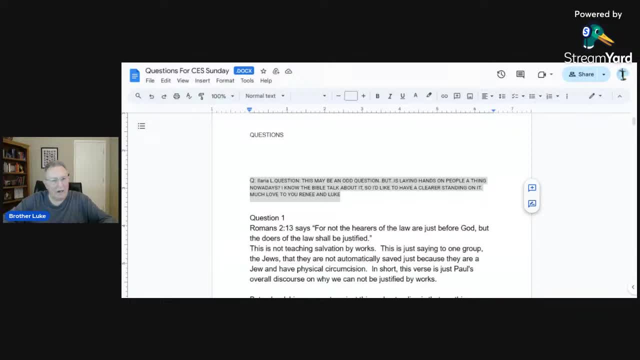 Laying on your hands, even anointing with oil. I don't see anything in the Bible that tells us stop doing that. Now, how important it is or not, I don't know, I don't. I don't know if it's necessary. I don't believe it would be necessary. Would it be helpful if I had a choice of praying for someone by laying my hands on them or praying them without laying my hands on them? Is there a difference? I don't know. I think you're free to do it either way. 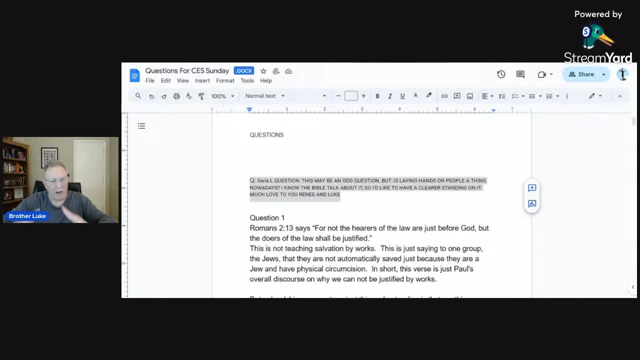 Okay, I think it's probably a beautiful thing as an expression, if nothing else, to lay your hands on someone so that they know that you're committing something to them. You're asking the Lord, You are saying it's intercessory prayer, praying for the needs of somebody else, and you're putting your hands on them to give them that blessing. 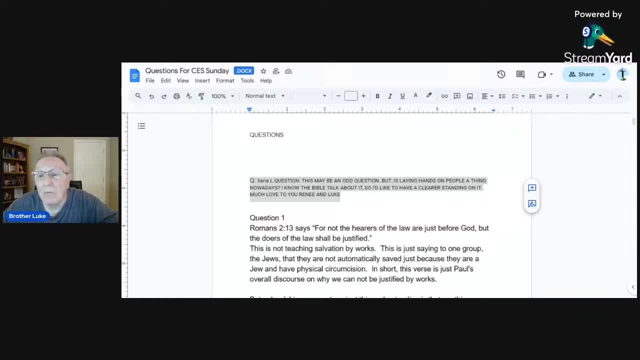 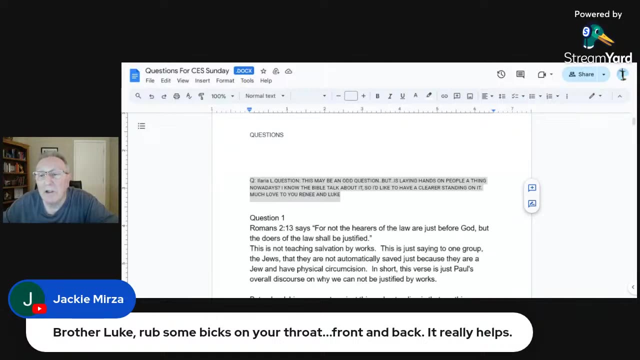 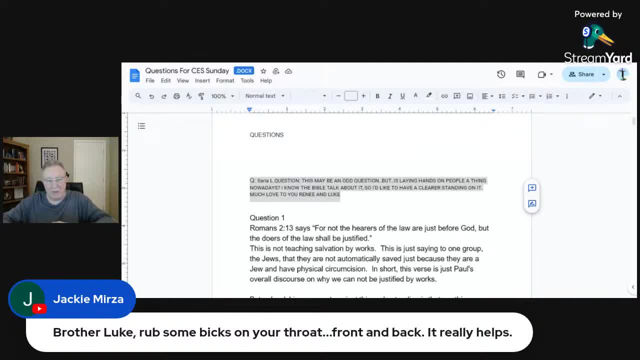 But I remember the very first time, when he was a newborn baby, the very first time I got to watch him by myself. My wife and my sister went off to do something, And when they came home they said: what's that smell? 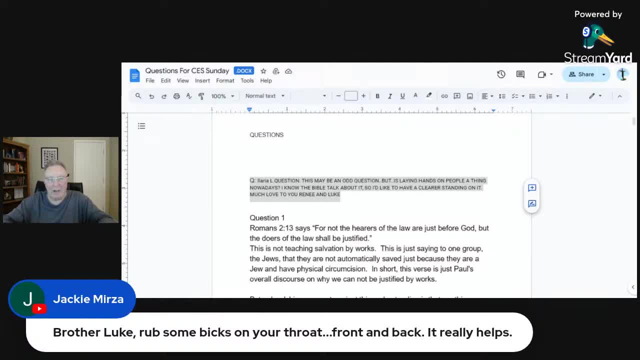 My boy, my little boy was crying and there's this smell in the air. What's that smell? I said, well, I just, I just changed his diaper. I was so proud of myself, I changed his diaper. I said: you know how you rub this stuff on them like a lotion, or it's supposed to be like Vaseline. You put Vaseline on them and then and then you put the diaper on them. That's what I did. That's not Vaseline, That's Vicks Vaporub. So could you imagine your baby and you wet and you got a little rash from being wet. 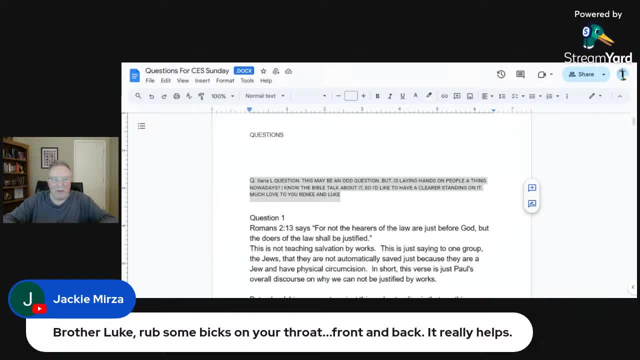 And now they? now they put Vicks Vaporub on it instead of Vaseline. I mean, It must have really burned a bit horrible. But that was my very first attempt and failure at changing my boy's diaper. But I don't know about Vicks on my throat. 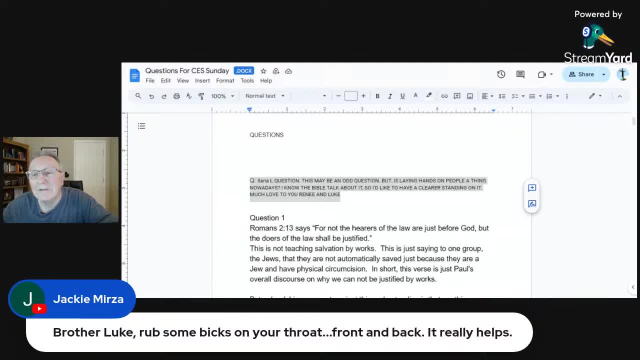 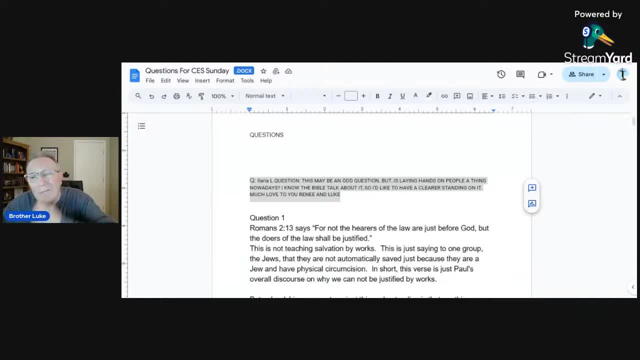 I'm not sure I could go for that. I don't know. Have you done it yourself? Have you done it yourself? Okay, All right, I think it's time. It's time I lasted longer than I thought. I thought. maybe I can last an hour.